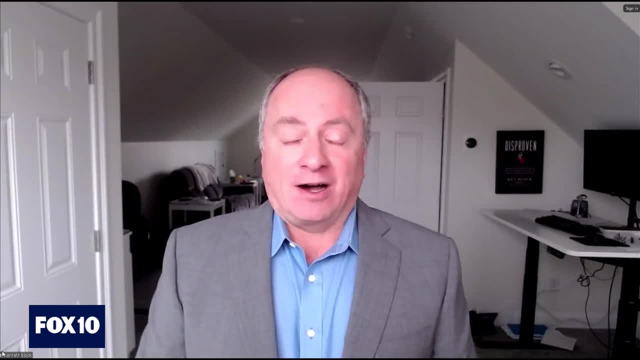 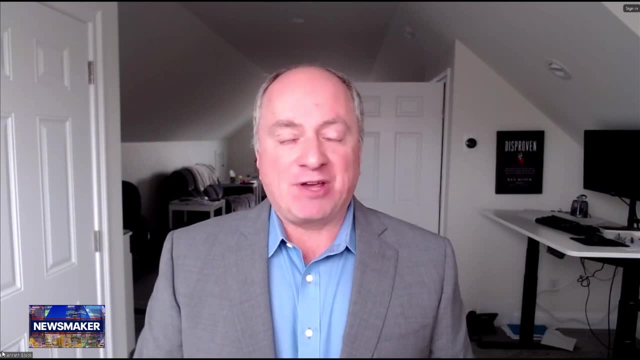 in the swing states And that was a shocking phone call. I told him I couldn't answer straight away and I needed the night to think about it. I did. I spoke to my family about it, thought about it a lot more, talked to some trusted advisors And when I called Alex back, 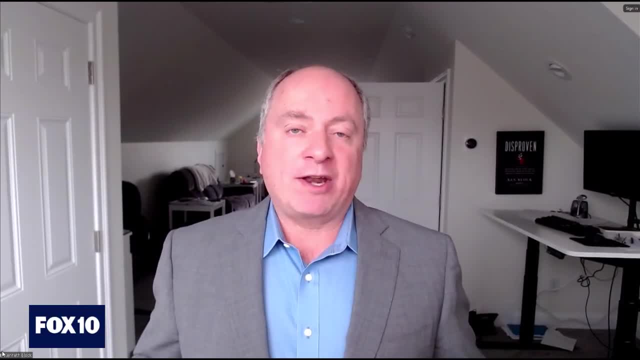 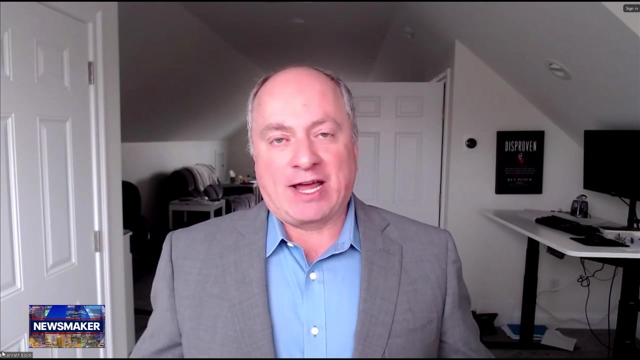 the next day I told him I would do it, but I wanted him to understand what the framework was that I was willing to work under, And that framework was really important to me. I wasn't going to custom deliver a series of findings that the campaign dictated me. What I told Alex was: if there's voter fraud, I'm going. 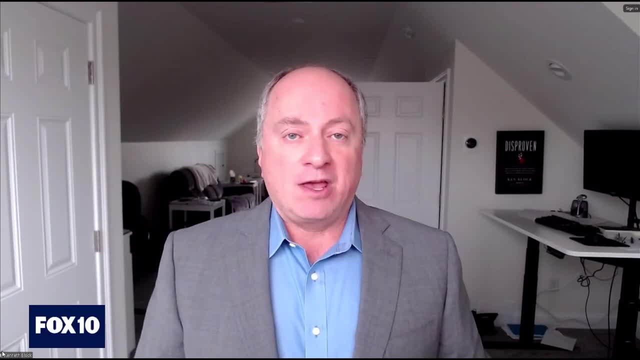 to find it and I will leave no stone unturned looking for it, And what I find I will successfully defend in court. That's actually a clause in our contract. But I also wanted him to make sure that not just Alex but everybody above Alex understood that the work that I was doing was not a promise. 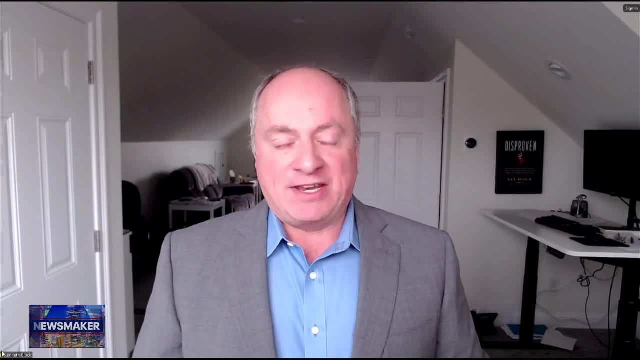 that I would deliver findings of voter fraud. I didn't want anybody to have the misconception that I was signing the contract and I was going to deliver the smoking gun that everybody needed. I wanted them to understand that I didn't think it would be there, but I would leave no stone. 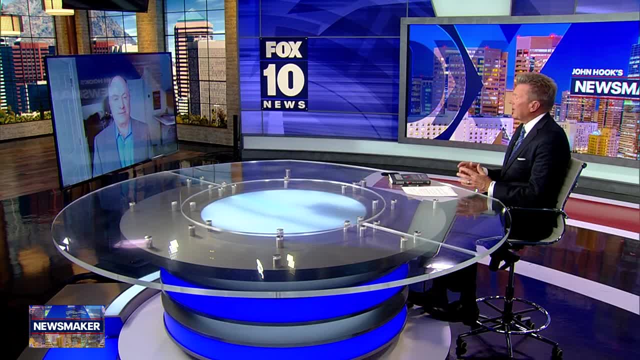 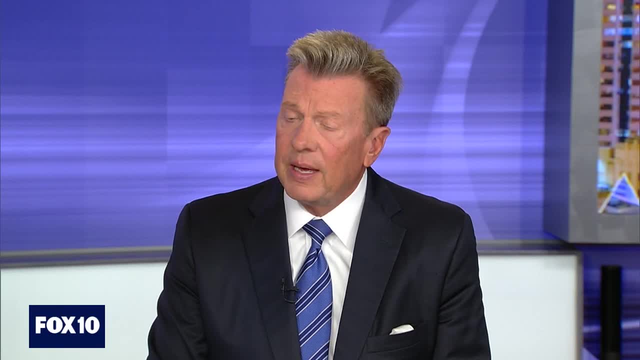 unturned, trying to find it. That's an important caveat. You told them up front that in years of doing this, this kind of work, you had never seen any kind of fraud On the scale that they needed quote unquote- to change the election result. And you told them that. 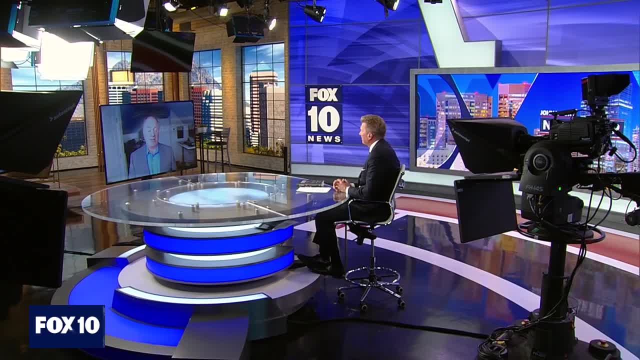 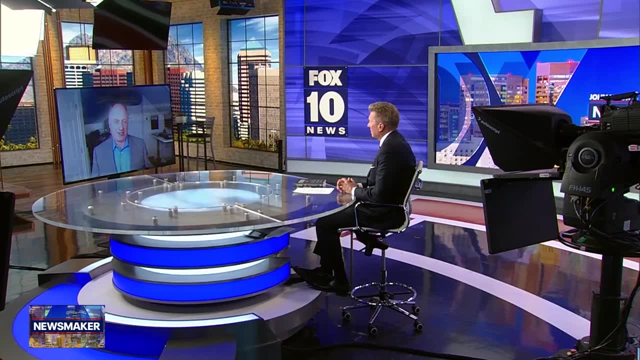 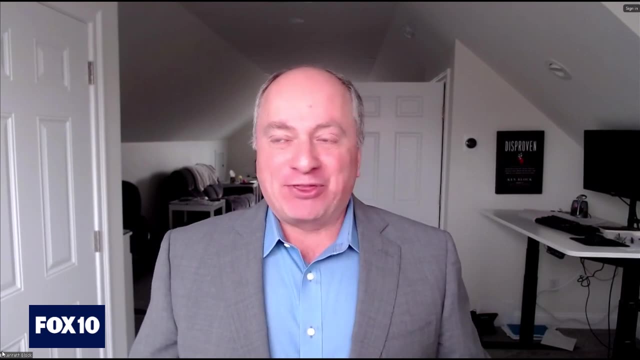 up front. Yes, I told them right up front because the way I do business, and especially with something as contentious and fraught and with such high stakes attached to everything that was about to happen, I didn't want anybody to have a misconception about what the potential realities. 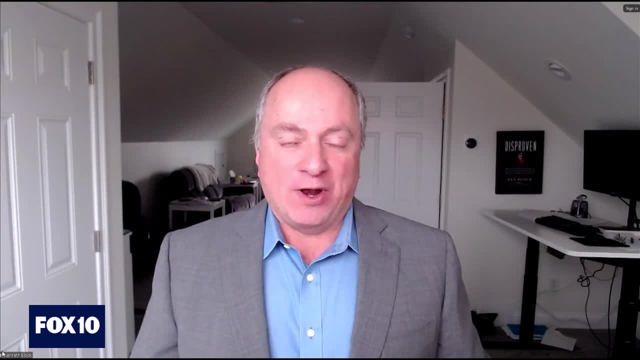 were going to be. I didn't want my customer to not be able to do what I wanted them to do, Not be put on notice that I might not be able to deliver what they wanted, And the response that came back from Alex. two responses came back. The first one was: we really want a straight up. 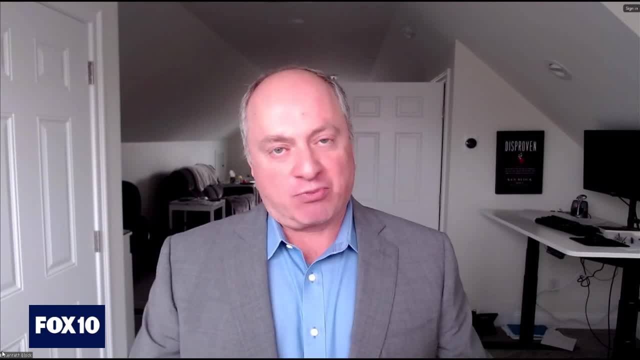 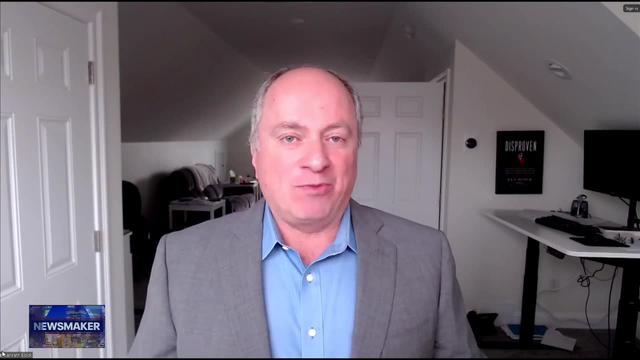 assessment. I appreciate your honesty and I appreciate the approach you're going to take to this. And then what he then did, which was even more important in retrospect, was he then told me that he was going to keep my company's identity and my identity a close secret? 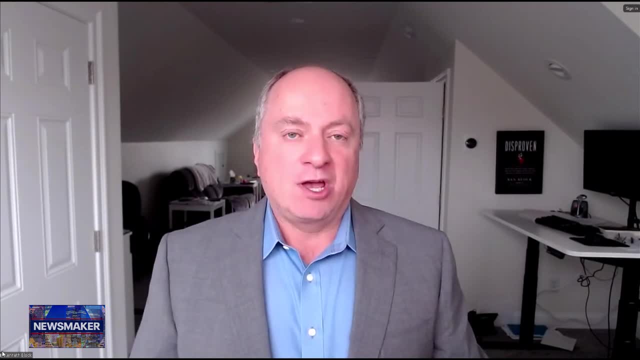 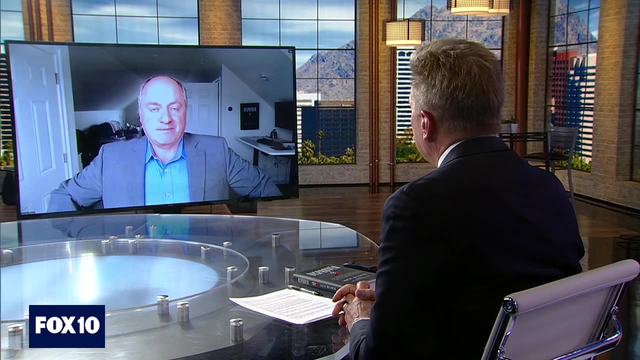 So that I wasn't put under undue political pressure to deliver specific results. If the folks didn't know how to reach me, they couldn't put pressure on me. Did anybody ever give you pressure, Ken? find it? No, No, never. It's remarkable. You were looking into the five swing states- Pennsylvania, Michigan, Wisconsin, Arizona, Nevada- And the two things you were primarily looking for were duplicate votes, people who voted twice and dead people voting Correct. What did you find? So we found handfuls, small handfuls, of deceased voters across the swing states. 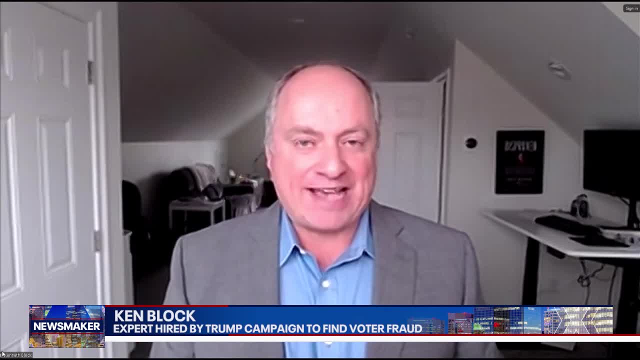 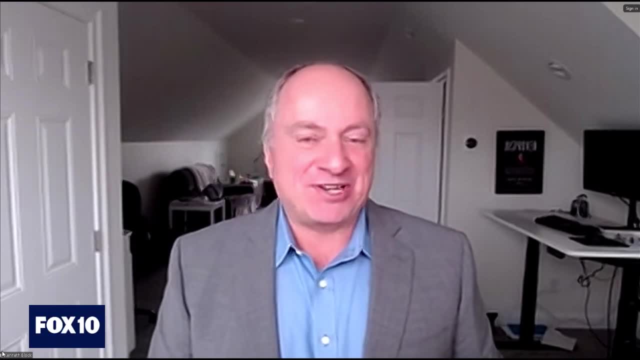 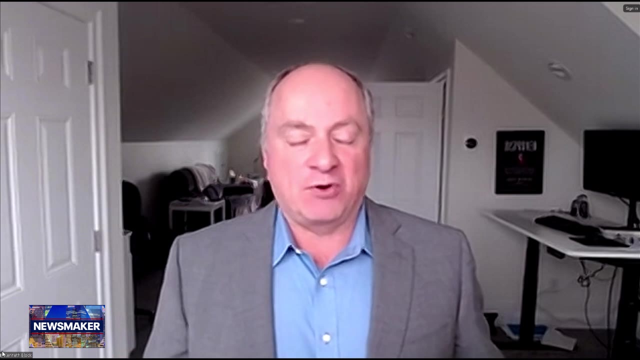 Interestingly, I predicted a vote cast in the name of a dead person before it actually was cast. As a little side note, I might be the only person in the United States history who's done that. Uh, just a small number of dead votes. hundreds of duplicate votes cast across the swing states. 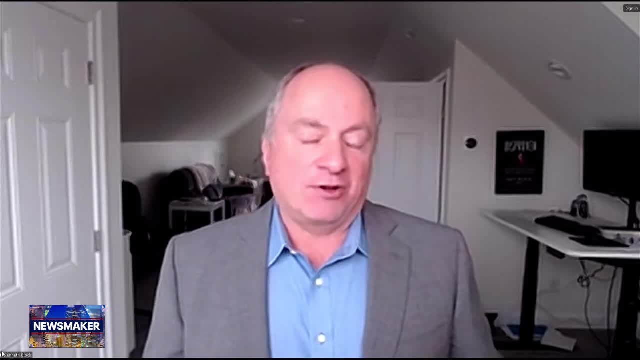 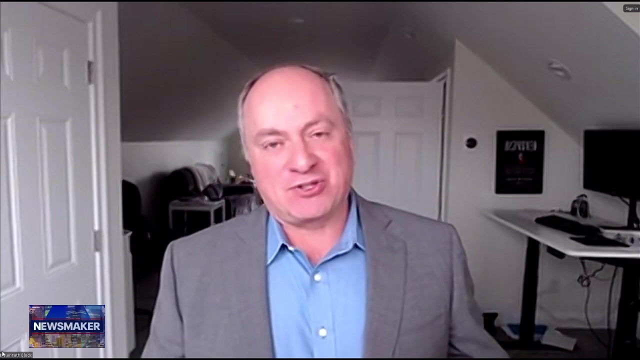 combined Not nearly enough. And what was nearly enough? Well, I mean your listeners know that, uh, the margin of victory in Arizona was between 11 and 12,000 votes. Nevada was roughly 11,000 votes. Michigan was 150,000 votes. Uh, Pennsylvania was 90,000 votes and, infamously, Georgia was. 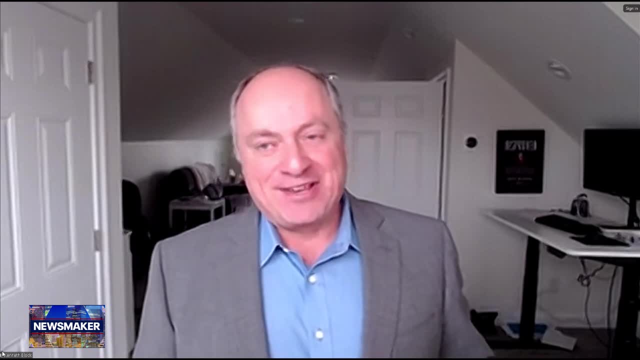 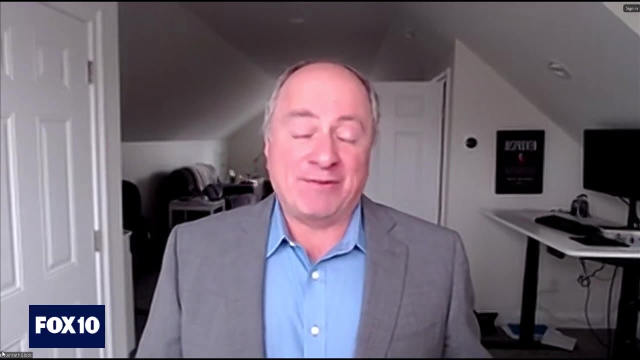 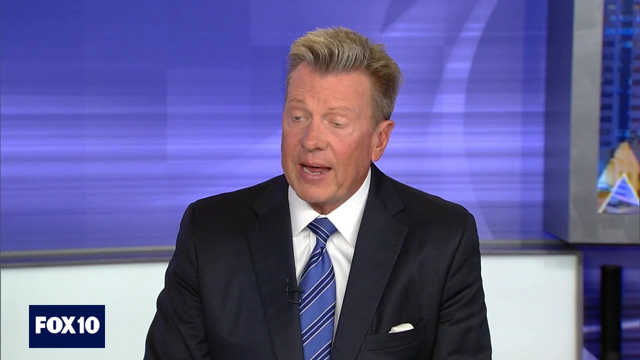 11,789 votes, Yeah, So the you need a lot of votes to cover those margins And, uh, the bottom line was we didn't come close to finding them. One thing that struck me is the timeframe. You have 35 days to do this work. That is a tight. 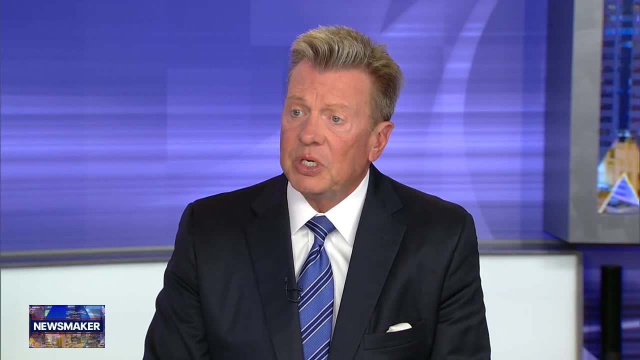 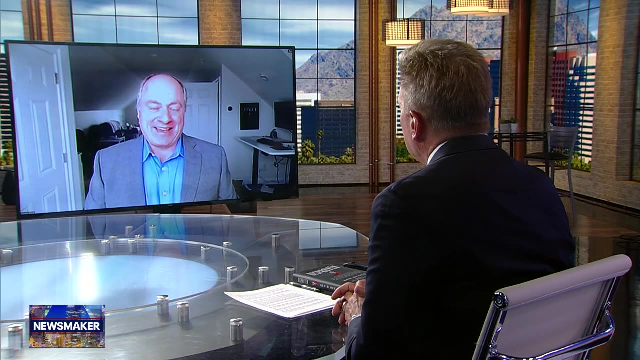 timeframe to do an audit on a national election, Do you feel? are you confident, Bananas? Are you confident you got it? Uh, and, and just if I was only focused on looking for the fraud that my contract uh bound me to. do. it would have been a very tight timeframe. And why 35 days? Well, the 35 days is because, in our legal system and per the wording of the constitution, your only real legal window to contest the election result is up until the day each state certifies the their election results. 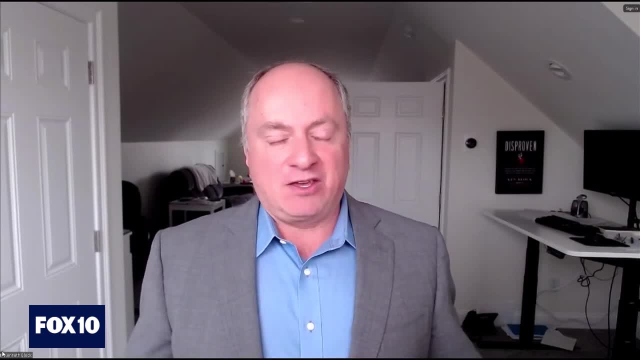 Once those results are certified, legally speaking, you are blocked out from having a successful legal challenge to the election result, And a lot of people don't understand that. Yeah, Uh, so that's what put the pressure on everything, But on top of looking for deceased voters. 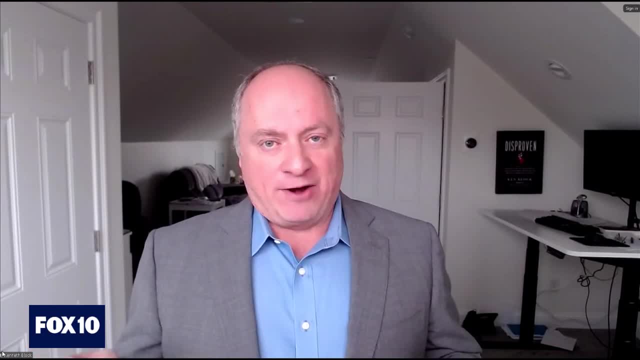 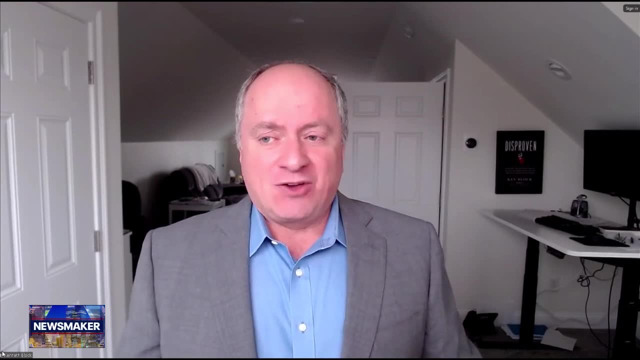 and looking for, uh, duplicate voters, where the data that we were working on was an extremely poor condition. Uh, and in a in a state like Nevada, we had to get 17 different files that contained the mail ballot votes from that state, And each one of those files was: 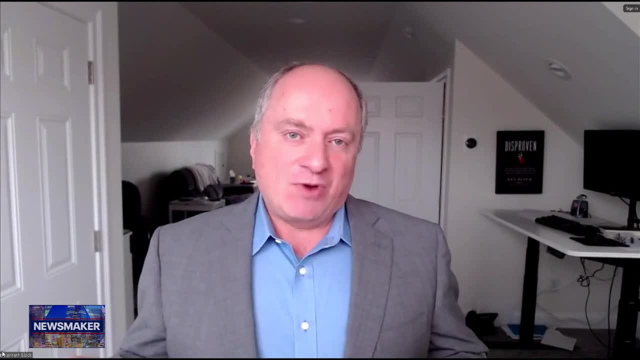 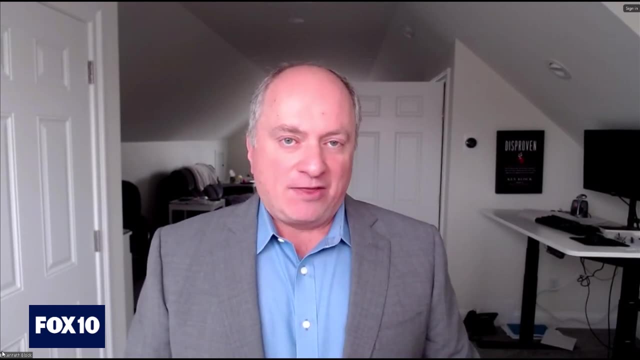 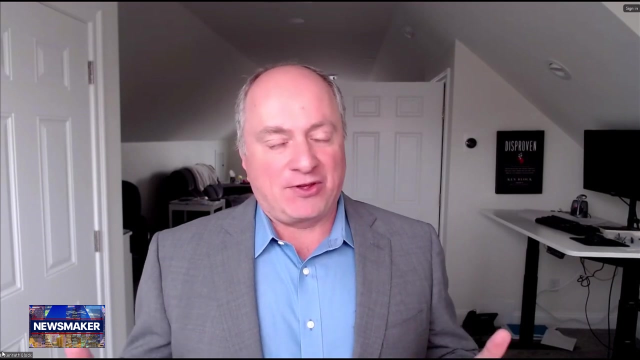 different. It was a monumental task, But then we were then very quickly asked, soon after the contract began, to start assessing claims of voter fraud that others made that were just just cascading into the campaign And they couldn't make heads or tails out of whether 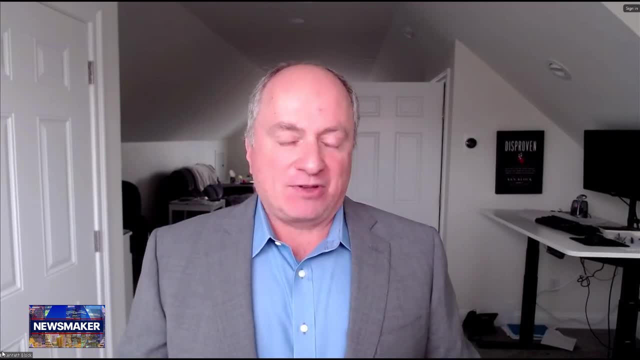 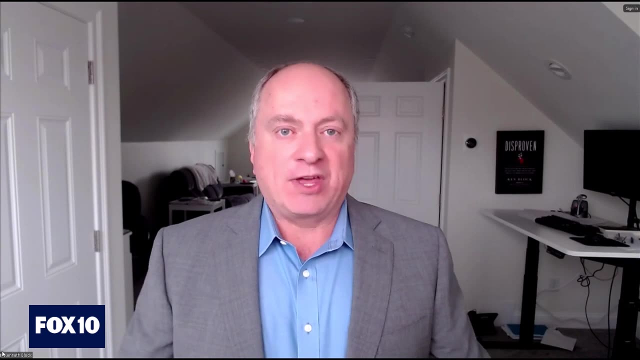 they were accurate, whether they were inaccurate, And what Alex asked me to do from the second day of my uh engagement was to look at these claims and tell him whether they were true or false. You had to vet those. There were about 15 of those where people said I saw something. 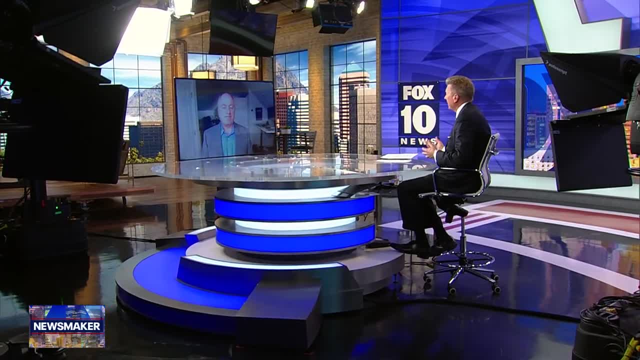 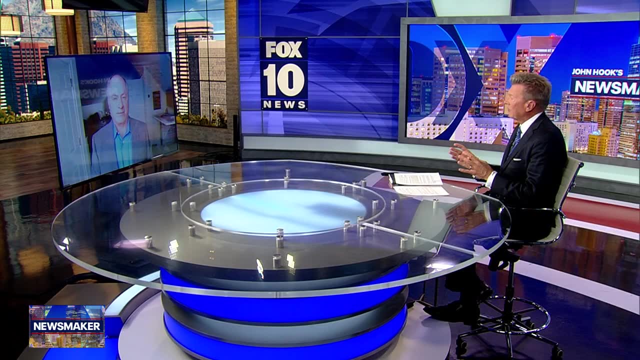 I talked to an election worker who saw some shenanigans. I met this person who told me this story. You had to run that down, But my point was: 35 days is such a tight, tight time frame. Are you confident in your heart of hearts that you didn't miss anything? 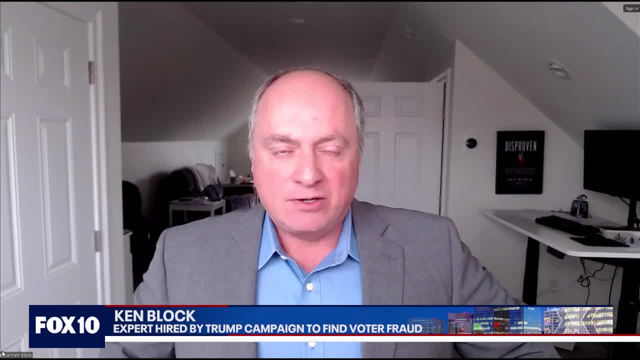 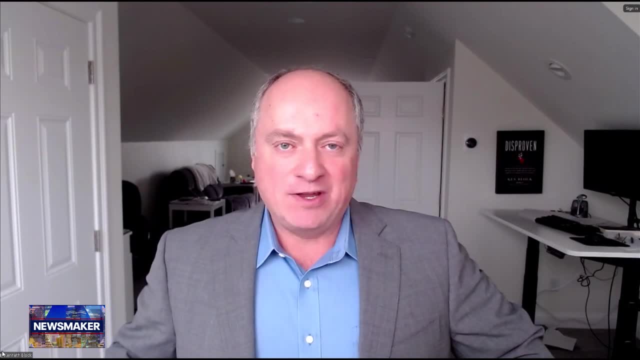 I am And and the, the. I have two different reasons for feeling that way. Uh, the first one is we still evaluated 21 million uh votes cast across the swing states, And when the question arises about deceased voters, I can state unequivocally that we looked at every single. 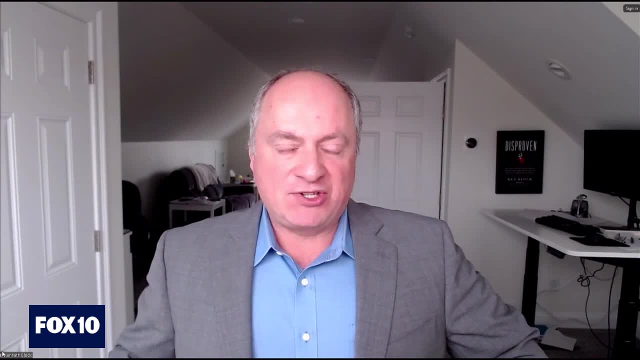 mail ballot that was cast and the number of deceased voters that were cast, And I can state that we looked at every single mail ballot that was cast and the number of deceased voters, that we looked at every single mail ballot that was cast and the number of deceased voters was tiny. 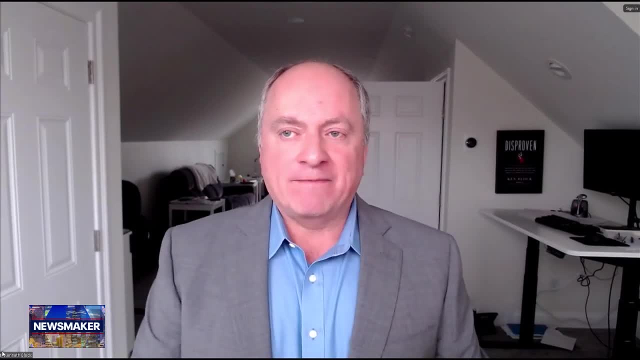 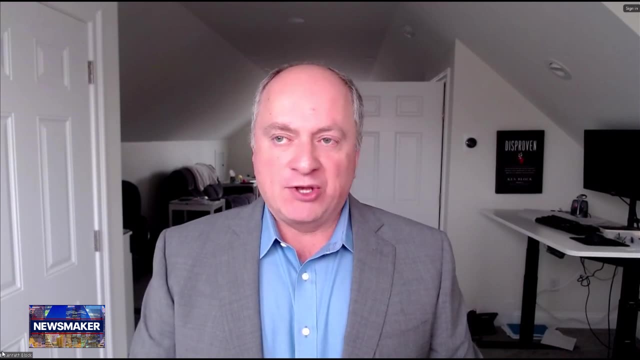 And that's done There. there, there is no wiggle room on that For the duplicate voters. the piece of information that was missing from every state that we looked at was in-person votes, For a reason that I still don't have my head around, uh, no state provides who voted in person. 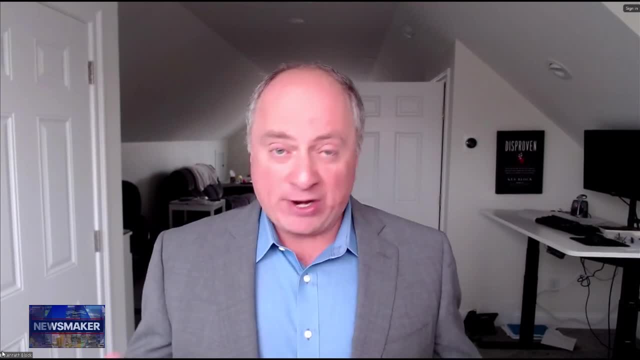 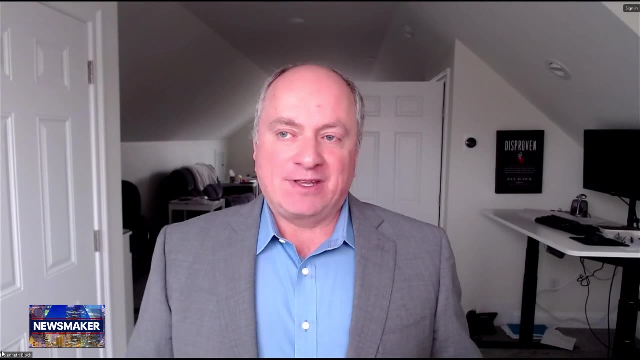 before the results get certified, And that's a weird statement of fact. I can't explain to your viewers why that is, but it is. I mean certainly for a a if you're not going to be Corps weeks, but that's a weird statement. 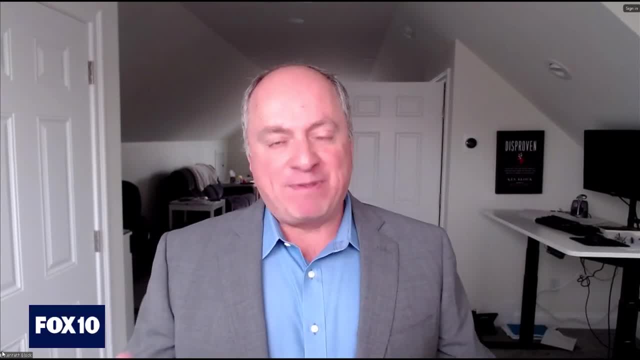 Yeah, it is So. uh, partly it also also gives particular pleasure to to to to notice that there wasn't like Stefano on the, the, the, the, like наш vibes towards the duplicates, which means that in some states 30,, 40, maybe 50% of the votes weren't there for us to assess from the duplicate vote perspective. But the reason I can say it doesn't matter is because there were so many people spending so much money looking at this election, trying to prove election fraud after the votes were certified that if there were a bomb in those in-person votes, that bomb would have been detonated, it would have been shown. 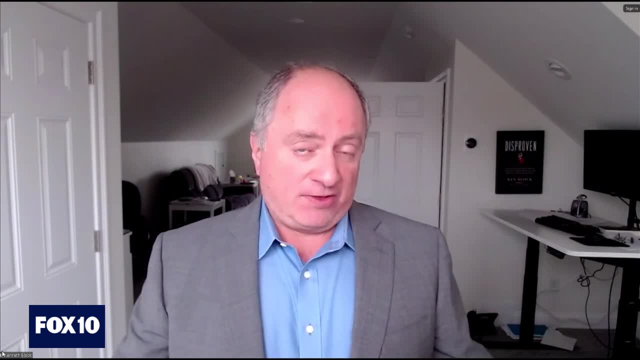 Uh, and there was another cases here too, because they're bipartisan against PACOS and other uh to�fferloh and operators slash voting rights over election rights And there would have been a reckoning to deal with the fallout of that kind of a claim and the proof. That proof was never brought forward In 2016,. I did a very similar exercise months after the 2016 election. I found about 8,000 duplicate votes cast across 21 different states, including most of our largest states, But of course, in a close election. if you take Bush v Gore Florida in 2000,, you've got 547 votes that separated the two. 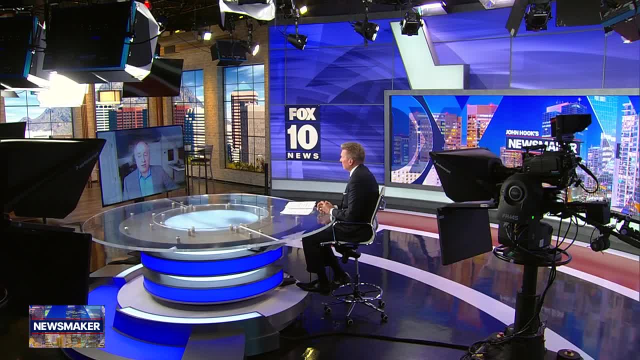 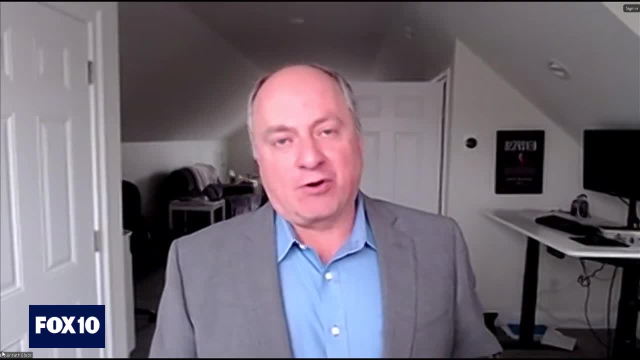 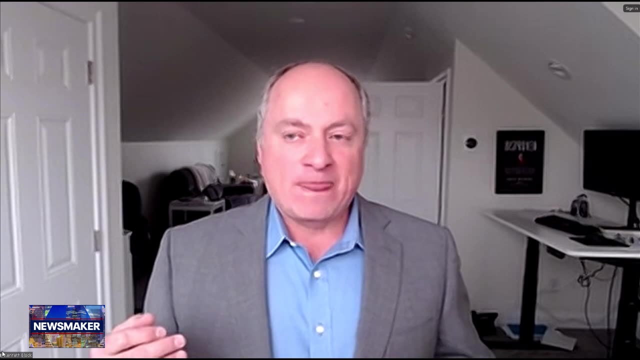 Then it would matter. It would matter, And in 2016,, I found more than 2,000 duplicate votes that were cast in Florida and also in some other states, So there was a problem. Now, all of this was happening before more tools were brought to the table to help identify duplicate registration. 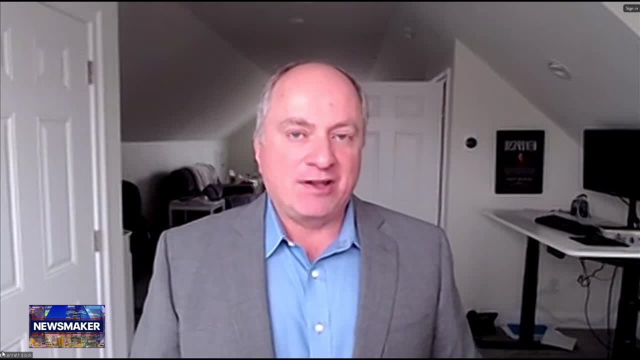 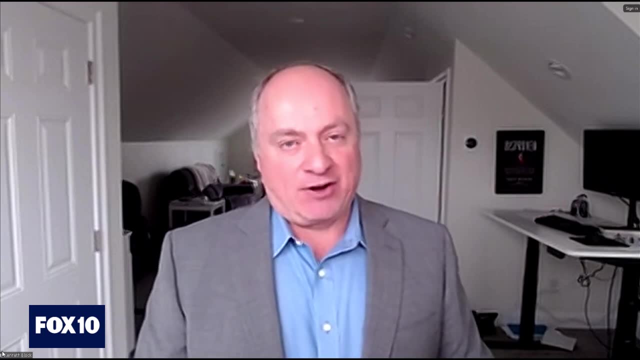 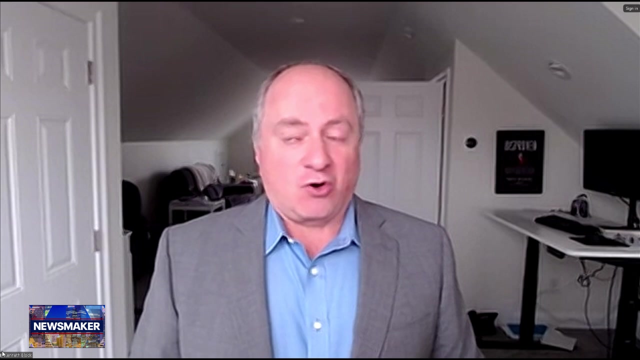 Across states. a consortium of states called ERIC, whose purpose is to look just for this sort of thing, got going And those numbers dropped after ERIC became effective at finding some of these duplicate registrations. But you're right: 547 votes across 2,000 duplicate votes in 2016, you're well above the margin of victory. 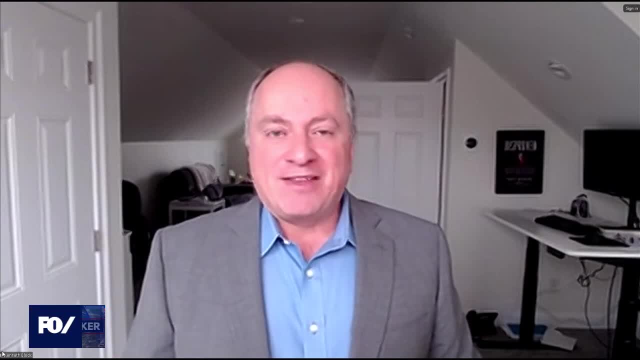 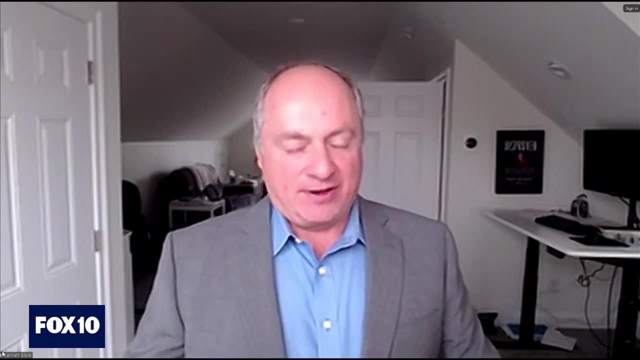 But here's the thing, And this is—I'm sure you're going here with this- What very few people understand is that— When we vote, our vote is anonymous. You can't tie the voter to which candidate the voter cast a vote for. 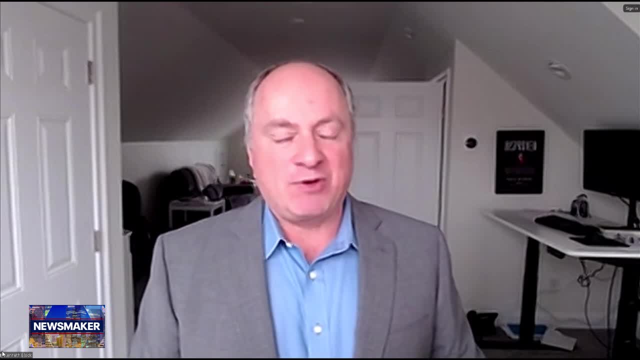 It's done that way on purpose. There are plenty of good reasons why we do that, But because the vote's anonymous- what we can never know— Let's use Arizona as the example. Let's imagine—I didn't, but let's imagine I found 15,000 fraudulent votes cast in Arizona and I didn't. 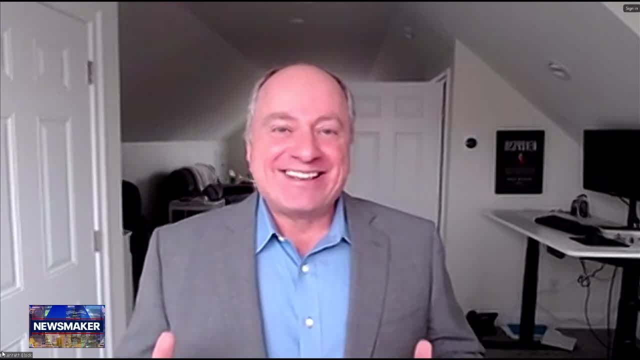 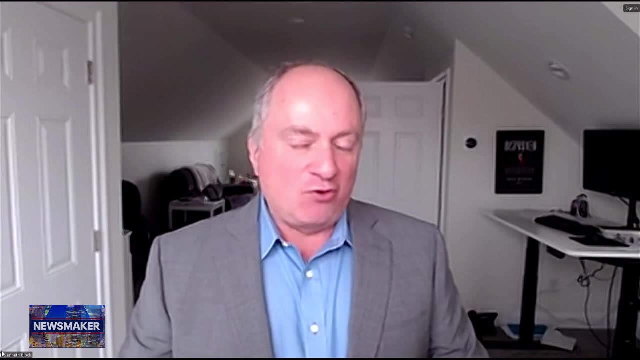 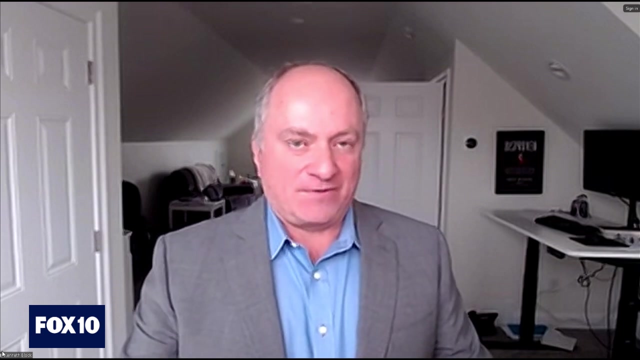 I just had to be really careful when I created this scenario. So let's imagine 15,000.. No court would overturn the election with 15,000 proven fraudulent votes. Let's imagine they're all dead Because we can't show for whom each of those fraudulent votes was cast. 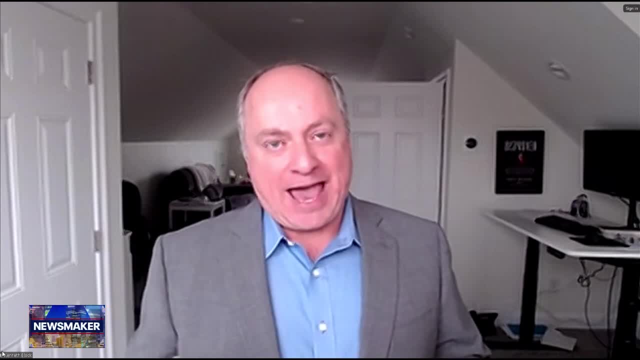 The candidate challenging the election has to be able to prove harm, And you cannot prove harm because we vote anonymously and therefore all these legal challenges were really probably doomed to failure. We can't show for whom each of those fraudulent votes was cast. The candidate challenging the election has to be able to prove harm. 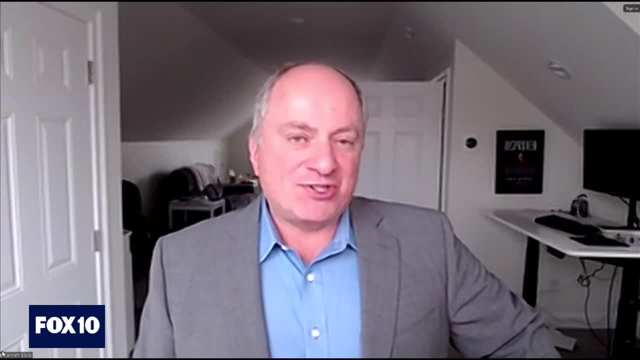 Because we can't show for whom each of those fraudulent votes was cast. The candidate challenging the election has to be able to prove harm, And so I realized that if I had to prove failure from the word go- that wasn't something that I realized as we were getting into it- 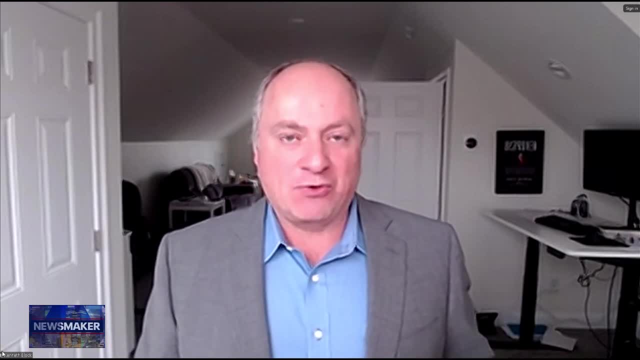 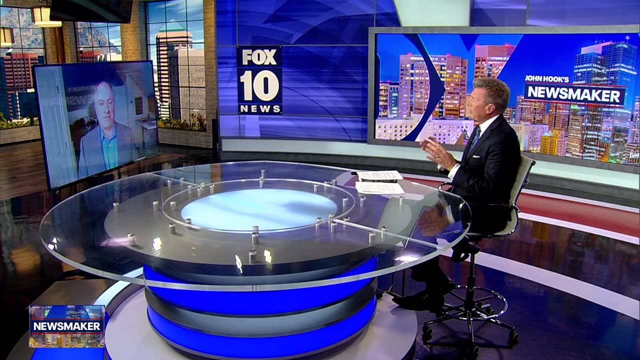 It's only something that I realized about three-quarters of the way through doing the work. Yeah, that is such an important point in your book and I was going to go there. Thank you for that. But with that in mind, you've looked into this in the past. 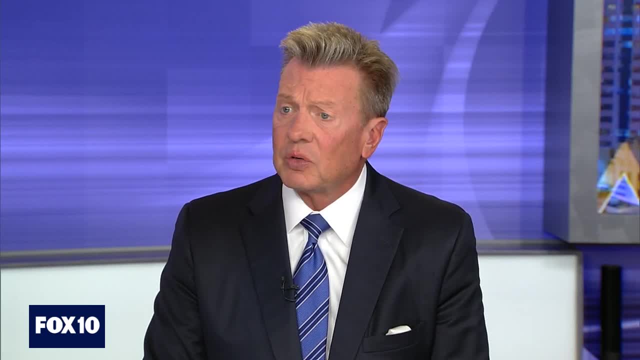 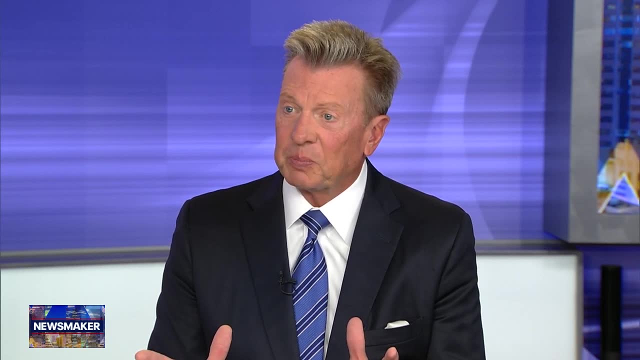 You've gone over voter data. I think for over 10 or 15 years you've been doing this stuff. Yeah, You kind of found that usually the fraud is— It's pretty evenly split between Republicans and Democrats. Yeah, So let's talk about the different kinds of fraud. I can give you some different percentages. When it comes to voting in two different states, it's a crime of privilege. It's usually people who own multiple properties in multiple states, And in Florida it turned out that the voter fraud skewed for duplicate votes about 60-40,. 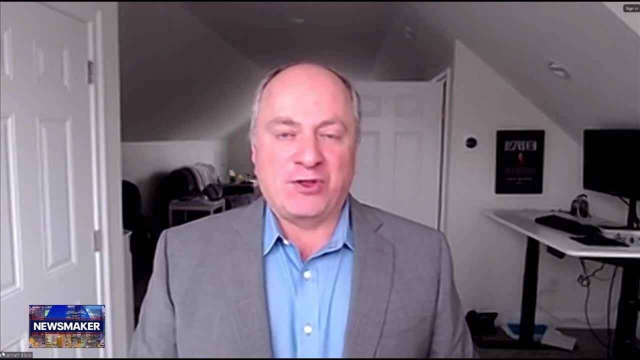 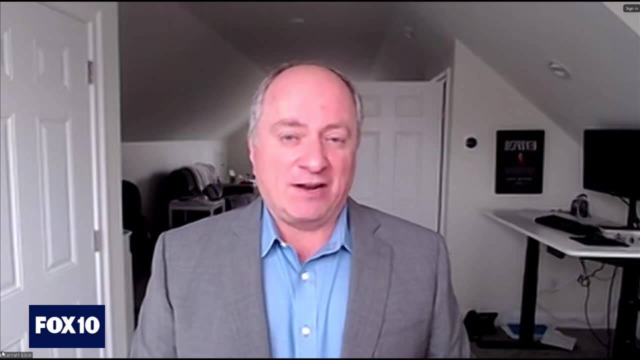 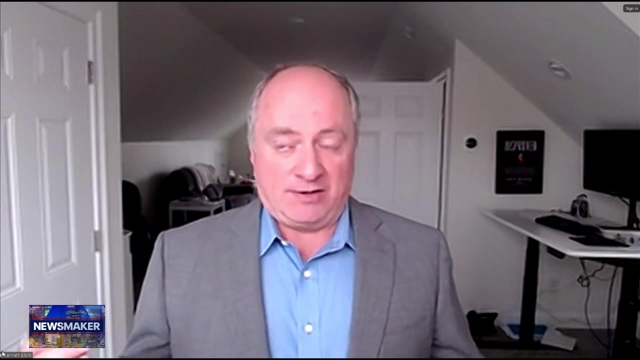 where 60% was Republicans- For the deceased votes in— In Pennsylvania, especially the one that I predicted and a few others that were prosecuted- the deceased votes that were prosecuted and where charges were—and a sentence was—a conviction was made. in both instances those were Republicans who admitted that they had cast votes in the name of their deceased relatives. 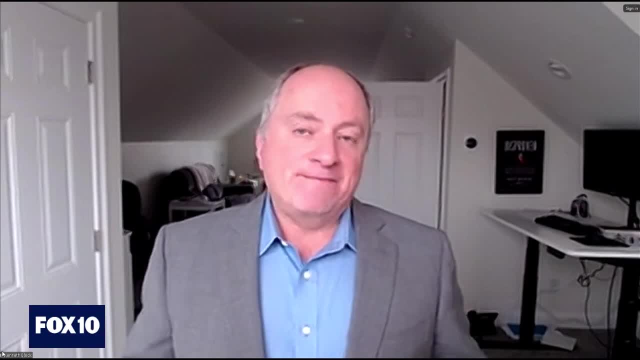 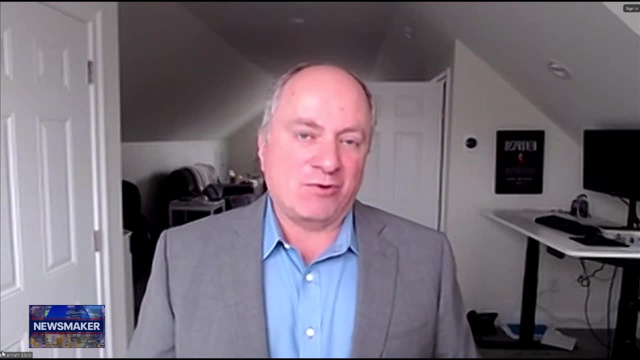 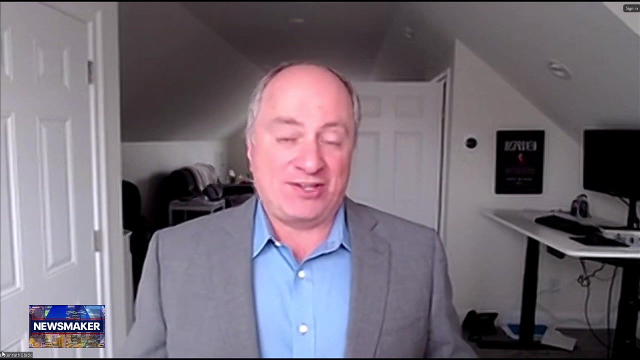 and that they had done it for Trump. So the narrative that only Democrats commit voter fraud- it's ridiculous. It's really bipartisan. I think some of the voter fraud we're talking about here, especially with the out-of-state duplicate voting, I think it's a crime of opportunity and it's not an—and this is. 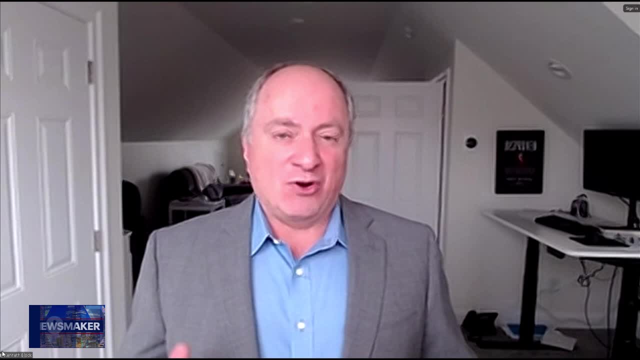 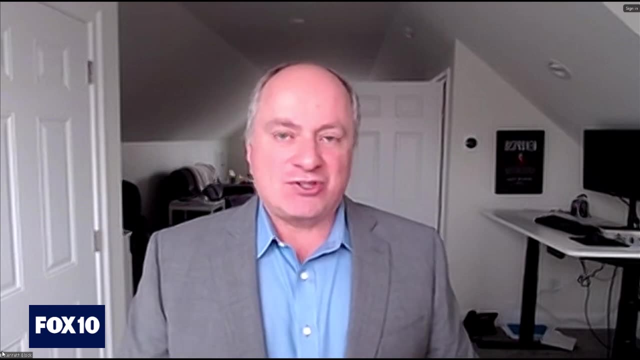 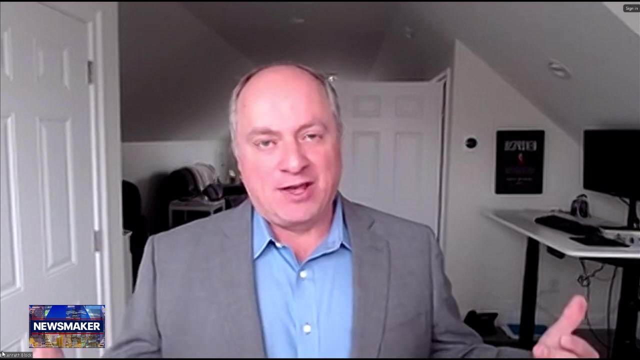 a really important point. I've seen no evidence of an organized, systematized effort for the fraud that I found It's been individuals just taking two bites of the apple because they could. It wasn't like someone sat down and figured out that they were going to cast 500 fraudulent. 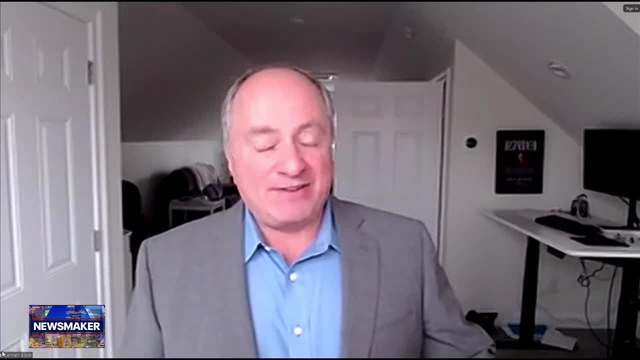 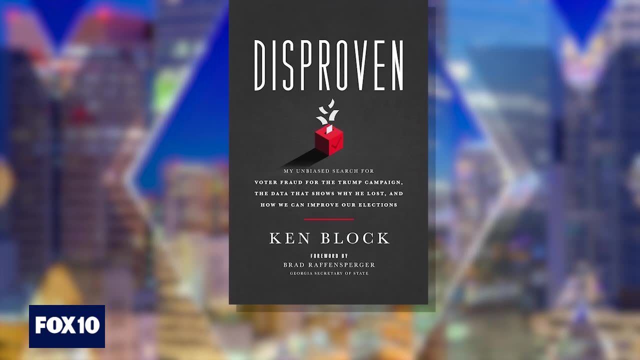 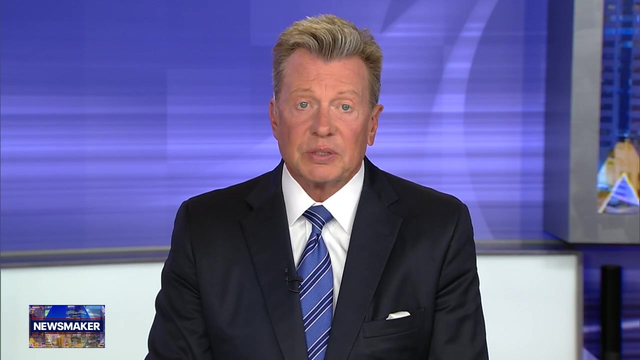 votes by— Voting a bunch of different people out of state. I've seen no evidence of that whatsoever. Ken Block is the author of this incredible book. Disproven My Unbiased Search for Voter Fraud and for the Trump campaign: the data that shows why he lost and how we can improve our elections. 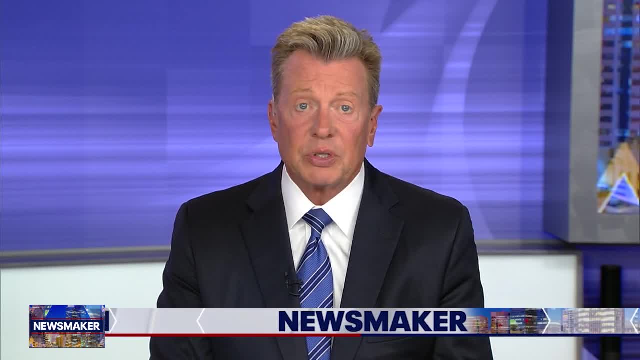 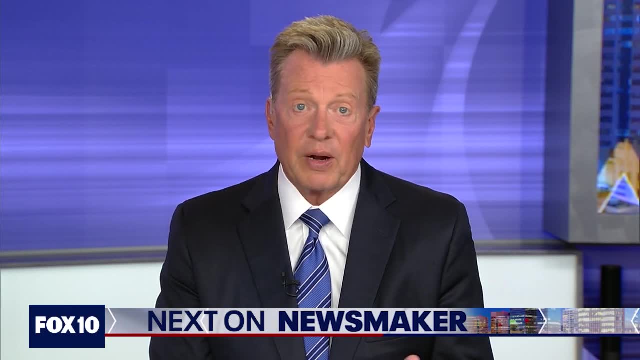 Ken Block is my guest on Newsmaker. We're back in a minute. We're going to talk about Arizona in that stack of five states that he really looked at- swing states. How did Arizona perform? How do we do on elections? 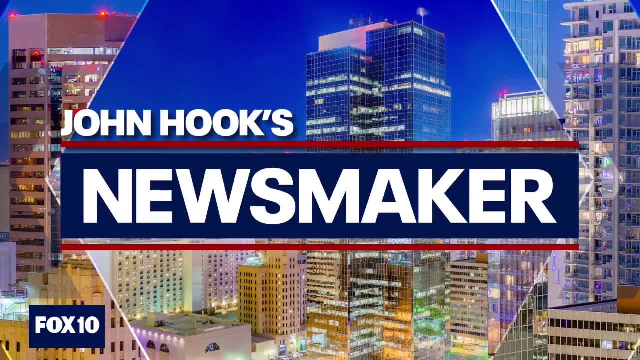 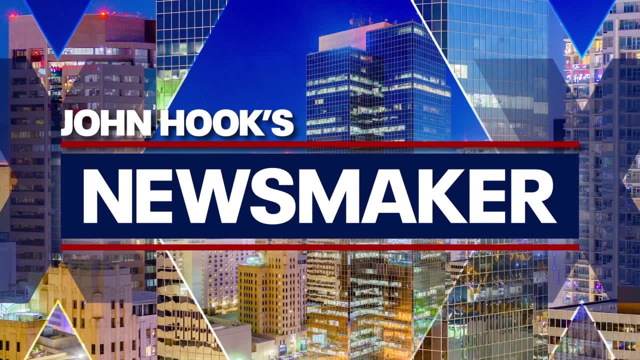 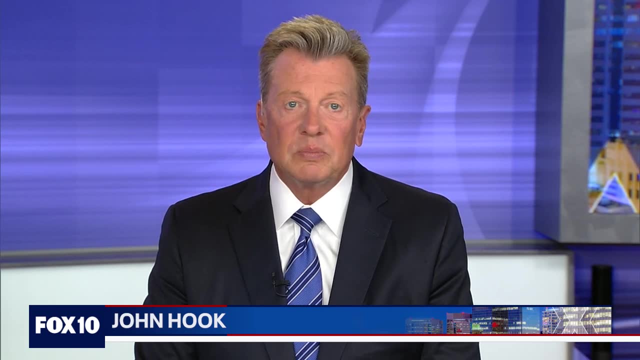 And what can we do to make a difference? And what can we do to make a difference And what can we do to make a difference And what can we do to make it better? Still ahead on Newsmaker Back with Ken Block, the man who was hired by the Trump campaign to look into claims of voter fraud in 2020.. And what he found was surprising, but not for the reasons you think. Ken Block rejoins us now on Newsmaker. OK, so you do all this analysis in the five swing states- Arizona is one of them, And you know that we were auditing and we were going back and forth. 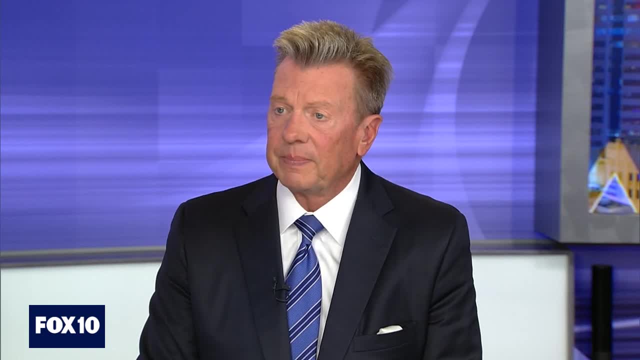 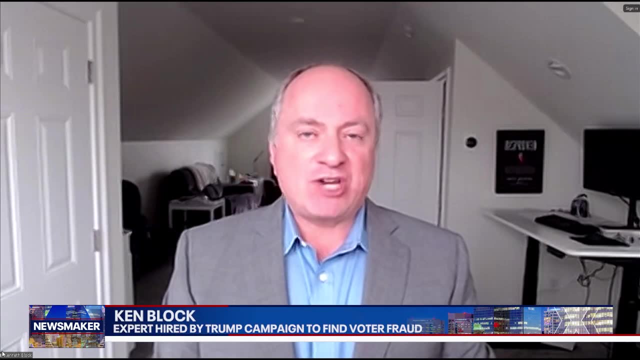 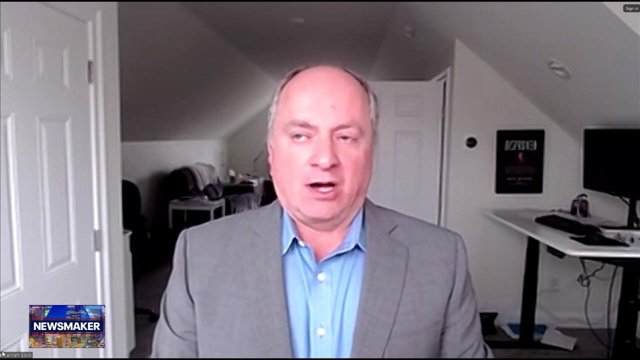 trying to figure out if there was a problem here. What did you find? We didn't find a problem. As we were looking at it. we had some challenges working with Arizona's data. You also have county administration of elections And it looks to me, if I remember correctly, there were probably three distinct computer, different computer systems. 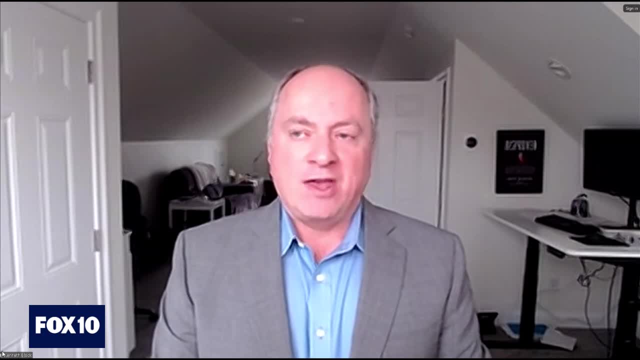 In terms of the different data that we were having to work on work with, and we had some data challenges trying to work with that data in the compressed time frame that we had, but, uh, what hasn't really jumped out at me looking at arizona, not just- 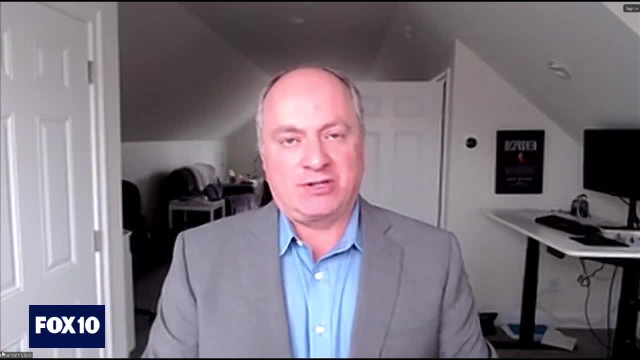 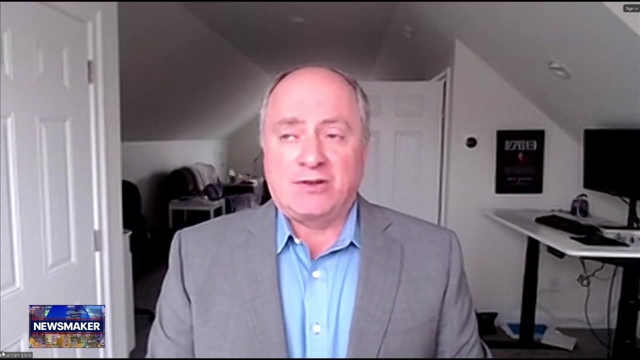 during the work i did for the trump campaign. but as i've looked at arizona at different times, arizona's election data is relatively speaking clean, uh, compared to some other states that have some really terrible problems with their data. uh, and so, uh, as i was talking with alex about, 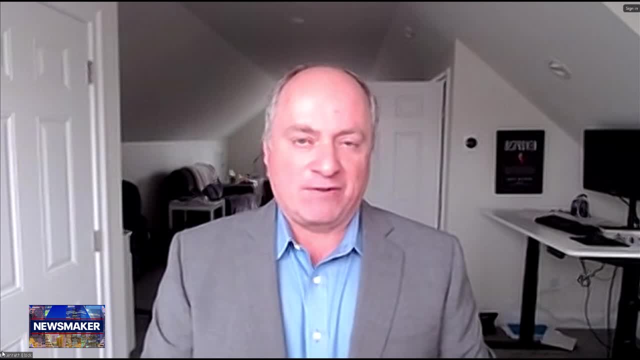 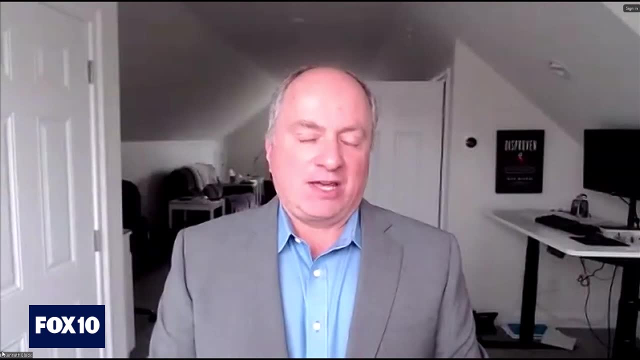 just we had to prioritize and make some decisions on where we were going to focus our efforts. uh, we quickly determined that arizona wasn't going to be a place that we were going to take put the most effort that we were looking at- uh, simply because there just really wasn't all that much. 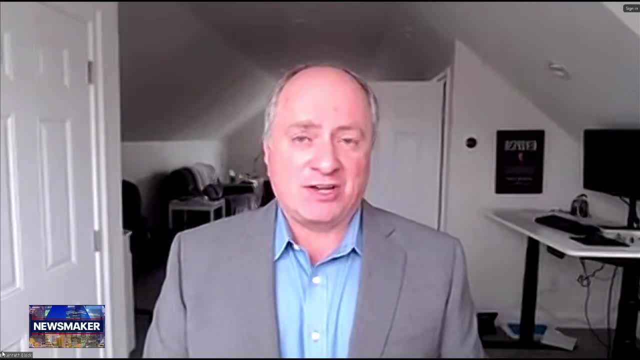 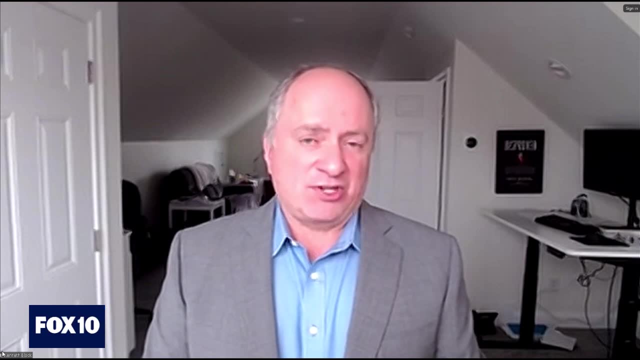 there uh, which i think speaks well to how arizona conducts their elections generally. uh, and i can tell you uh afterwards, and this did. this wasn't a factor while i was doing the work for the trump campaign, but certainly as i was preparing all the data and analysis on top of what i had done in 2020 for the book. 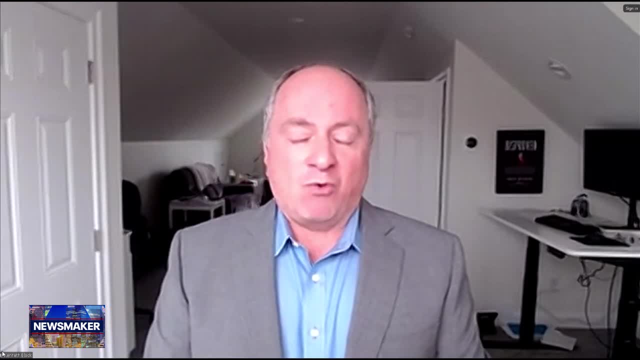 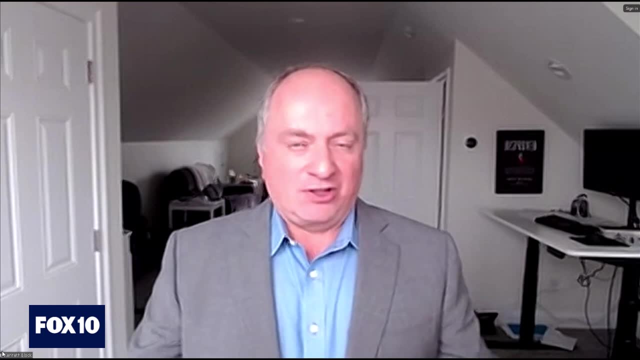 there are some very interesting facts that pop out about what really happened in arizona, and i don't know if this is the time where you want to sort of swing into that or not. um and i'll, you can leave me where you want me to go here, but there there are some very interesting basic common sense. 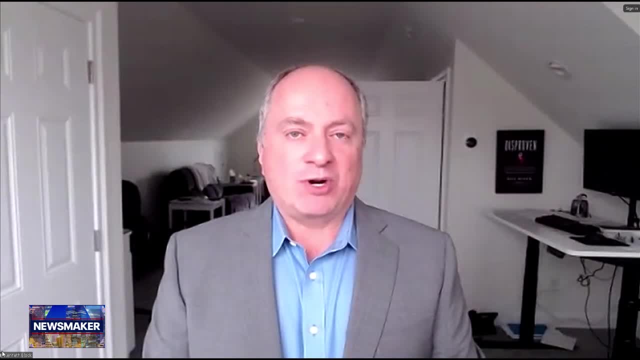 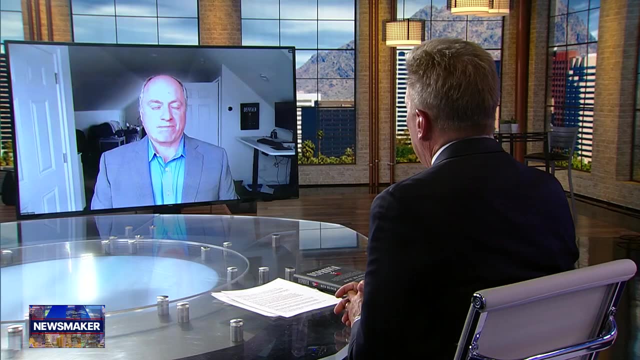 reasons why the election went down the way it did in 2020.. no, we were just going to go there before we got the vote and we're going to go back to the eleventh day of the election. so let me just let me just ask you: when you came back with your findings, how was it received by the trump team? 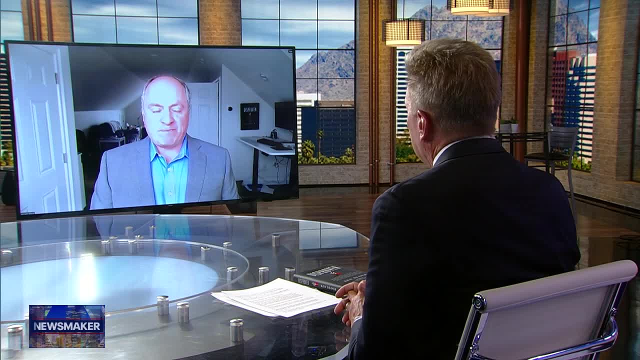 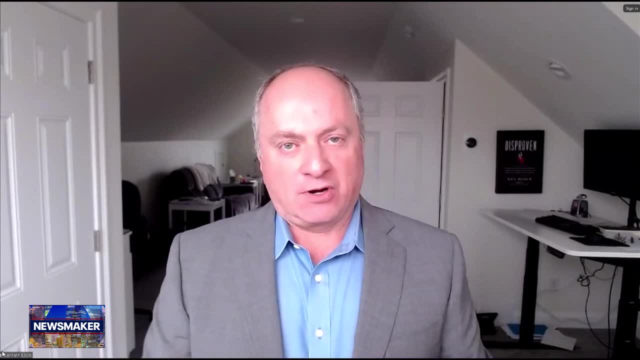 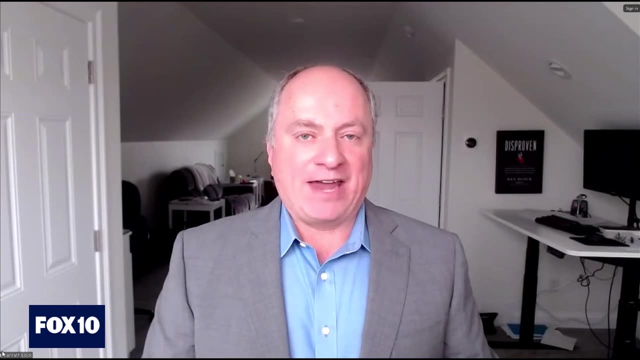 you basically said: it's guys, i've looked, it's just not there, sure. so just bear in mind that not only was i dealing with my work looking for deceased voters and looking for uh duplicate voters, i was also being presented claims about uh dead people voting in pennsylvania that others had brought forward. 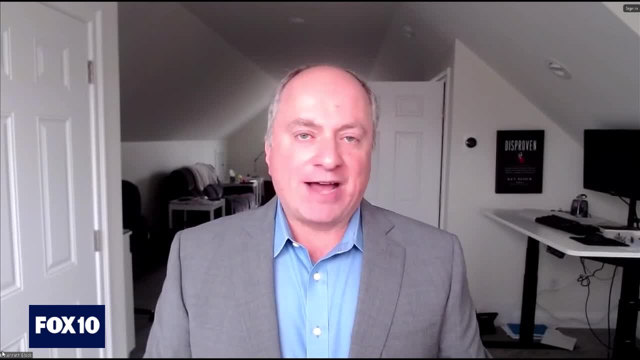 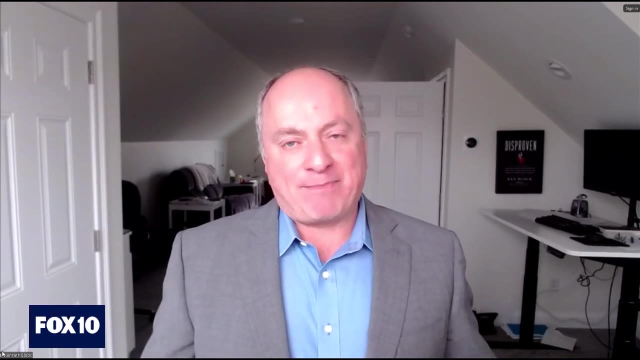 i was asked to evaluate a claim of 20 2500 non-citizens casting votes in arizona. i was asked to deal with a crazy claim that 740 000 duplicate votes were cast in wisconsin fraudulently. so all of that was happening at the same time and on a daily pace basis. alex was calling me and we 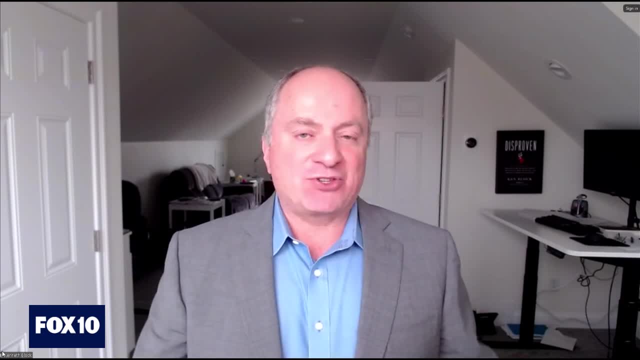 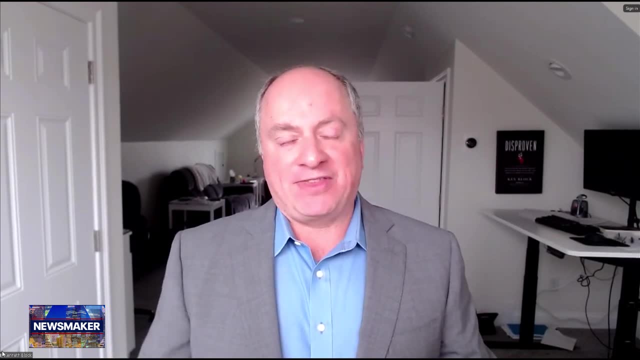 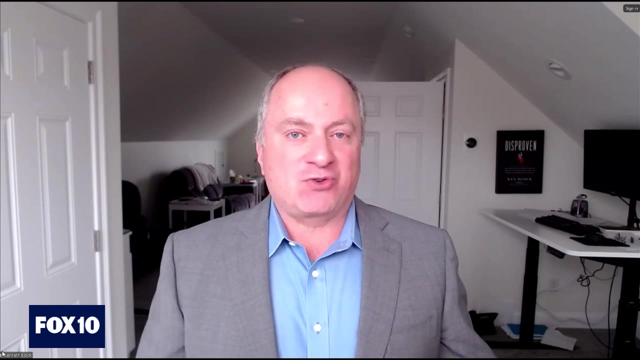 were talking about the, the claim of the day that i had to have an answer to in a matter of hours, and those claims started off with him asking me whether it was true or false, and at the end he was just saying to me: tell me why this one is false. so there were, there was enough history and there were some basic. 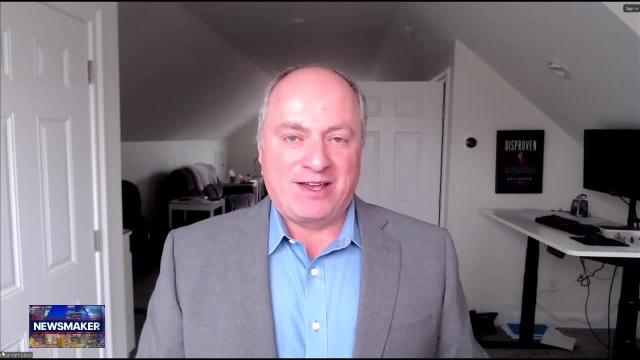 problems that every claim stumbled into, where he realized that none of these claims were ever going to evaluate as true. and when alex was subpoenaed by the january 6 committee in in his uh deposition transcript and in the one minute they broadcast him on tcv. 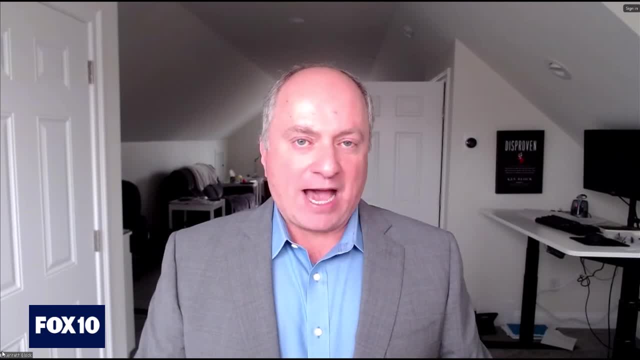 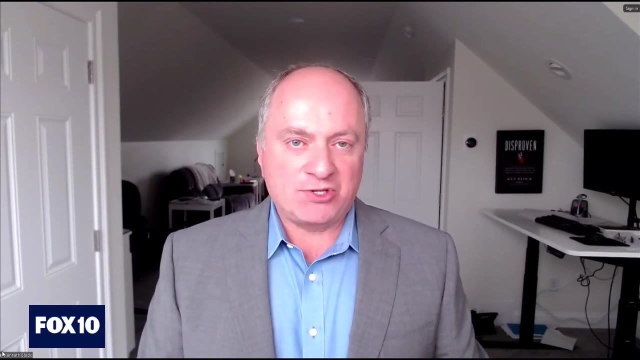 during the hearings he described how he brought the campaign's findings in their work looking at voter fraud to mark meadows- and he- and mark meadows, just to remind everybody, was president trump's chief of staff at the time- and what he told mark meadows was: the campaign looked. 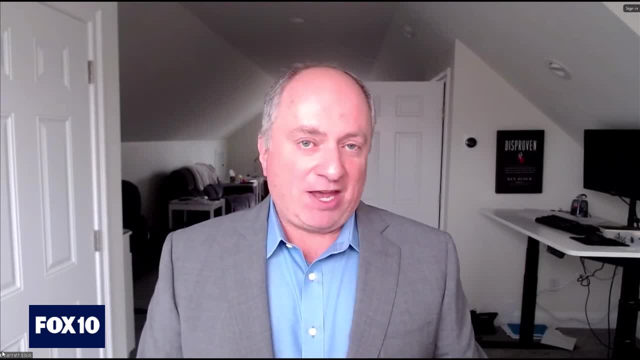 as exhaustively as we could for voter fraud and the campaign evaluated every claim of voter fraud that we were asked to evaluate and we found no voter fraud in. every claim of voter fraud was false and what meadows response to that was: was that means there's no? they're there meaning? 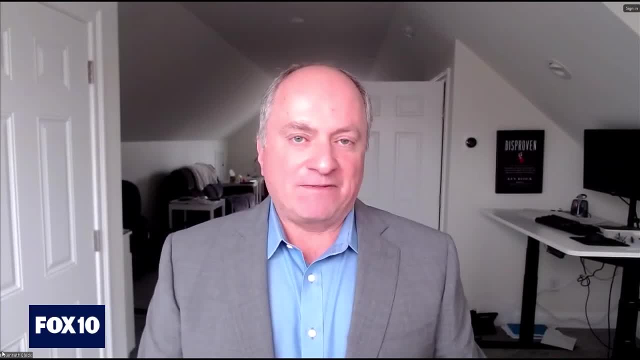 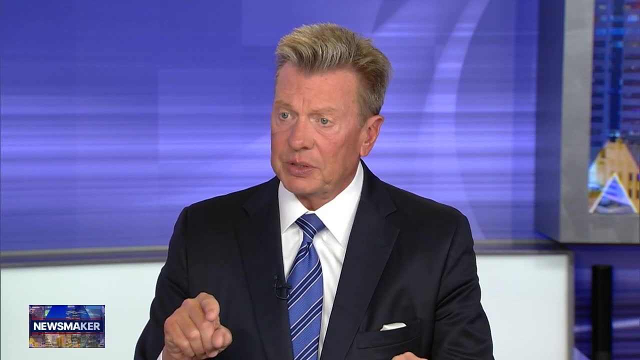 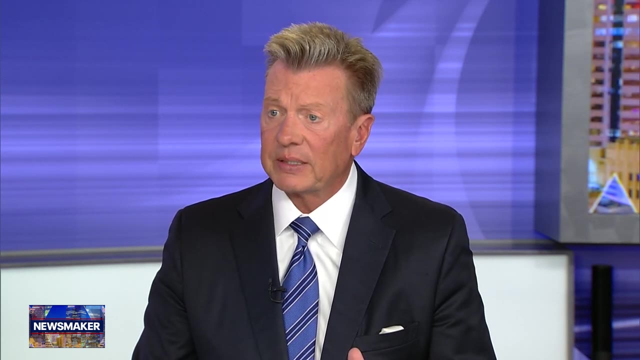 that the claims of voter fraud had no foundation. in fact, we should point out, there was another group looking at this at the same time- you were the berkeley group. so there were different agents diving into the data to try to figure out: was there fraud? you came up empty, which you kind of expected. 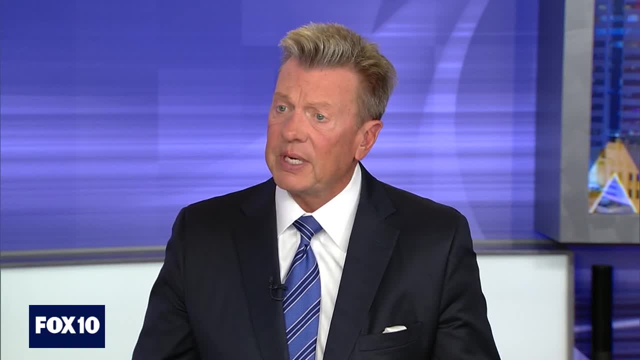 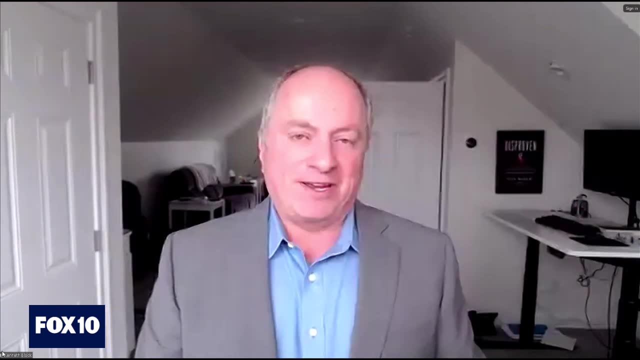 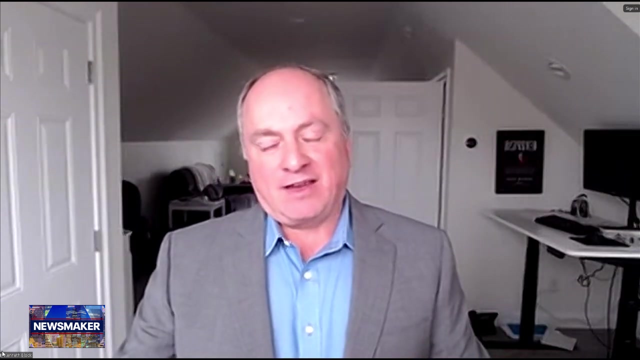 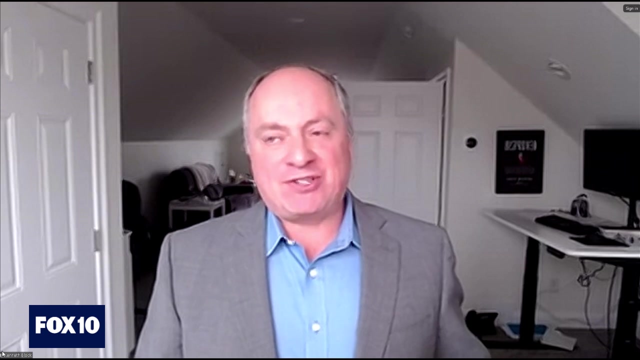 berkeley group didn't find it. nobody has found it since correct the so and i think it's worth. this is actually a really important thing to talk about here. so you have evidence that is legal in nature and then you have evidence that is political in nature, and they're two completely different things to make statements about voter fraud. 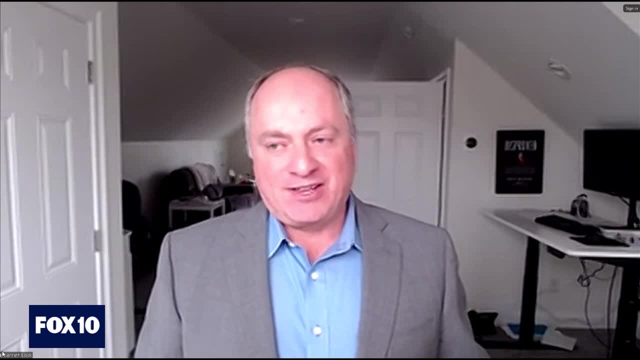 in the with the, the viewpoint of politics. you can say just about anything you want and you can think about different things you want, but you know you think about everything thatnothing out on your yewell. or you know a bunch of articles that use as your evidence hearsay evidence. well, 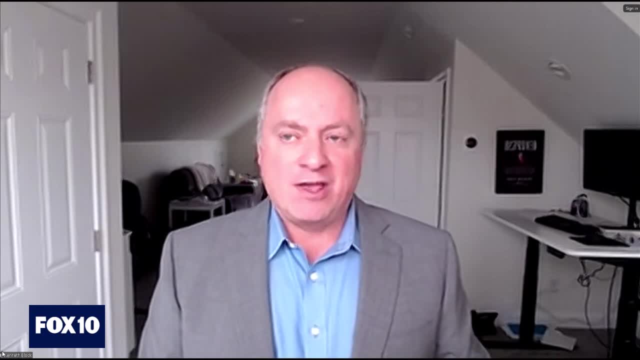 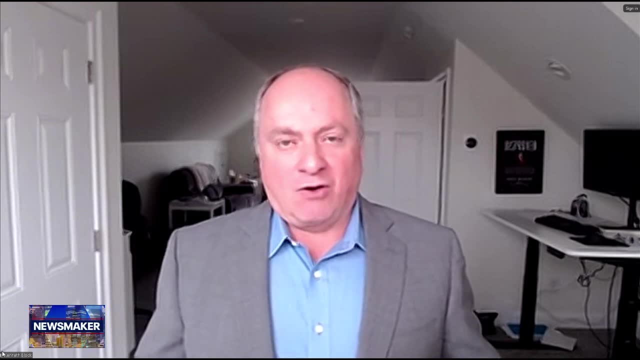 you know, joe, saw a bunch of ballots in a ditch, or this or that or bamboo in the the ballot paper, whatever right, these are all hearsay claims and and they're they're very unlikely to ever stand up in court. but they're not really intended for court. they're more about public opinion and PR and 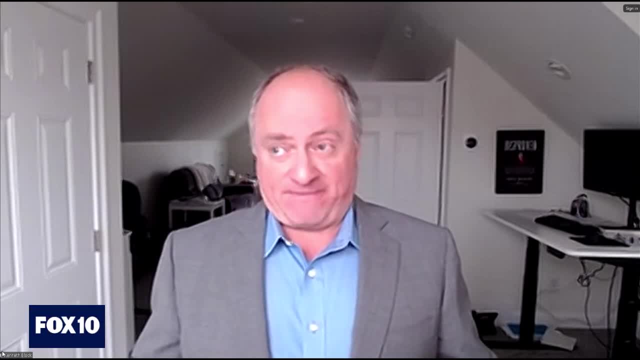 that sort of thing, uh, whereas if you're serious about impacting the election result and you want to prevail in court and you want the court to come to a higher level, isn't just correct to take some fundamentally unreal action in terms of overturning an election result or 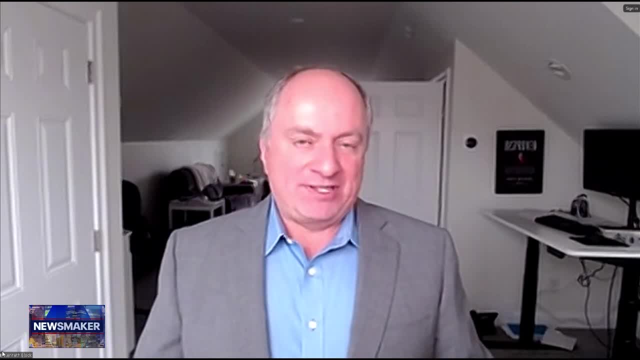 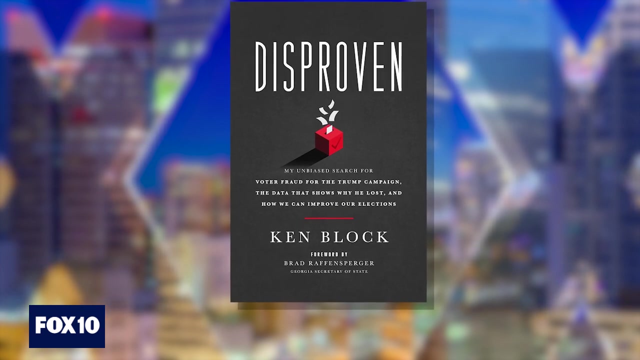 recasting an election, you've got to come with data and with proof that is unimpeachable, And nobody has come forward with unimpeachable proof of fraud, Never. Yeah, Let's talk about- and this gets into the section of your book- Why Trump Lost. 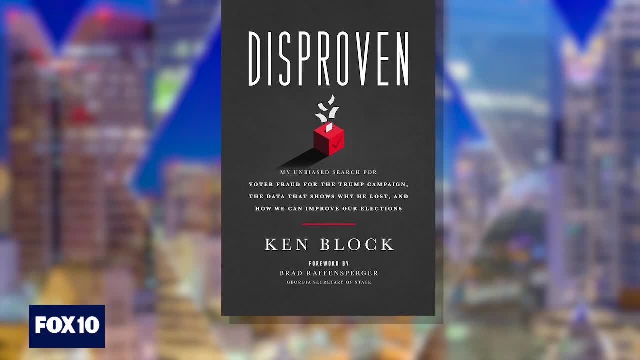 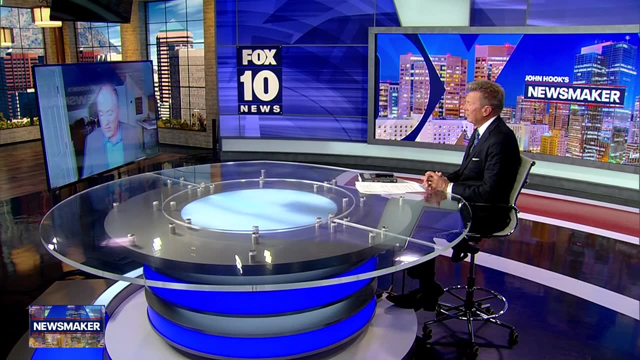 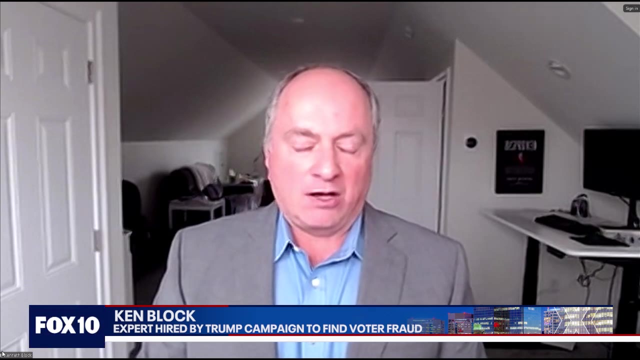 And this gets into Arizona. what happened here? Maybe you use Arizona as a springboard for that, but you say that it's very basic. what happened, Explain? Yeah, So there's actually a couple of different, perfectly explainable and understandable events. 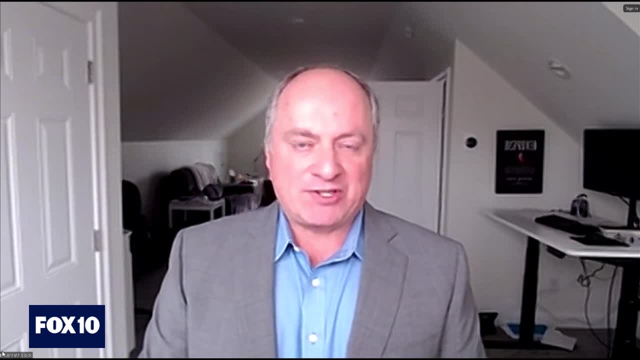 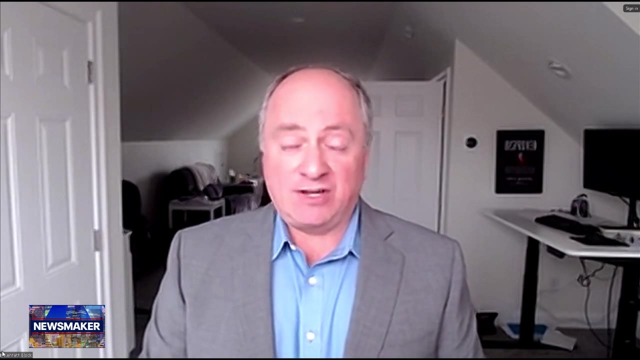 that happened during this election. In most of the swing states, the Libertarian candidate for president took more votes than the margin of victory, And in the 2020 election, the Libertarian candidate was Donald Trump, Joe Jorgensen, And she did very well. 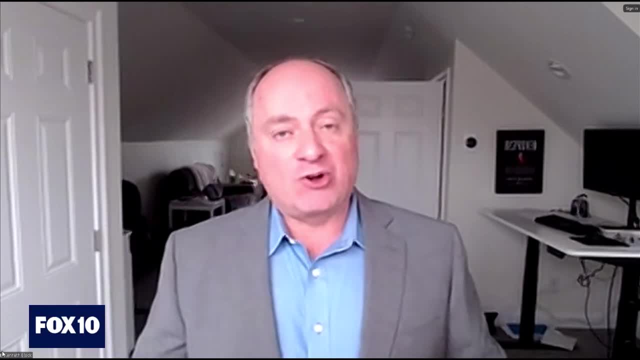 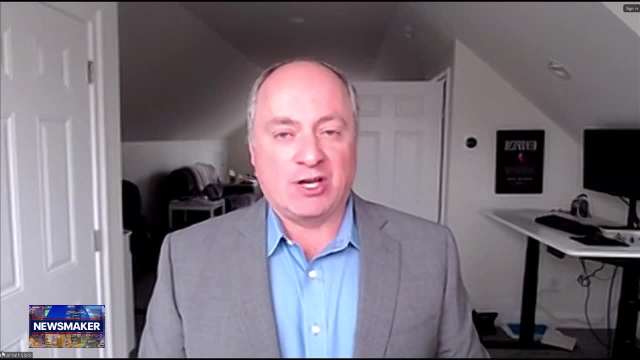 She took almost 90,000 votes in Pennsylvania, which was the margin of victory in Pennsylvania. She took more than 50,000 votes in Georgia and the margin of victory was 12,000 votes, And I'm hedging on the number here. 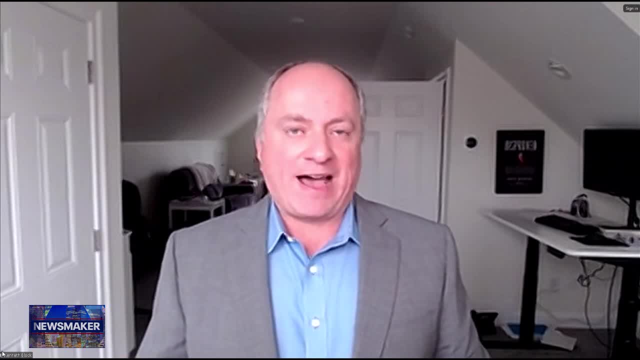 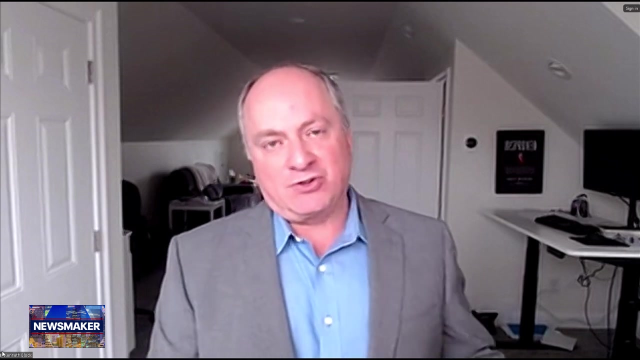 I believe that Joe Jorgensen took five times the margin of victory in Arizona as well. So that's an amazing thing. That's an amazing finding because, at the risk of generalizing, Libertarian voters tend to lean a bit more conservative than they do liberal. 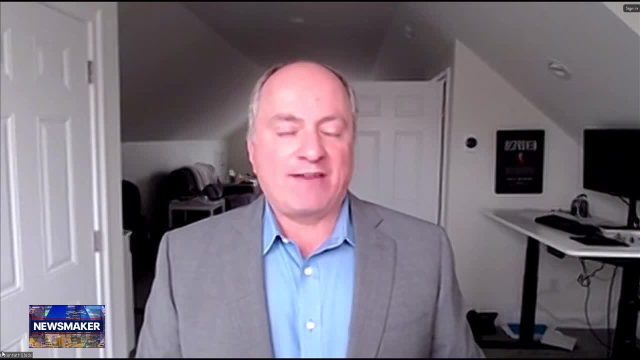 And those were a pool of votes that President Trump should have been trying harder to get. He didn't need that many to have swung the election. So that's one, And those numbers are part of the record. It's easy to see it and you can begin to understand that. 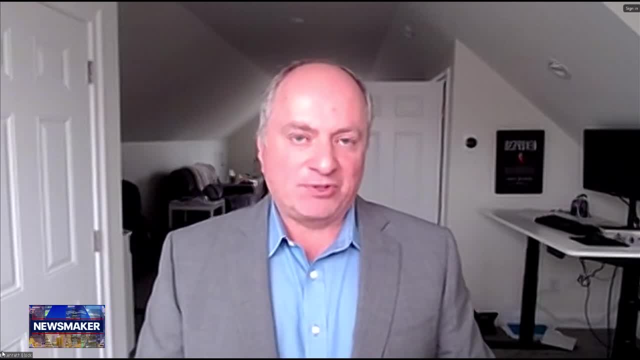 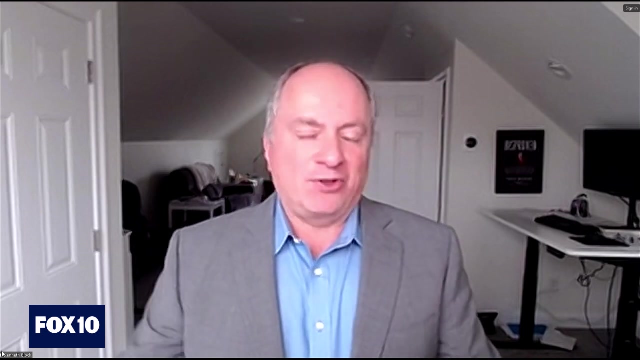 The bigger one, and the one that is evident in multiple different ways- and I have proof of it. Trump's own pollster proved this in a different way- is that President Trump lost the support of moderate Republicans. In fact, he more or less told them he didn't want their support. 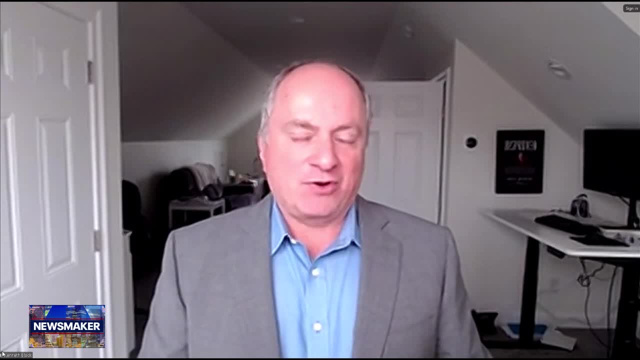 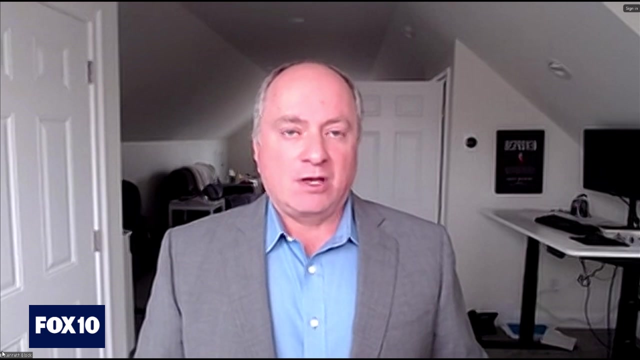 And it shouldn't surprise anybody that a lot of those voters chose not to vote for him. Well, the numbers: when you add up the moderate Republican numbers in Georgia, for example, there were more than 100,000.. 100,000 rhinos who didn't cast a vote for Trump in 2020.. 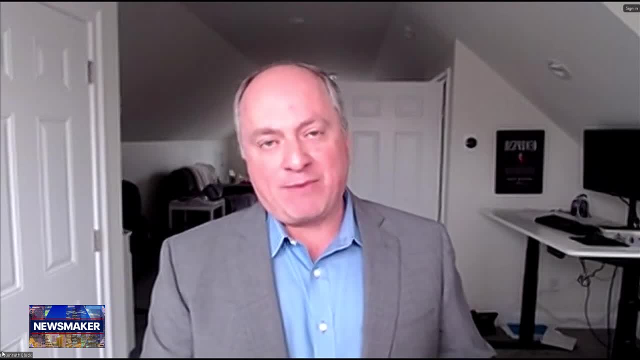 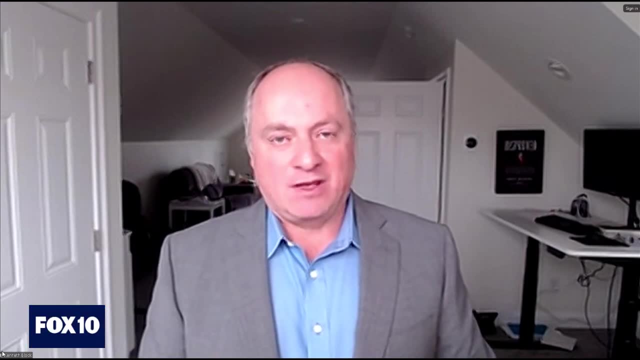 Now, how do I know that? Well, there were 30,000 Republican primary voters who didn't vote in the general election in Georgia. That's twice the margin of victory. Another 30,000 voters in Georgia voted for down-ticket Republicans but left the presidential. 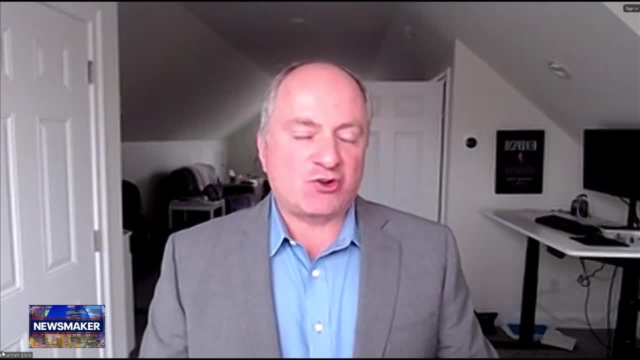 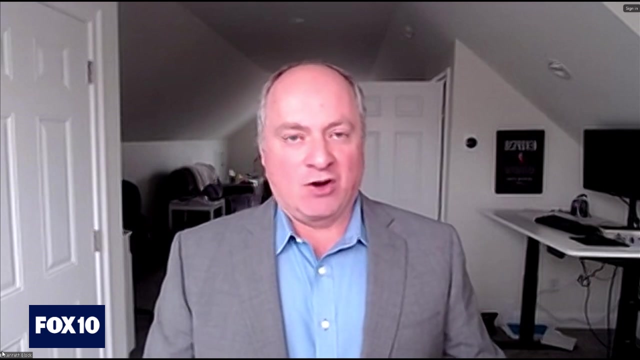 selection blank. That's the rhinos again registering their unhappiness with their choice for candidates. And I saw reports in Arizona where that same dynamic was at play, where there were primary voters who didn't participate in the general and there were ballots where down-ticket Republicans 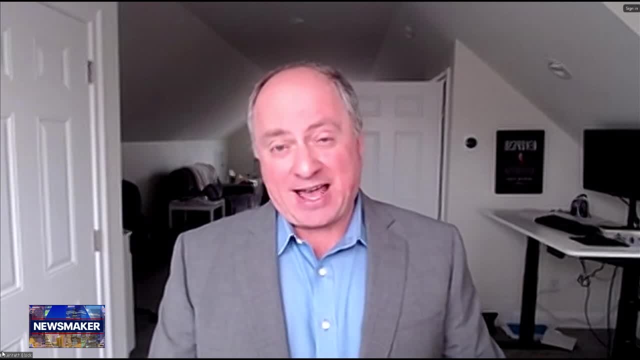 received votes, but the top of the ticket didn't, And that didn't happen in Arizona, And this went for the governor's race too, here as well. That's what I was just going to say. It didn't happen only in 2020.. 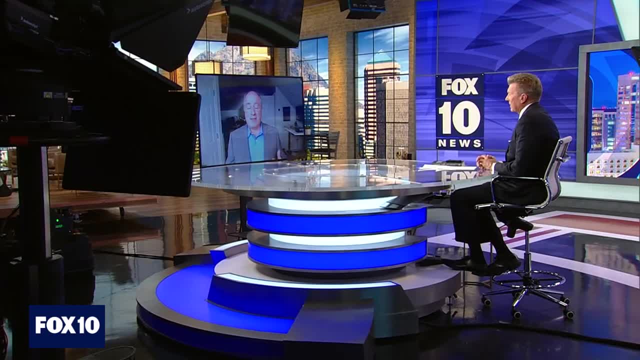 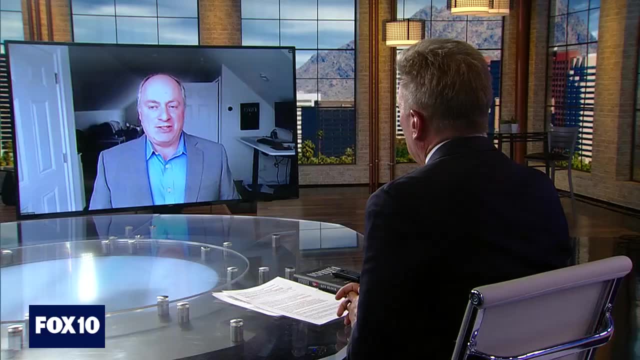 It's also very evident in 2022.. So you can't. I'm a two-time candidate for governor in my ridiculously blue state of Rhode Island And what I know, having run twice, is that you need the biggest coalition of voters behind. 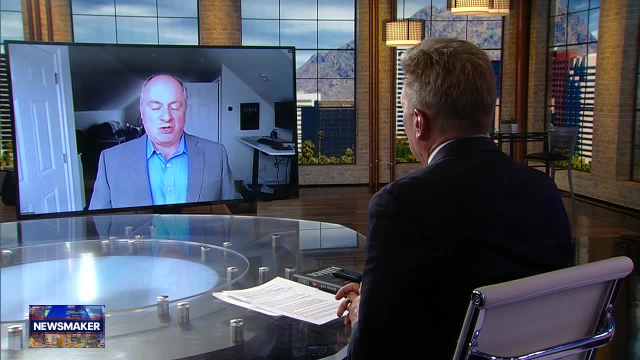 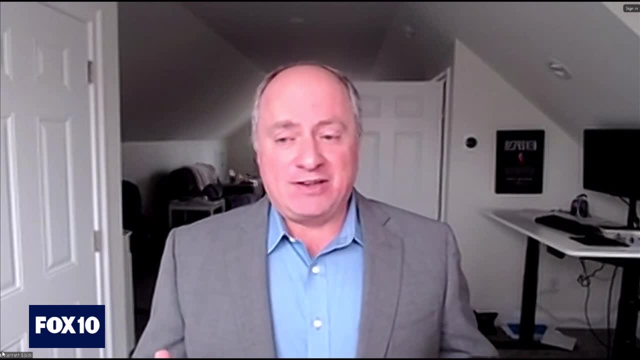 you that you can get to prevail in an election where you need minimally a plurality of votes. you need more votes than the other guy, or you need 50.1 if it's head-to-head And you can't get there. if you're telling a lot of voters you don't want their support. 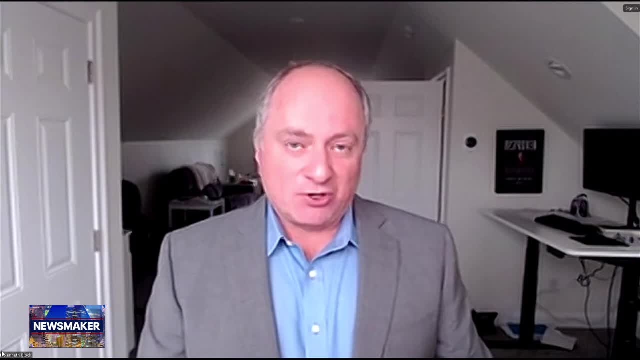 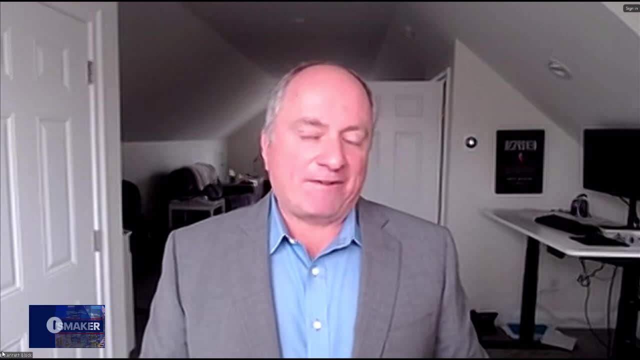 Yeah, it's true, It's always been puzzling to me. This pollster, Tony Fabrizio, who polled my race in 2014,. just to be fully transparent, produced an after-action report for the campaign. The campaign conducted exit polling in the swing states. 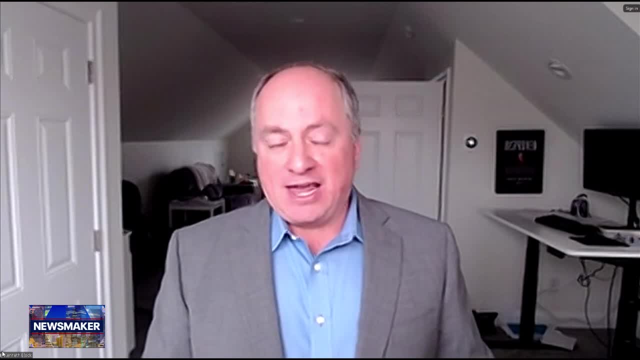 They interviewed 30,000 voters leaving the polling places, And what they learned was that one out of six of those 30,000 voters across the swing states were Republicans who voted against President Trump. There you go, There you go, Ken Block. 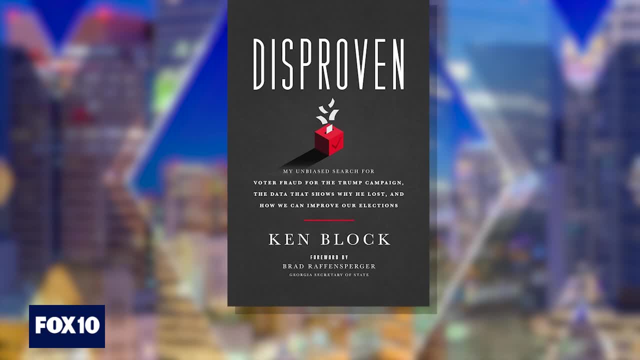 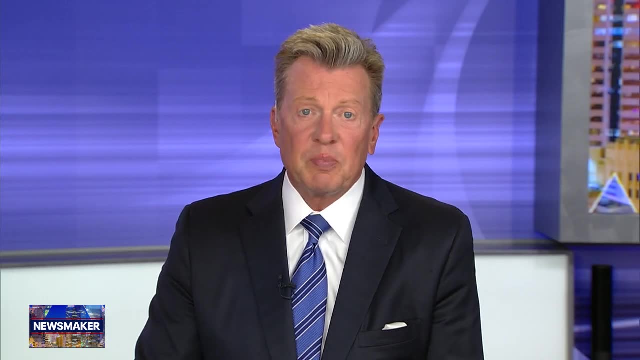 Author of Disproven. Our conversation with Ken is going to continue on the web, Fox10Phoenixcom and on all of our streaming platforms For Newsmaker. we're going to have to say goodnight, Ken, but we will continue this. 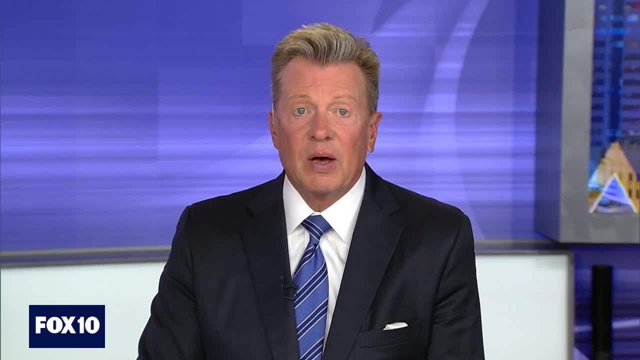 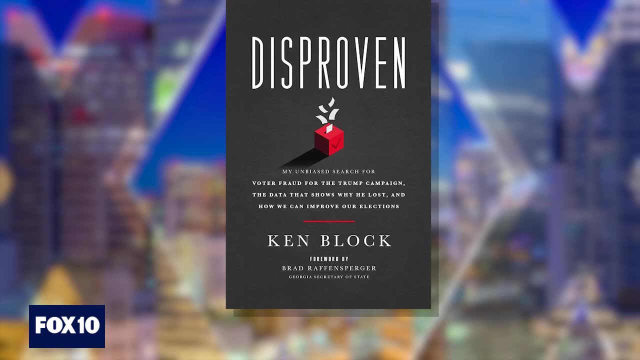 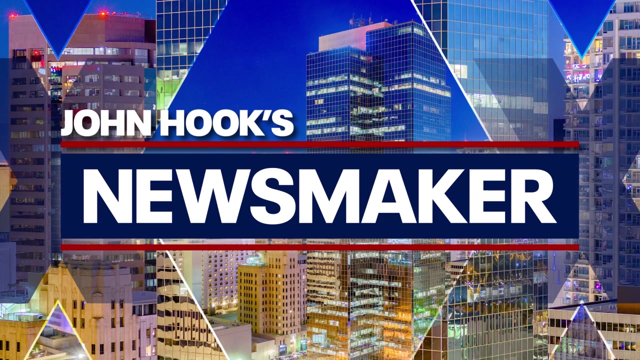 conversation And I hope you all pick it up on the other side on our streaming platforms. Ken Block, author of Disproven my unbiased search for voter fraud for the Trump campaign: We're back in a moment. Thanks for joining us on Newsmaker. 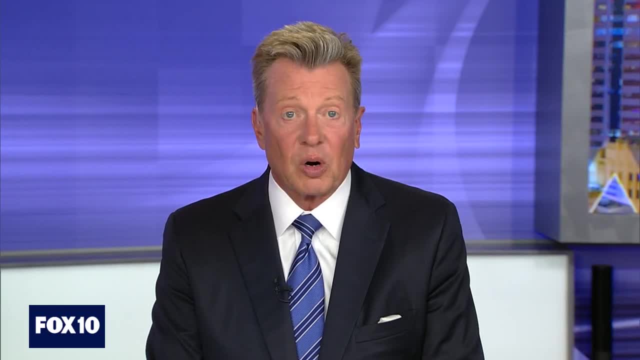 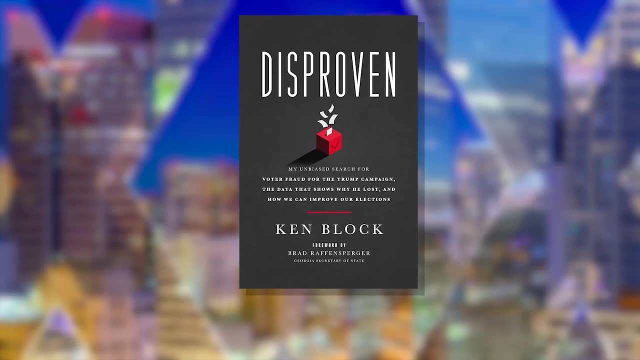 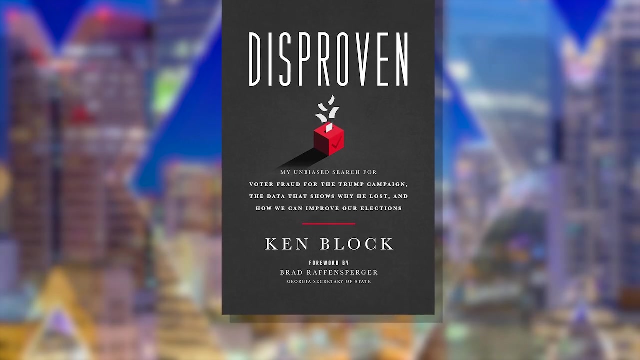 This conversation with Ken Block continues on our streaming platforms and on our website. We'll see you next week. Okay, Back with Ken Block. author of Disproven my unbiased search for voter fraud with the Trump campaign. Okay, Mail-in voting has become. 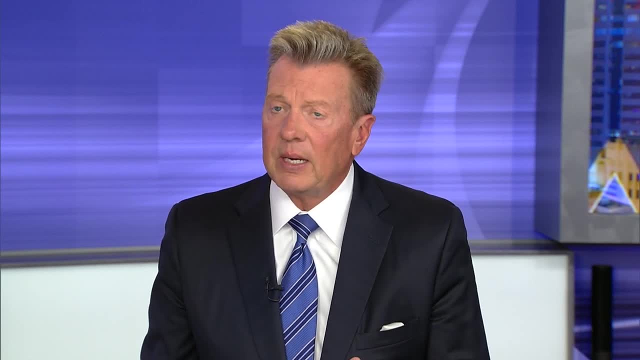 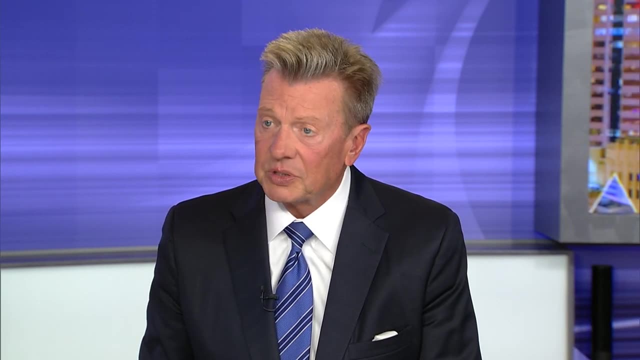 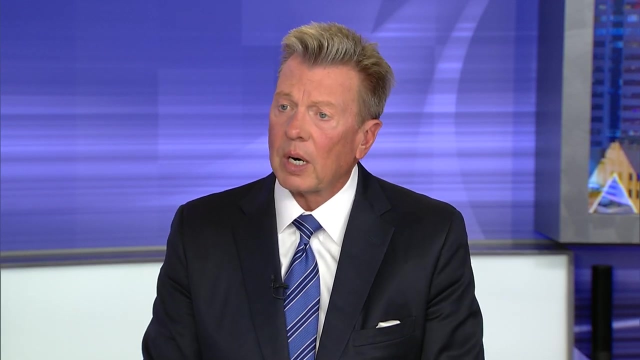 And during COVID it became such a huge deal. Have we sacrificed, potentially, security in our vote for convenience? In other words, whenever you separate a voter from their ballot, do you not open the door to the possibility of mischief? Of course you do. 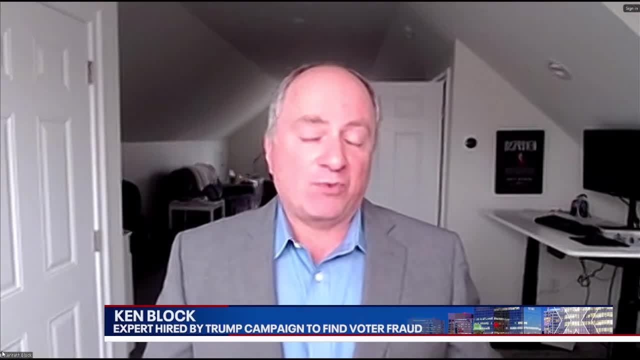 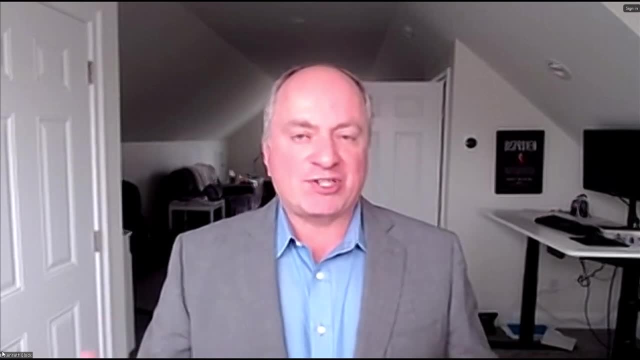 And one of the reforms that I think we really need to consider across the country is coming up with a better, more solid form of voter identification than we have right now, And I know that, reflexively, some more left-leaning people hear the word voter identification and 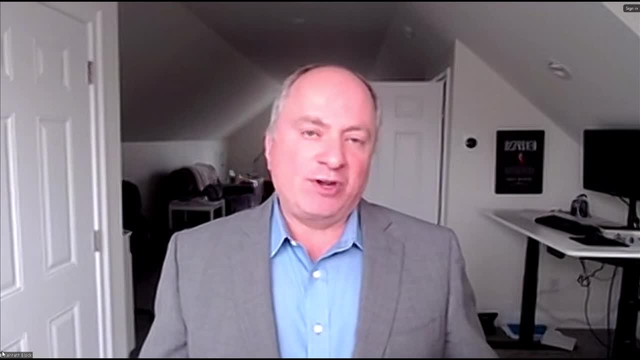 they conflate that with bad. But what we're really dealing with here, especially with mail ballots, is, first of all, the mail ballots are done so amazingly differently by, in some cases, the different counties in the same state, but certainly state to state across the country. 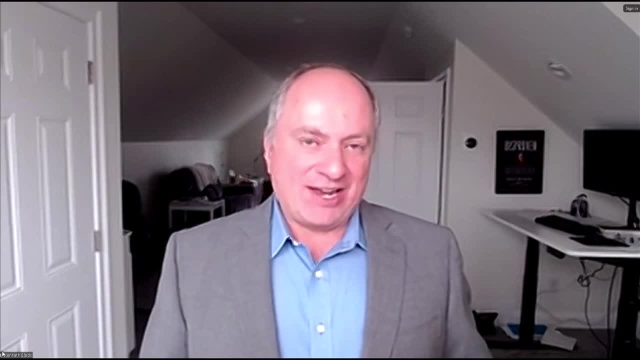 They're done radically differently All over the country, All over the place. We need some standards for how it works And we really should insist on better being able to identify who's responsible for casting the vote and ensure that the person who is going to be voting for. 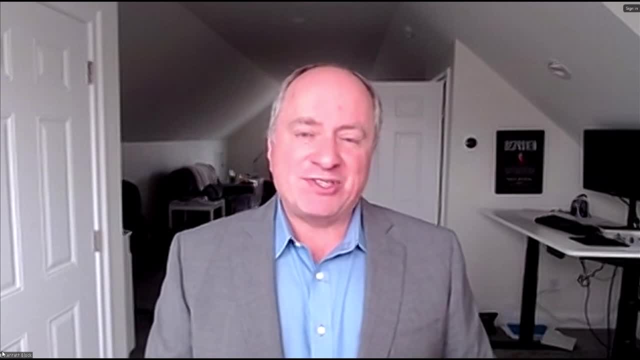 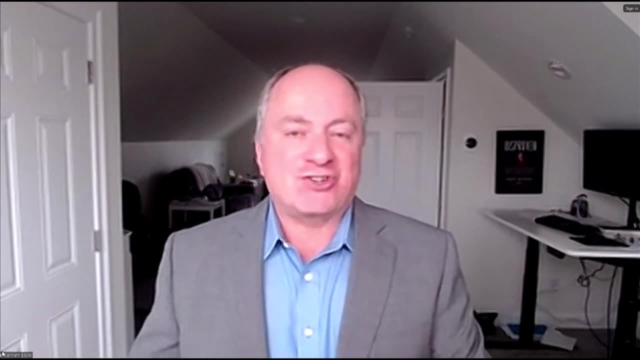 Whose ballot is being voted was voted by that person. It's really a common sense thing And for something as important as choosing- whether we're choosing a president, a governor, a mayor or a dog catcher- it's really important that we know that that vote is happening with. 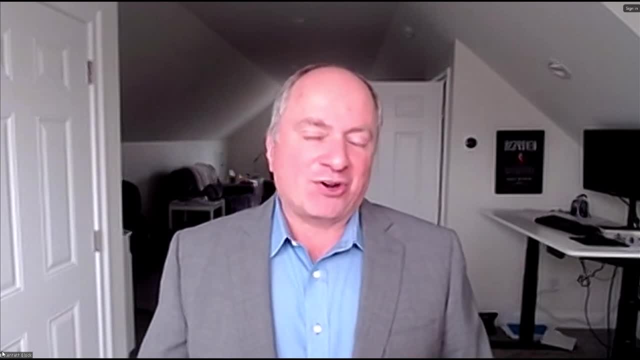 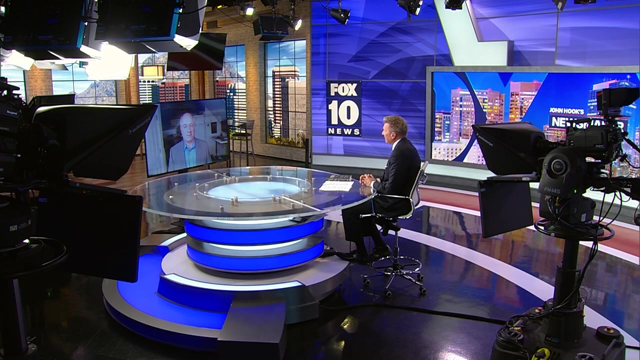 the best integrity that we can get, And the way mail ballots are currently implemented, it leaves a lot to be desired. Now, that doesn't mean that there's rampant fraud, but it certainly means that we can do better than we're doing. You said in the book you called our current voting system deeply flawed. 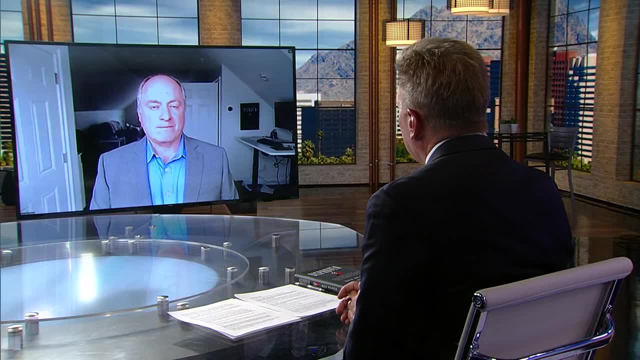 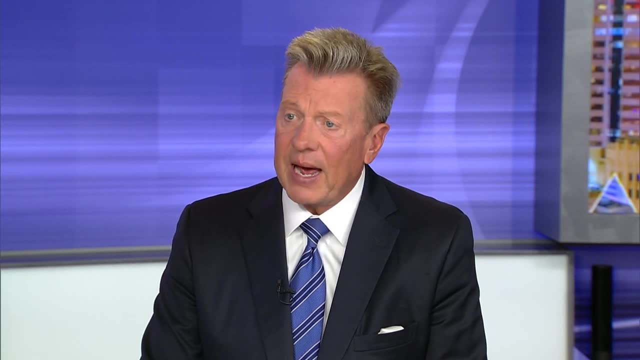 I was surprised that you went there, but you've looked at this carefully And this ID thing is one of the issues. You said, for instance, Yeah Yeah, Yeah, Yeah, Yeah Yeah. You said you had an election standard and you said giving somebody your power bill at 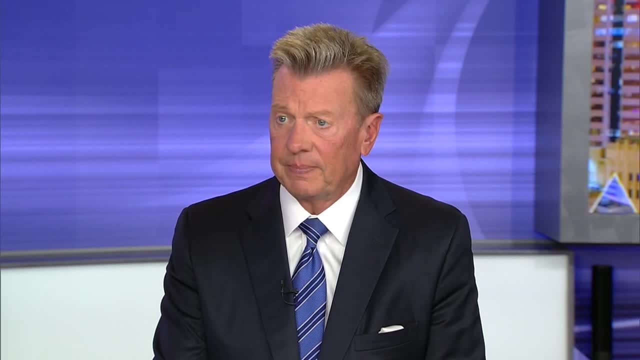 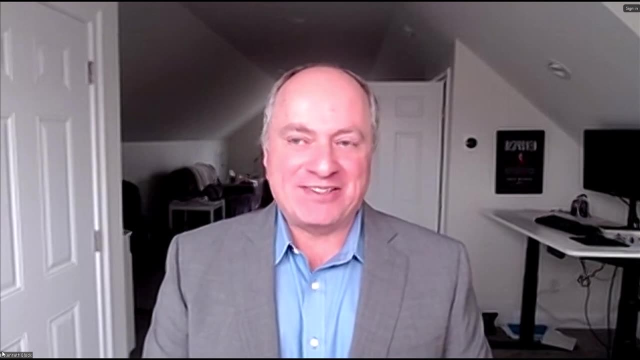 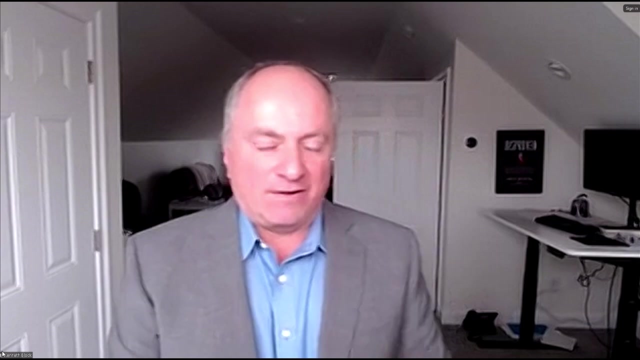 the polling place should not pass for voter ID Correct, So I'll tell a story that will horrify everybody. Back in 2017, as I was exploring with the Rhode Island secretary of state about registration issues and voter ID issues, I suggested that I could send in a voter identification for 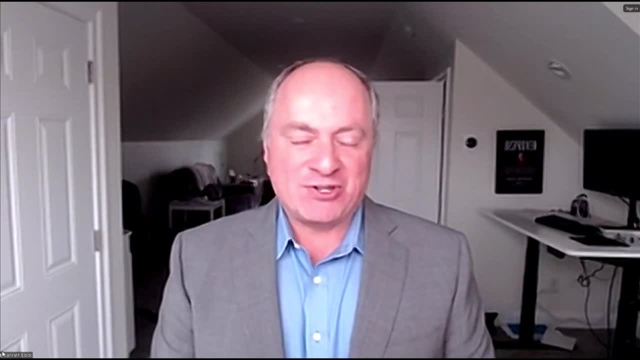 John Jacob Jingleheimer Schmidt registered to vote at my business address And the answer that came back was: yes, you could send that in and we would register that person. I said okay, And then I could walk into the Secretary of State's office with a gym membership for John Jacob Jingleheimer. 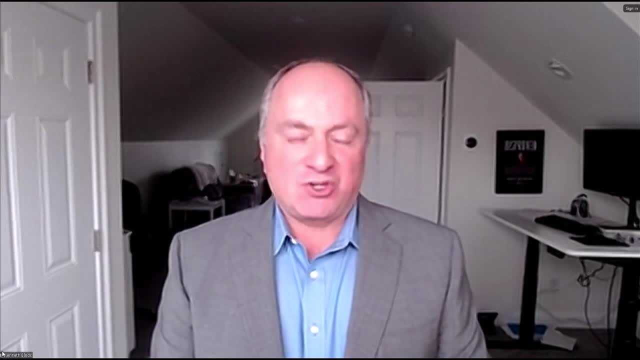 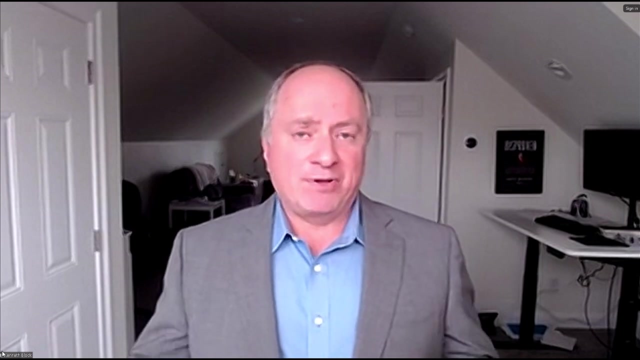 Schmidt and he would get a voter ID card And the answer was yes, you would. Now Rhode Island has voter ID but what you have to submit to get the ID is pretty weak And I found that ridiculous And I thought that was very troubling that someone clearly made up would find its way. 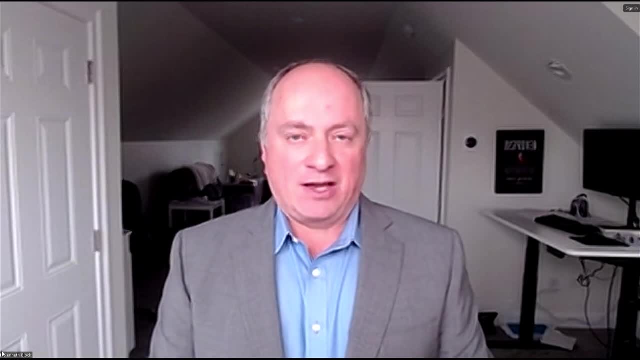 through all the different checks and balances and yield me, ultimately, a valid voter registration. That's only possible because we have fairly weak identification across the board, And I think honestly, if we're going to talk about a solution that solves a bunch of our problems all at once, 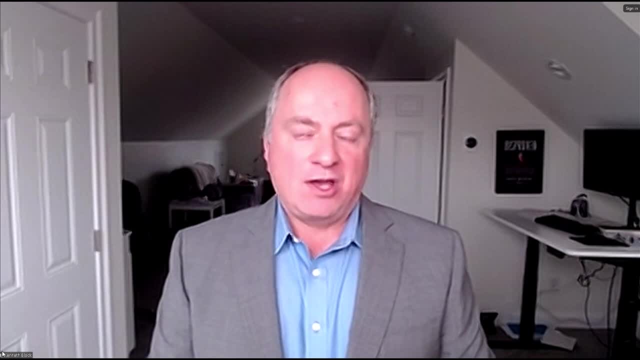 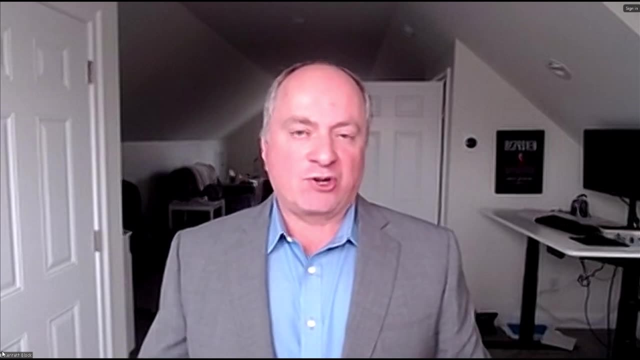 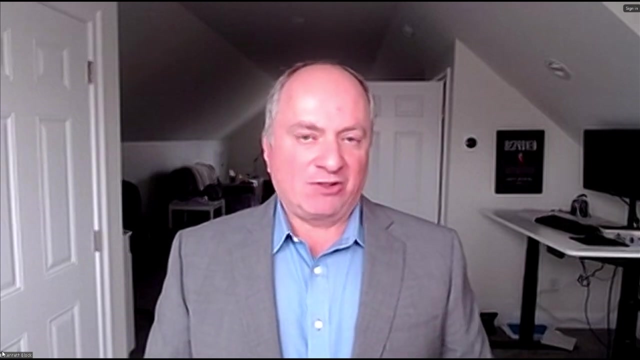 we should take states out of the business. We should have a single national voter registry and we give everyone a voter registration number at birth or at naturalization, And with those two different ways of becoming legally able to vote covered, you then begin to deal with all of the concerns about non-citizens voting. You remove. forever the trouble with people being registered to vote in multiple states and assuming that the federal government should have a single national voter registry and we give everyone a voter registration number at once. And if you're in a state where a state does the best job of any state in terms of removing deceased voters from the rolls and they better you could clean up the rolls, You could have a phenomenally more stable infrastructure on which to conduct our elections. It makes all the sense in the world And honestly, states rights in this case has to take a backseat to enhanced elections integrity. 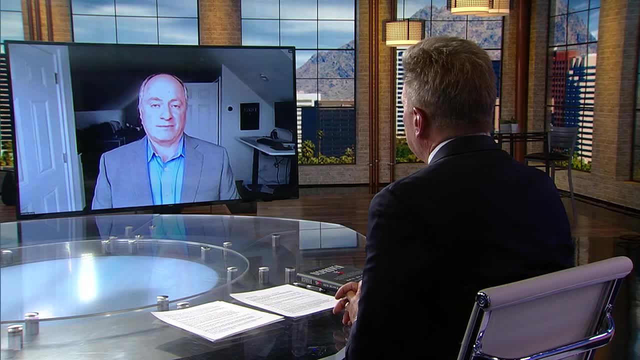 Well, you hit on a big one that everybody worries about in Arizona is that people here illegally are voting. Do you think that's actually a thing? Well, you hit on a big one that everybody worries about in Arizona is that people here illegally are voting. Do you think that's actually a thing? 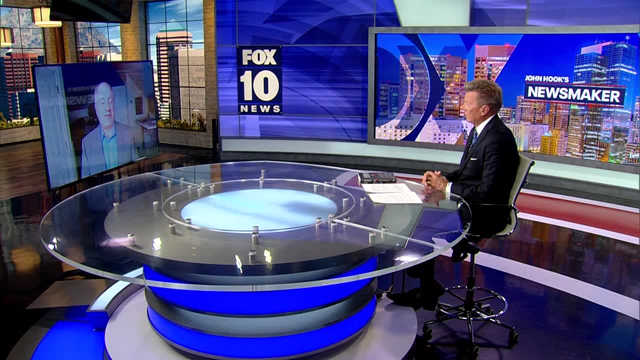 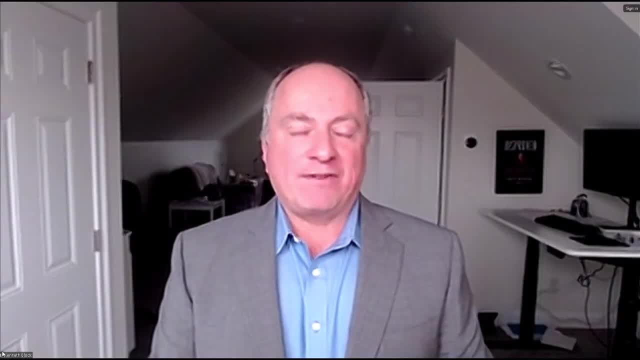 Well, I was asked to look in 2020.. One of the claims of fraud that landed on my desk that involved Arizona was a spreadsheet of 2500. Well, I was asked to look in 2020.. One of the claims of fraud that landed on my desk that involved Arizona was a spreadsheet of 2500. 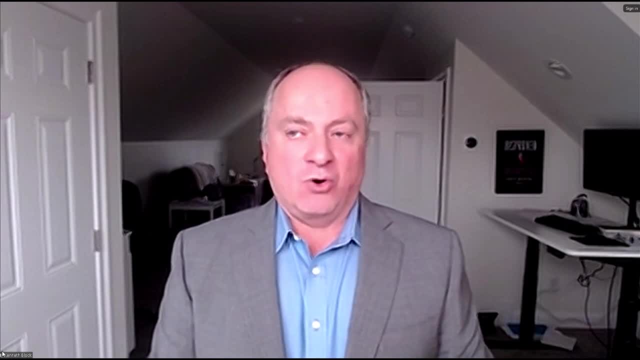 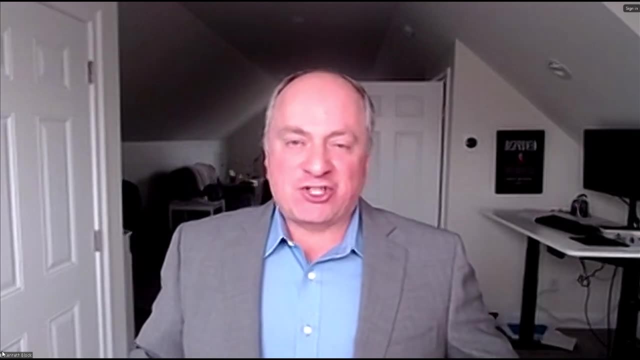 names And I was asked to determine if those were citizens or not. And there was a kind of an amazing ask, because I explored this with Vice And I was asked to determine if those were citizens or not. And there was kind of an amazing ask, because I explored this with Vice. 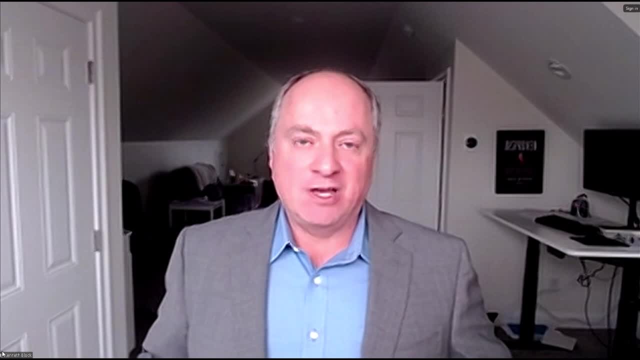 President Pence's staff in twenty seventeen. the asked me if it was possible to have normal elections in that state, and I didn't. These changes look like times have come. Those changes look like times have come determine if registered voters were non-citizens or not. what i told them then was: there isn't any. 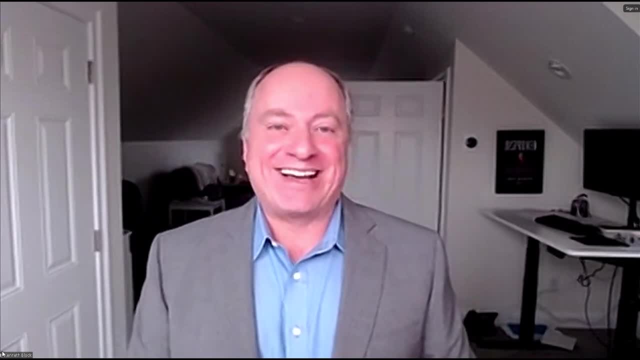 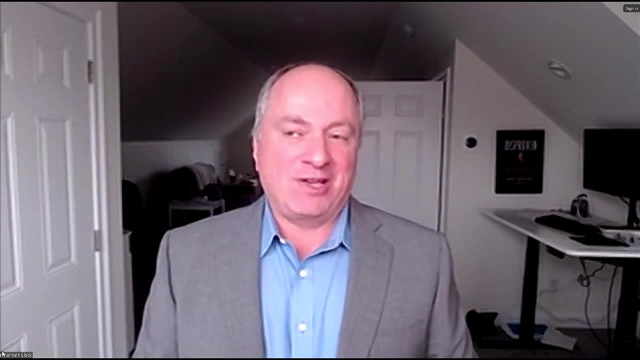 database you can go to that just has a list of everybody who's a non-citizen. uh, and there really isn't a good way to get there. and as alex delivered this one to me, i i told him i said, well, you know, we can try, but there's a lot of, there's a lot of caveats to all of this right and we would use 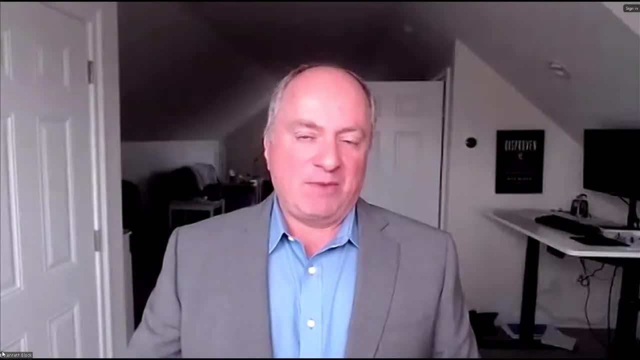 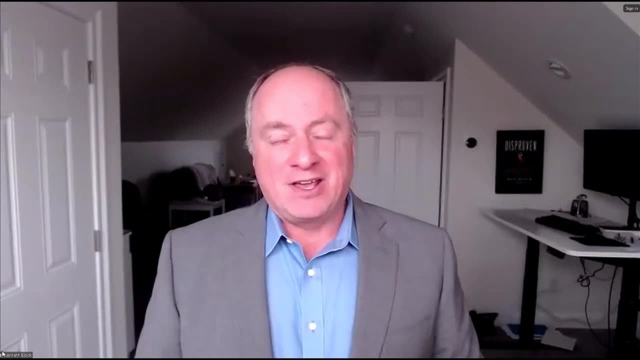 credit bureau data and we would look to see which of the people didn't have social security numbers. and i said: but if we find someone without a social security number doesn't mean they're a non-citizen student. students in the credit bureau databases often don't have any real information in there. 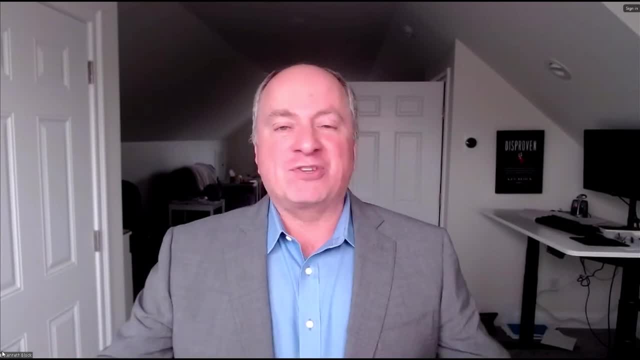 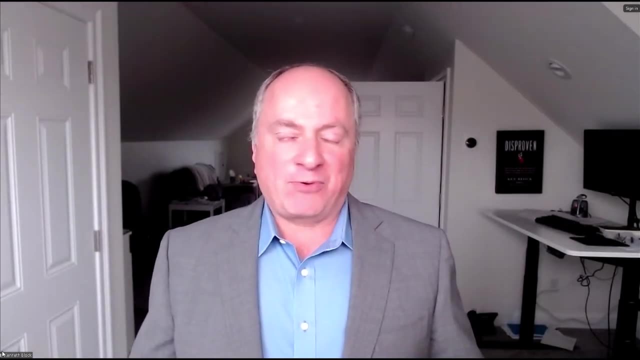 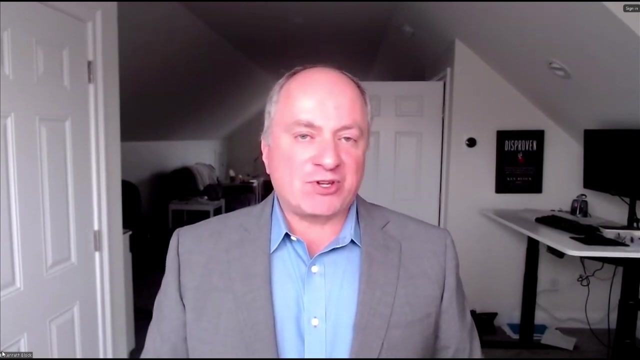 because they don't have credit. and they don't uh, they just aren't visible yet. uh to those businesses. and so we did the analysis, and sure enough, of the maybe three or four hundred uh registered voters that we couldn't find socials for in these different databases, most of them were under the age of 30. 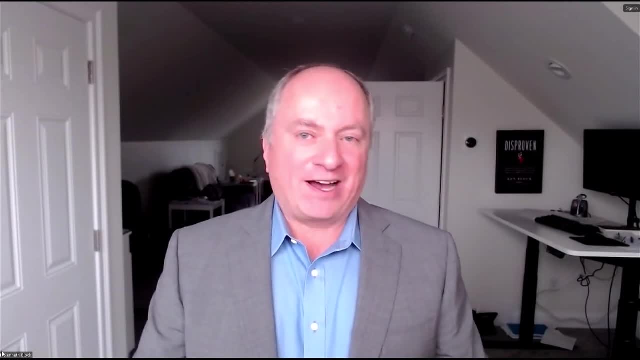 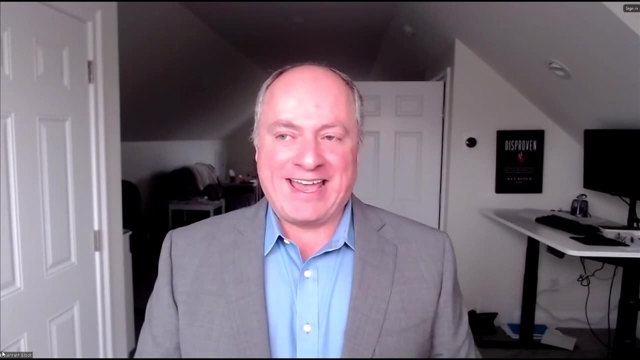 and many of them were under the age of 25, which fits the student profile. okay, uh, and you know the the totality of it was: you can't ever take this to court. uh, and it's not even a smoking gun here. it's every one of these people. if you've knocked on their dinner or you'd probably learn. 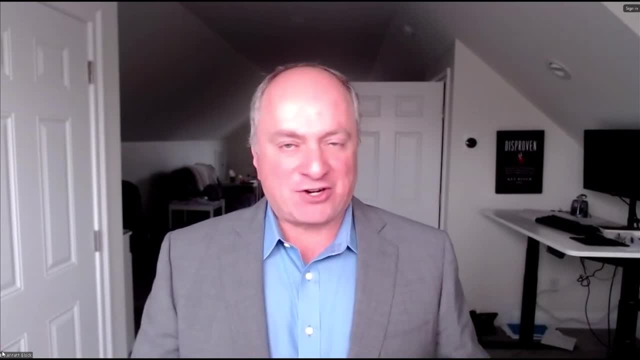 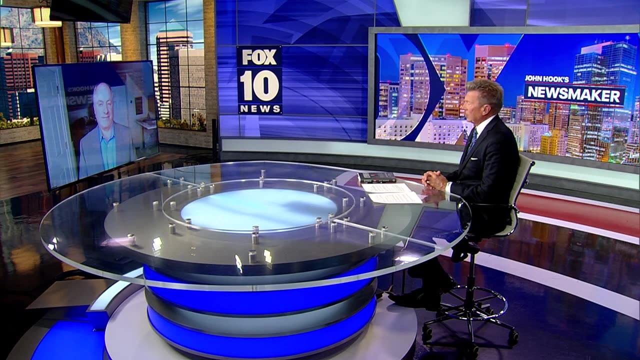 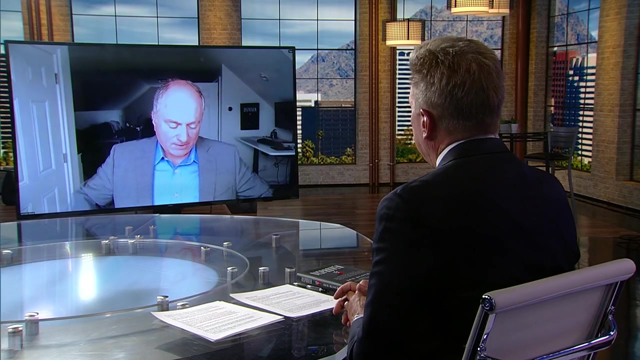 that they just aren't visible to the credit bureaus and they're actually perfectly legitimate citizens and there's nothing here. the other thing that came up during in the wake of the 2020 election was manipulation of voting machines. is that something that people should worry about? well, my work and the claims 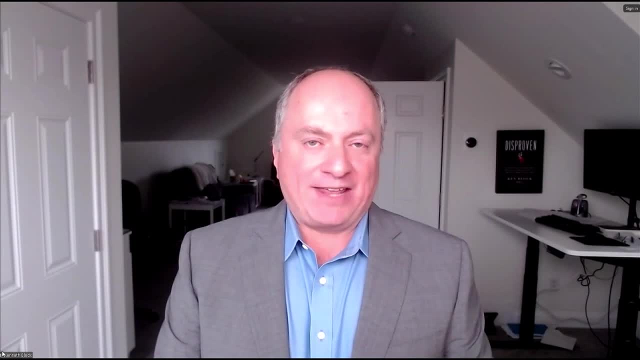 that i assessed were all claims that had at their foundation data. so what i wasn't given was uh rudy giuliani's lies about ruby freeman, for example. right, that wasn't. that wasn't a claim that ever found its way to me, none of the claims about any of the uh election infrastructure. 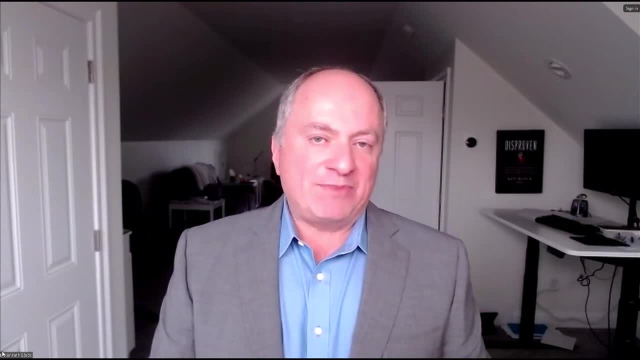 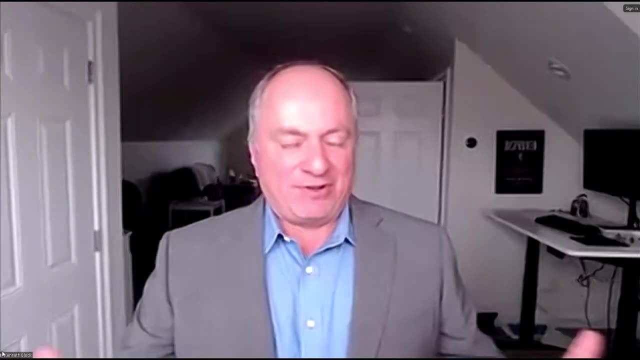 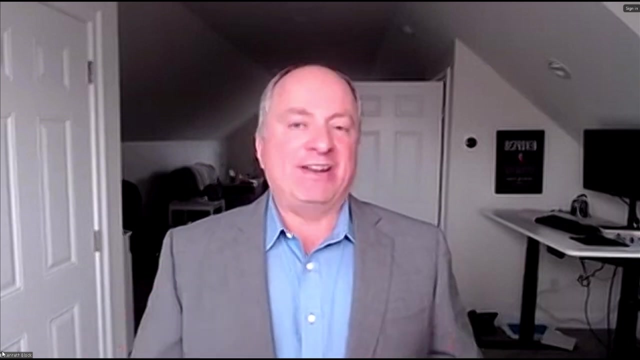 vendors came to me because those claims hadn't really didn't have any data behind them. it was more a hearsay type claim of: well you know, it must have happened this way because of how the results ended up, nobody surfaced actual proof in evidence that could be brought. 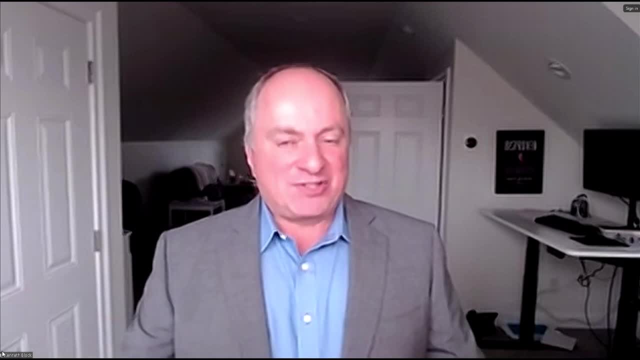 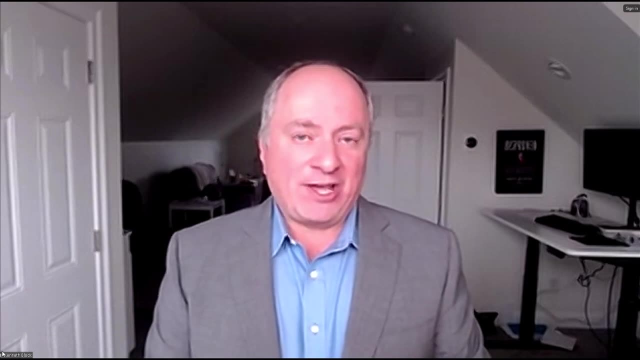 to court and would survive legal scrutiny. that evidence that some of this manipulation actually happen. I think we've seen enough scrutiny of these claims and we've certainly seen the results of legal actions over the claims that I don't think. I don't see how anybody can. 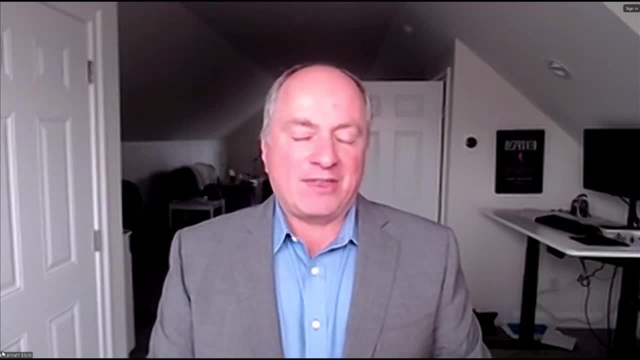 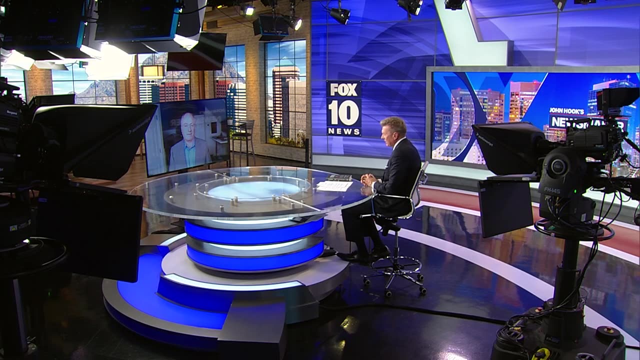 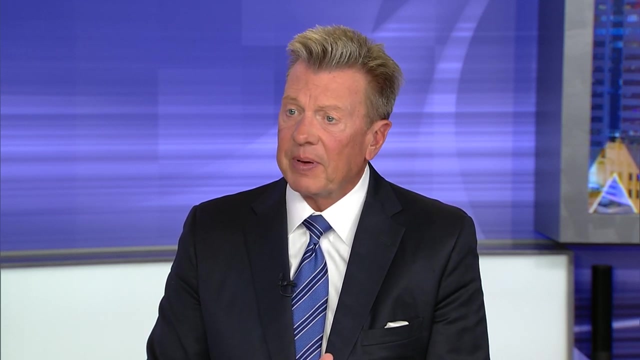 still look at these claims as having any legitimacy to them. They, in my professional opinion, have been thoroughly debunked. Okay, Joe Biden in 2020 earned 81 million votes. That shattered Barack Obama's record of 69.5 million in 08.. You remember that campaign? That was a movement. 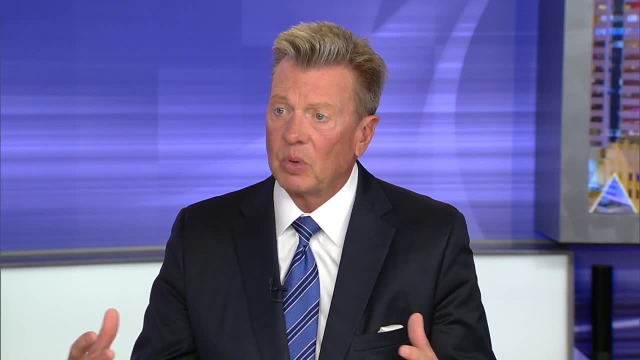 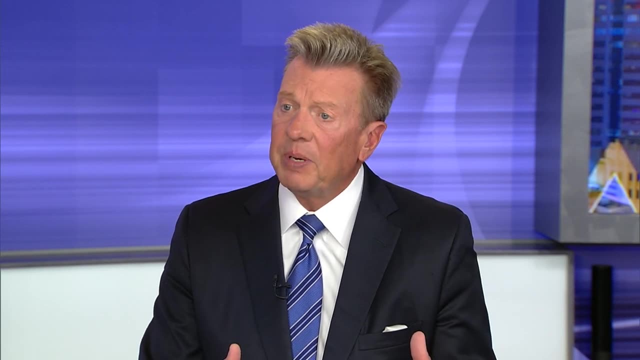 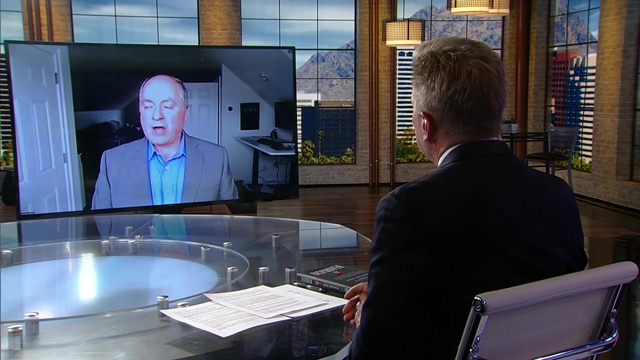 You could feel it. Barack Obama's campaign was an absolute movement. Joe Biden's campaign was largely a basement-run campaign. during COVID, People say: how is it possible he outperformed his predecessor? What would you tell them? Yeah, I'm going to fall back to what President. 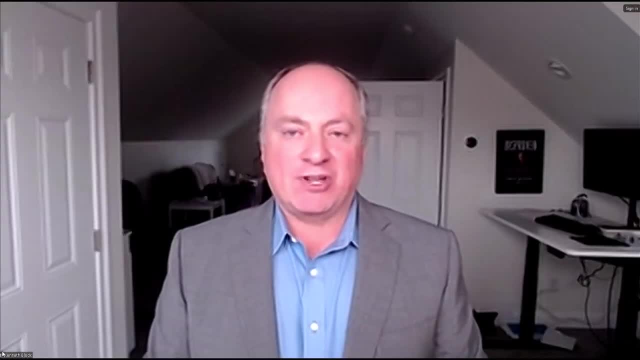 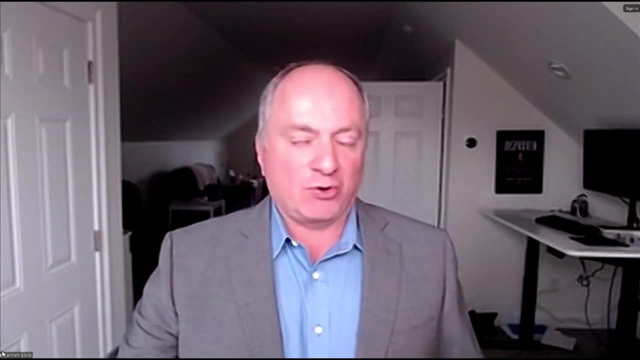 Trump's pollster told him in the after-action report. But I'm also going to go back a little bit in history. In 2016,, the polls had that race completely wrong. The polls showed Hillary Clinton in the lead pretty much right up until the end. 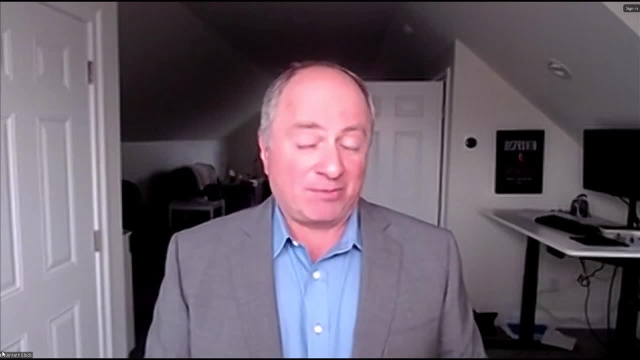 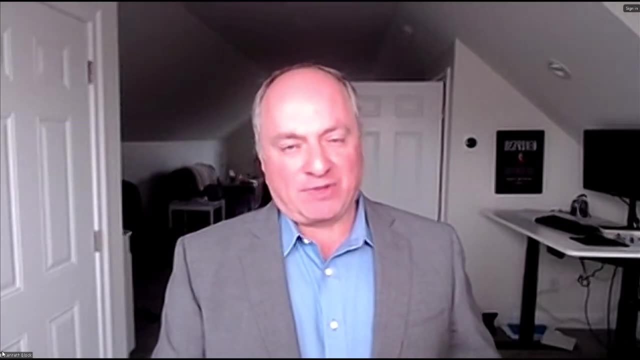 and President Trump's victory in 2016 was not predicted by the polls. The reason for that is unlikely. voters were motivated by President Trump, the candidate, to come out and vote for him, And he won. Michigan, which is a blue state, has been 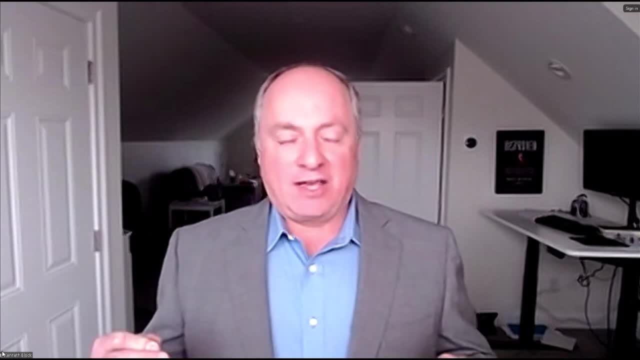 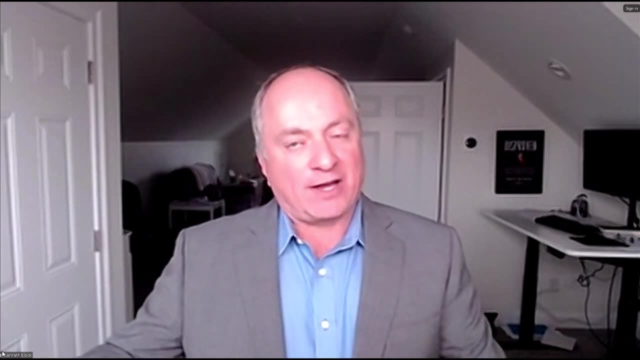 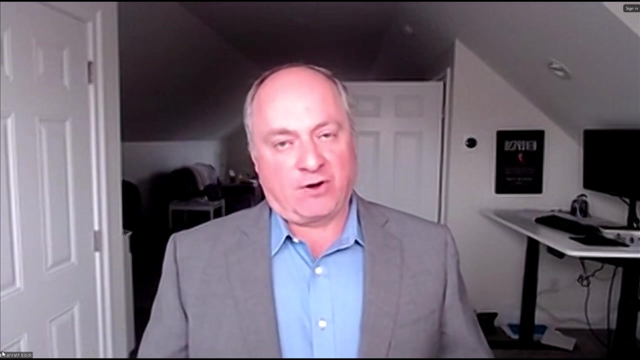 forever, And he managed to squeak out a win there. He motivated first-time voters to come out and vote for him. He had a movement and that movement took him over the finish line. In 2020, the movement worked in reverse: There were enough different voters with different 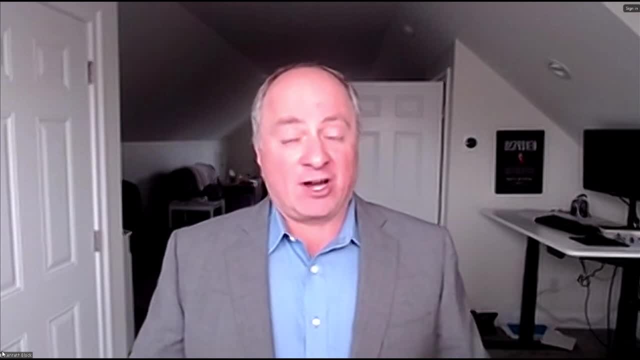 issues that they had with President Trump, and they were motivated to come out and vote against him for a couple of different reasons. One, as we already talked about, one in six were the rhinos. Another one in six was the rhinos. 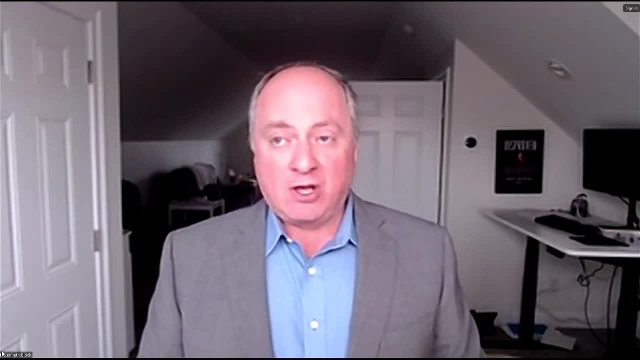 Another one in six were voters- first-time voters- who came out to vote, who weren't happy with the way President Trump conducted the COVID crisis. And that's black and white. Those aren't my words. Those are the words of Trump's pollster, as he wrote them in the 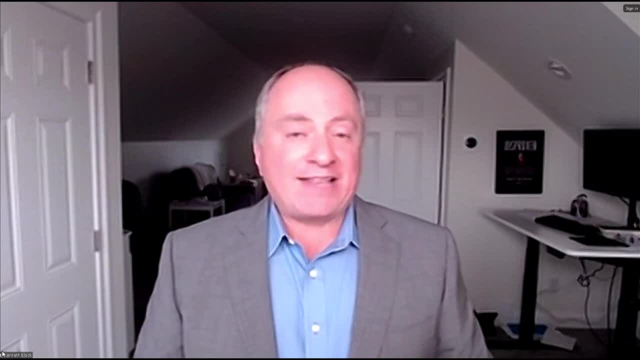 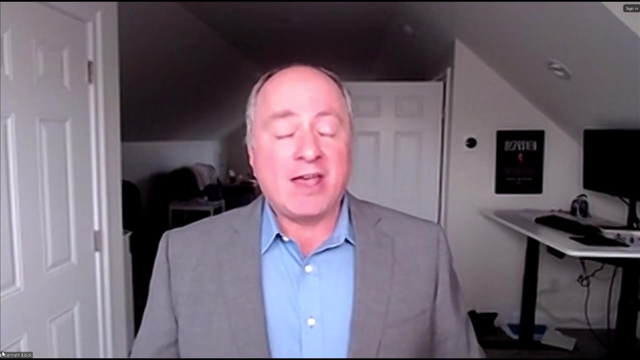 After Action Report. So that's really what happened there, and I don't think there's anything nefarious about it. There were just some undercurrents happening that spoke to people in really powerful ways in both ways- Both 16 and 20, and that's going to happen again. All the polls that we're seeing right. 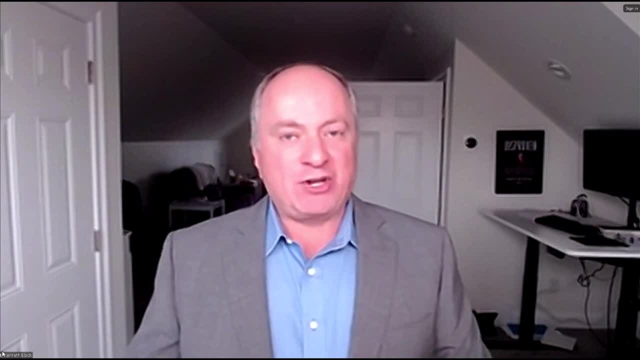 now about what may or what may not happen in 2024 are almost for sure going to be wrong because they're polling likely voters And I believe firmly that this race will come down to unlikely voters and only unlikely voters in the swing states. That is interesting. You mention in the book as well, which I thought we've had a big debate about this in Arizona and other states. How long the voting cycle goes on, You said in the book you think 10 days is a reasonable time for everybody to cast their vote, And if you go longer, you again. it becomes kind. 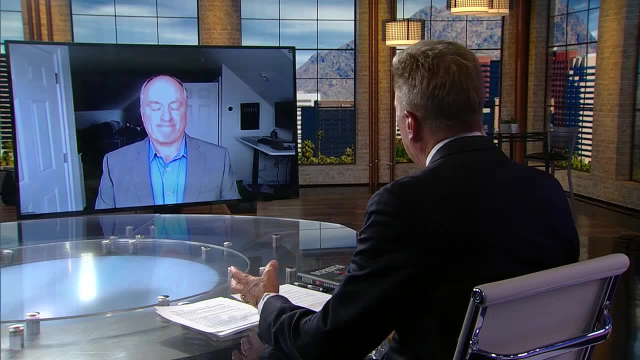 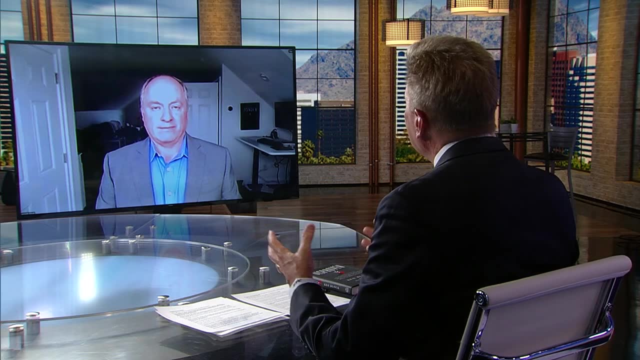 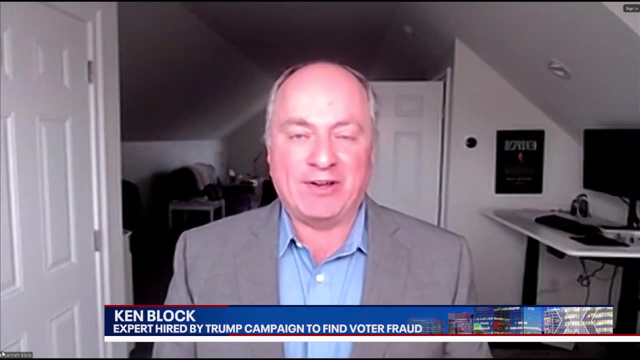 of a ballot harvesting game and a manipulation game And you know it gets away from the campaign messaging and the actual ideas of the campaign. I agree 100 percent. You know they're a state of Rhode Island, It's a 20-day window And that 20 days a couple of bad things can happen inside those. 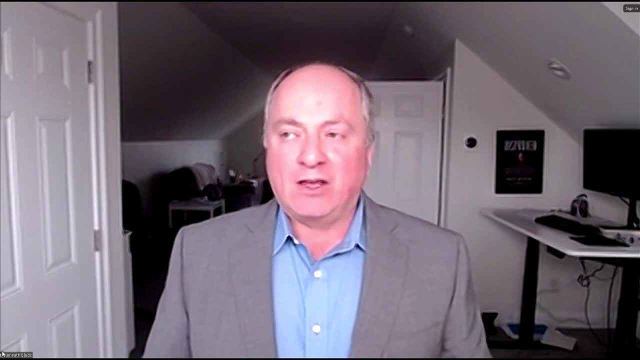 20 days, We had a special congressional election where- and the Democratic- for your viewers who don't really understand Rhode Island- there probably isn't a more Democratic state in terms of percentages in the country, And our elections come down to the Democratic. 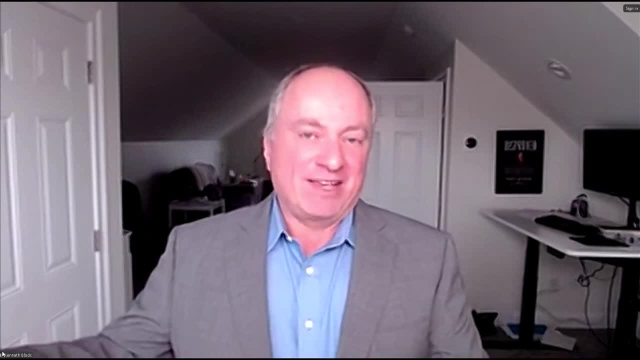 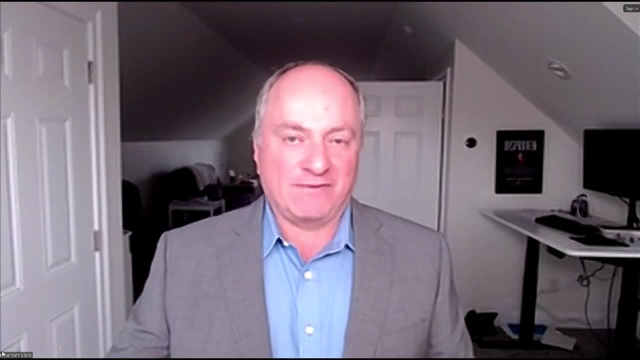 primaries. By and large, whoever wins the Democratic primary is usually the victor in November. Yeah, We had a special election where there was a special election. There were, I think, 10 Democrats running for David Cicilline's congressional seat. 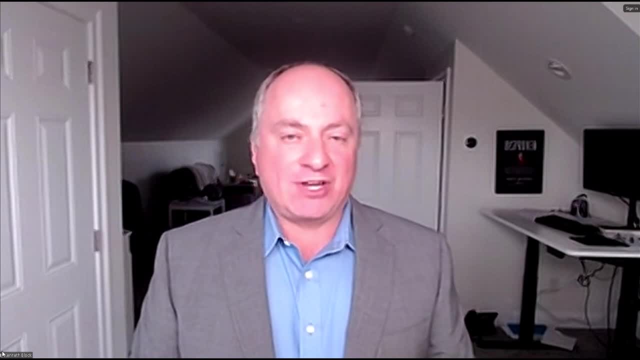 And one of them was pretty well financed. He was funding his own campaign And he had a disqualifying issue come out about 10 days before the election. We had already had early voting for 10 days And it was a disqualifying event. It was so bad. there was no way he 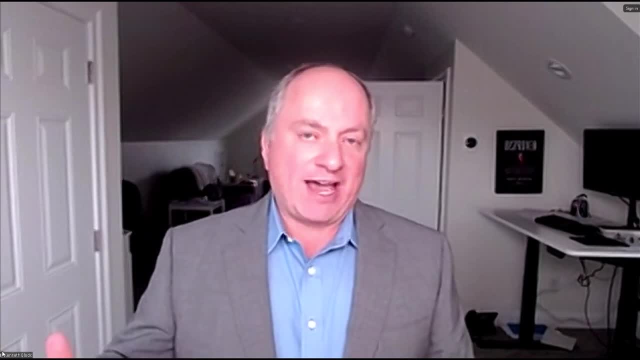 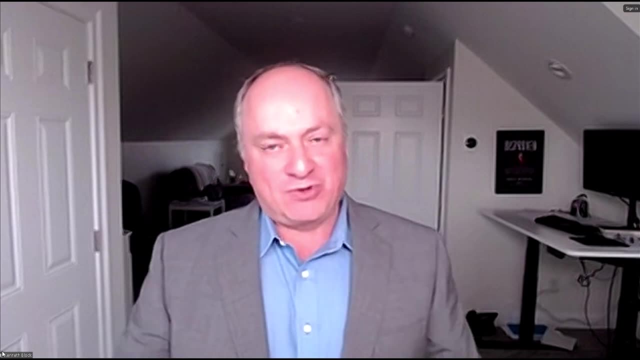 could ever win the election because of this news, But all of the voters who had cast votes for him before that news came out had lost votes, Right, I mean, their votes were wasted. They didn't know this bad news until it was too. 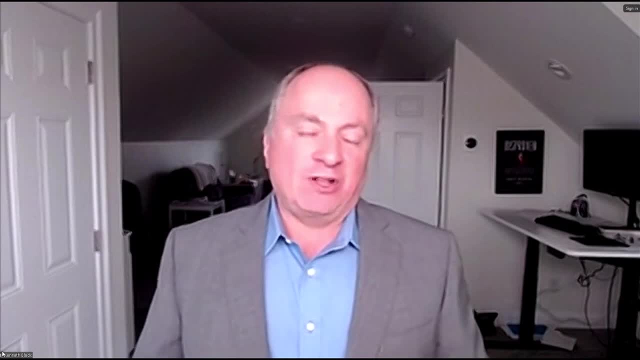 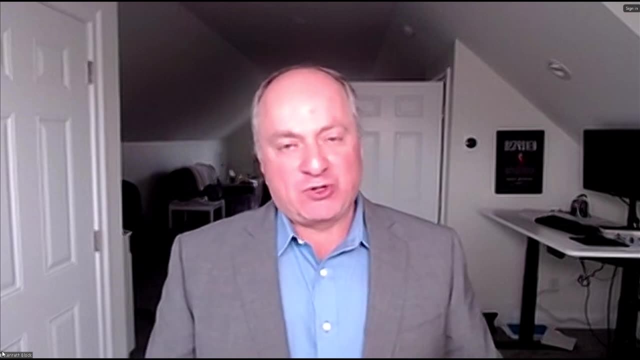 late and they had already cast their vote As a candidate. it's really hard to figure out. when you bring forward your most powerful messaging, You bring it out too early and voters who tune in late don't hear it. If you bring it out too late, your earliest voters 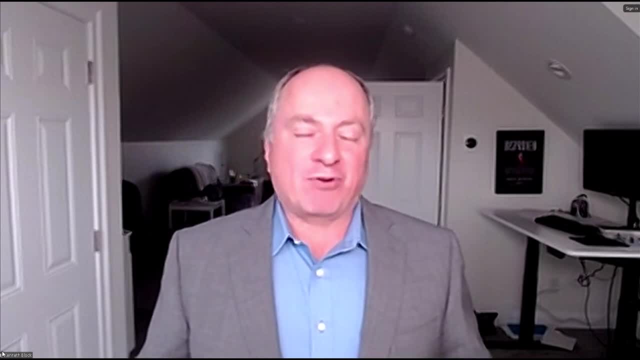 don't hear it. It's really a challenge. And then you have the problem of voting from the grave- And I hope I have a minute to discuss this. Yeah, Yeah, Yeah, Yeah, Yeah, Yeah, Yeah. What you have is a scenario where, let's say, in Rhode Island, you have a 20-day window. 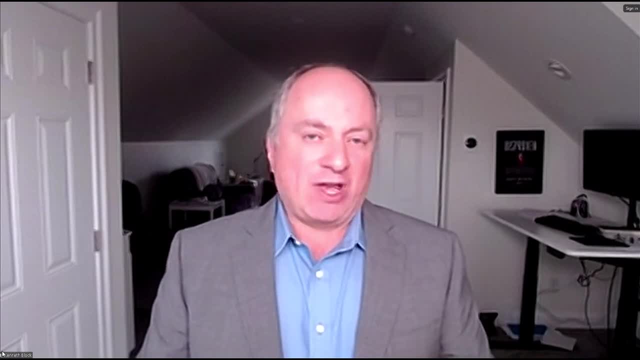 Someone votes 20 days before the election and then passes away before the election. Does the vote count or does the vote not count? Well, in a third of the states it counts by law. In a third of the states it doesn't count by law. And in the other third of the states, there's no law for this scenario at all. So in Michigan in 2020, 35% of the voters were canceled because of early voting, where the voter died before the election. That's not a small number of votes that have been canceled. No, it's not. And the longer the window is, the more voters are going to fall into this unfortunate set of circumstances And in states that allow the vote. I mean, what if you have a six-month window? At what point is it too much? Yeah, And I think, because of everything I just described as problems, that we want to provide voters a meaningful window that solves most problems that a voter can have, And I think 10 days covers that You're going to have a weekend, You're going to have a full week plus a few. 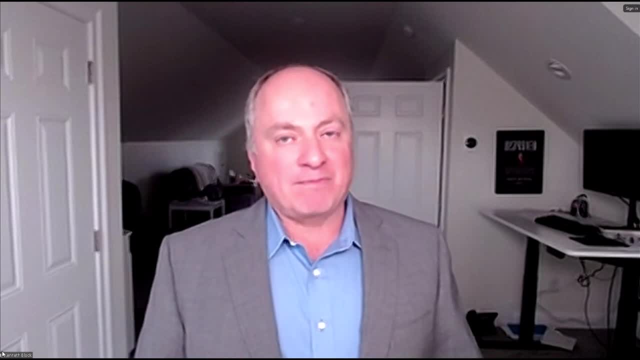 days on top of it. That should solve almost everybody's problem, except for, potentially, mail ballots, because we know that the mail service can be unpredictable. Maybe we need a few more days for mail ballots to ensure that any difficulties we have with the US mail. 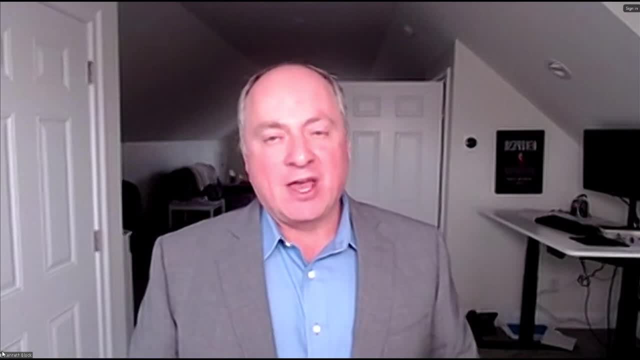 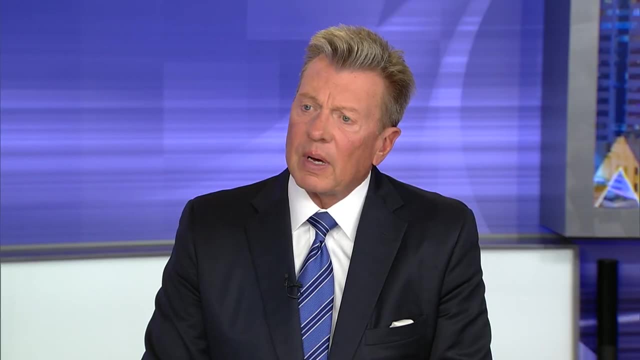 service aren't a cause of disenfranchisement for any voters. I think it's really important to keep a lid on how wide these windows are. Yeah, I agree with that, Do you? I'm curious: do you find a distinction between, say a: 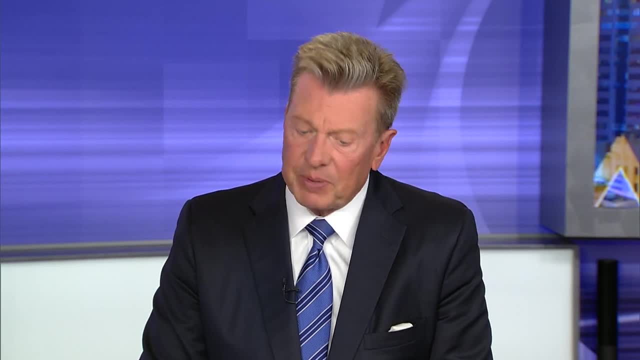 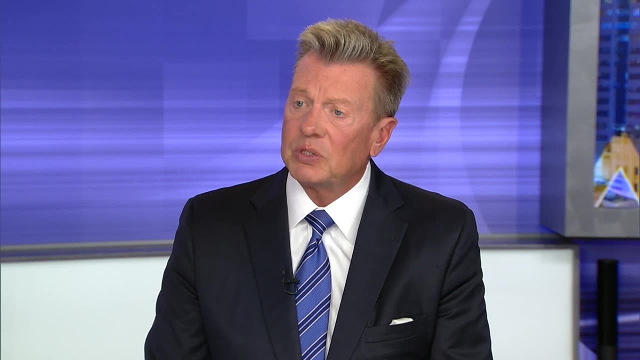 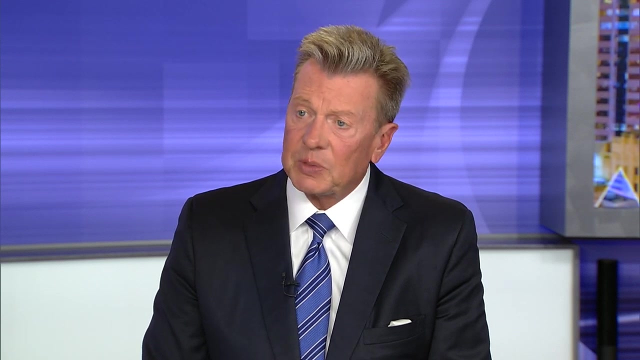 stolen election, where data is actually manipulated, versus a fair election, And what I'm getting at here is the lead up to the 2020 election. President Trump had his headwinds. You had legacy media spiking, the Hunter Biden laptop story. You had the 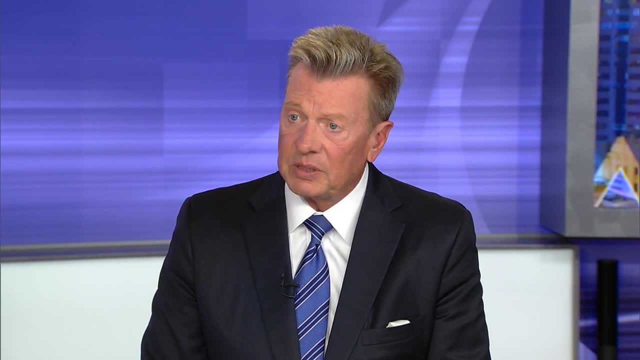 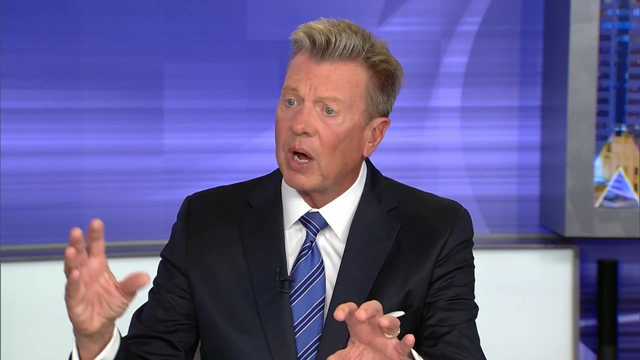 Russia collusion thing still bubbling. that dogged him his entire three years. You had silencing of conservative voices on social media. You can have technically a fair election, but is it fair when that stuff is going on in the background? Yeah, that's a really good question And 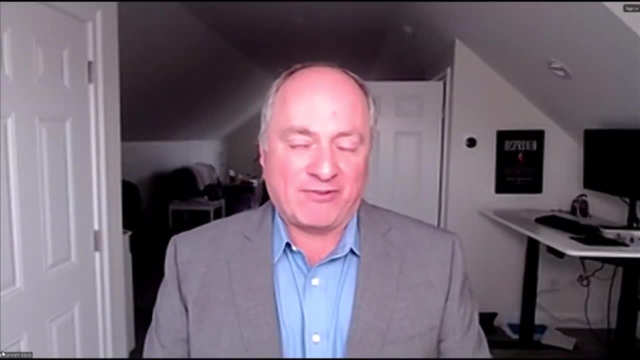 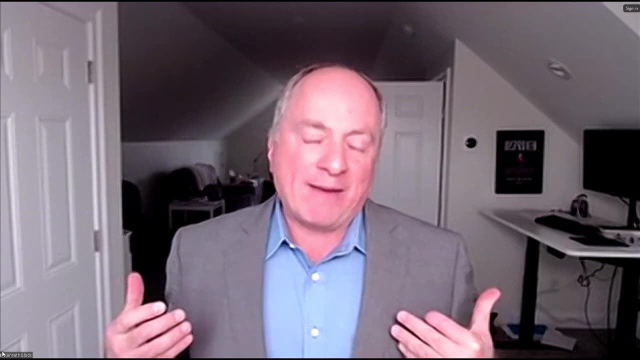 I am going to clearly struggle in how to provide you a meaningful answer. I think it's really hard to tease that all out and address them in the way that I'm trying to talk about everything regarding my involvement with the election. I'm trying to keep it all. 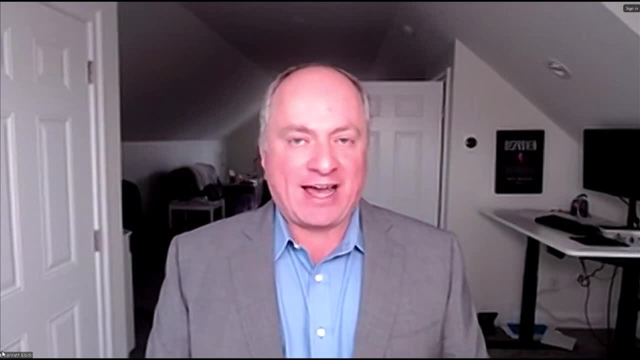 100 percent strictly factual on the things that I had done. And data-driven. I understand that. And data-driven: What I'll say is that it's been generally difficult for me to talk about everything that I've done. I've been talking about the front part of my book. with conservative media. They often don't want to. 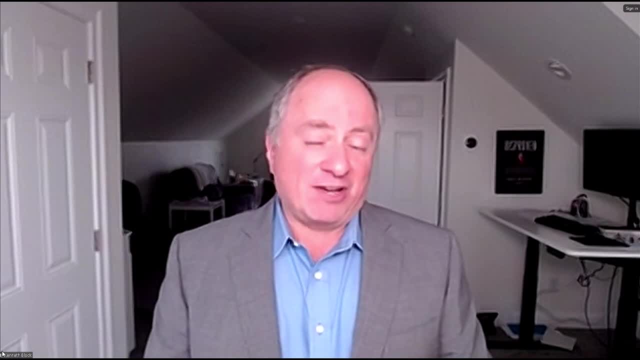 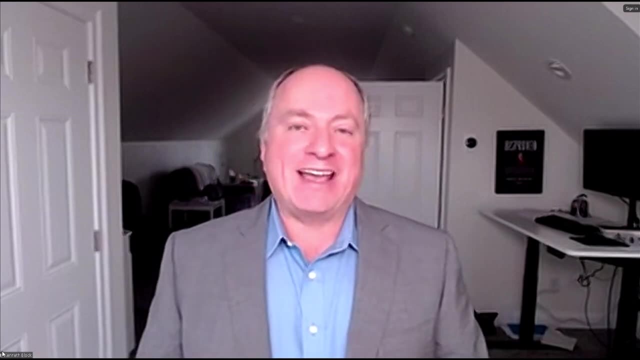 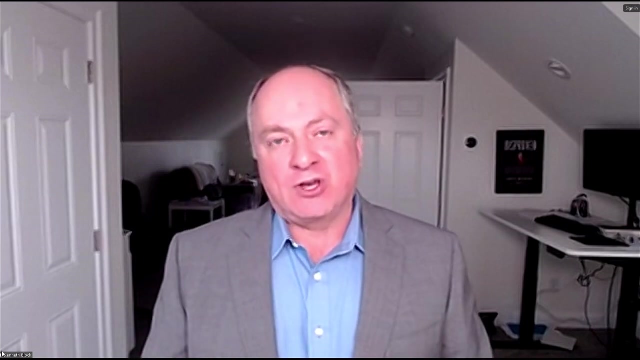 have the conversation And I've had a difficult time talking about the reforms that we should make to our election systems with liberal media. They're not all that interested in entertaining the idea that our elections can be better than they are right now, So I'm not sure how many actual votes were swung by some of the issues that you raised to me. 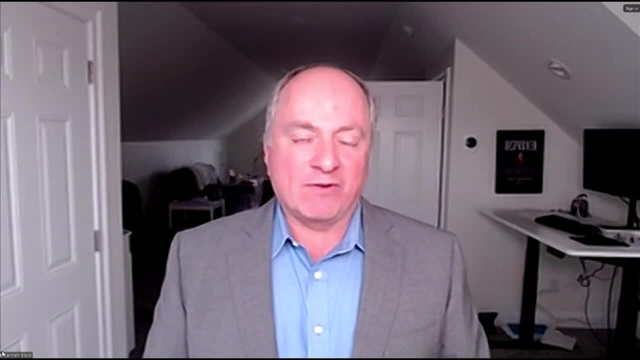 Uh, I think that by the time we were were voting, it would shock me that there were very, very many voters who hadn't already made a determination in their minds on which way they were going to vote. I don't think there were very many people walking into the voter booth going I don't know who I'm going to vote for. 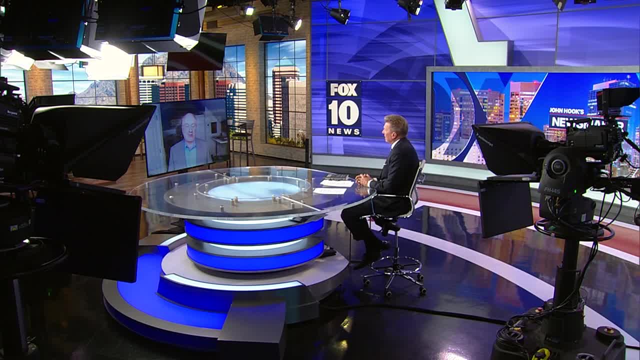 Yeah, That's a great point. I don't. I don't know for sure And it's really, it's really hard. It's a very squishy area to talk about. Uh, I think that in general, you know, there's there's a lot of unfounded. 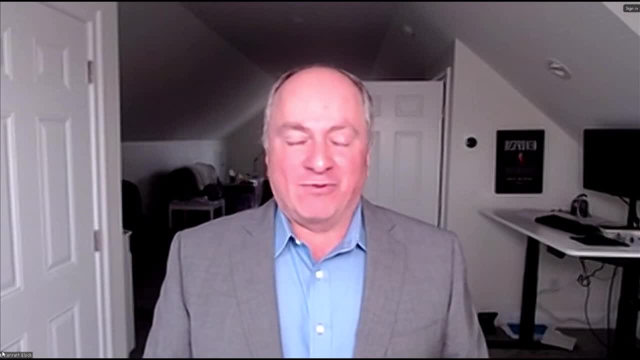 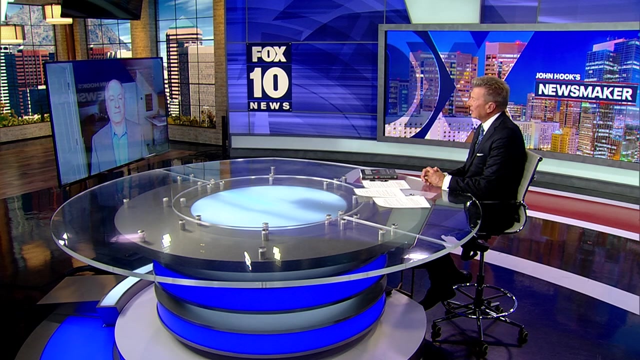 information swirling all around us, Uh, and the most important skill we can teach our kids is how to identify it and make sure it doesn't unnecessarily- uh, swing you in a way you don't want to be swung. Ken, if somebody comes up to you now on an airplane, if they know who you are and they say: 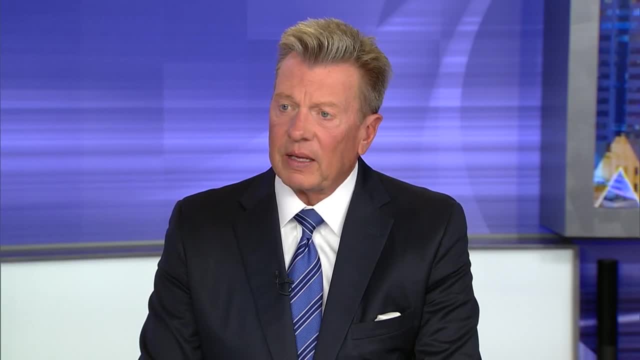 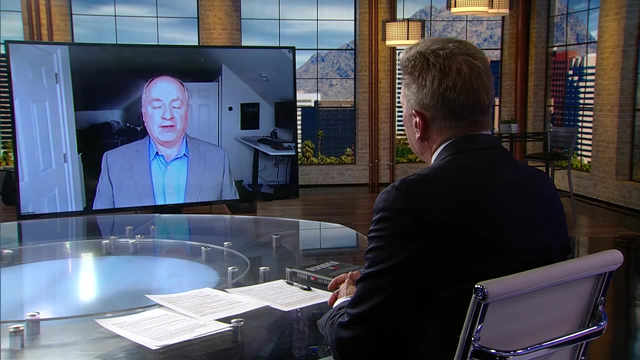 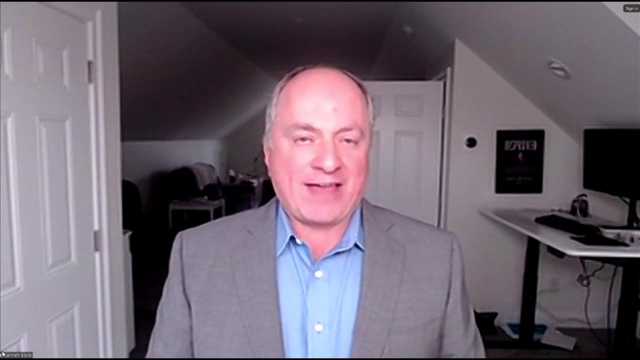 listen, I know what you wrote, but I believe that election in 2020 was stolen. What would you tell them? Yeah, Uh. what I would tell them is, from a legal and fact-based perspective, not only was it not there in the window in which it could be contested, it to this day isn't there. 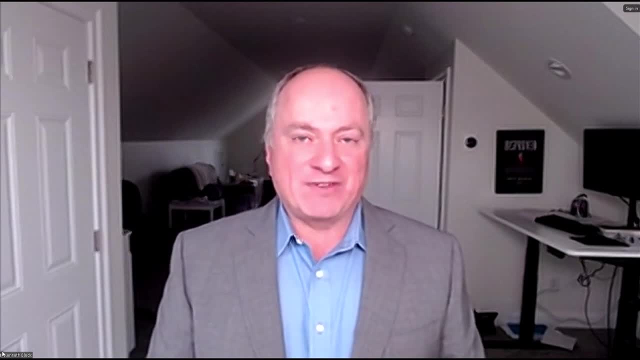 I am not a disinterested observer of the different claims of voter fraud, the different legal actions that are happening- uh, still all over the country about 2020.. Uh, and nobody has surfaced a complaint that has the legal legs. it needs to matter. Uh, it's just the the the evidence. 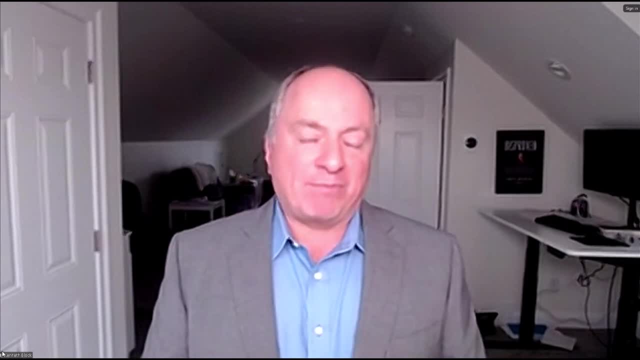 isn't simply. it just simply isn't there. Now we're talking about the election in 2020.. We're talking about political messaging, and the political messaging has been phenomenally effective. The election was stolen, The election was stolen, The election was stolen. We don't. 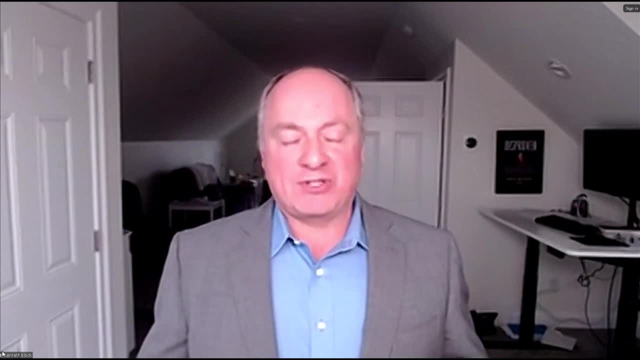 have the evidence. but just look at the number of votes, Look at the, the what's staring you in the face? Uh, it couldn't have been anything else And I get how that's an emotional argument, but it's not a successful legal argument And it's not a successful argument that can change. 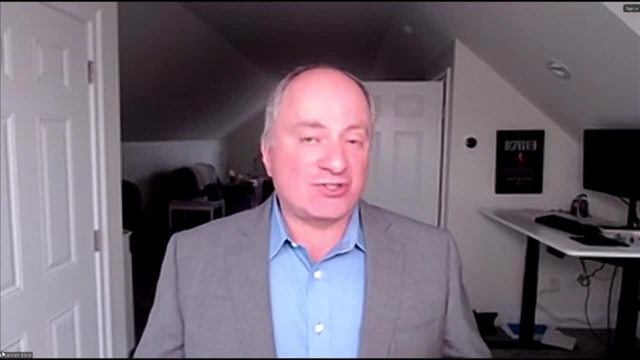 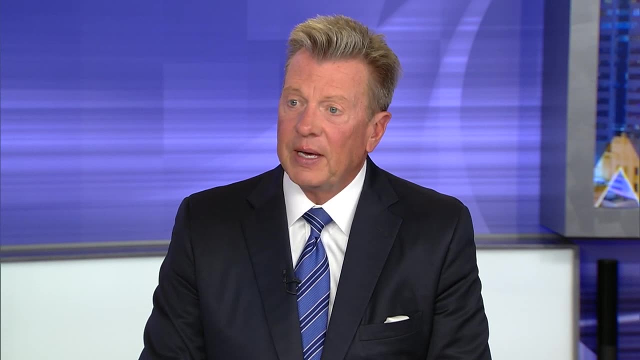 what has happened? Uh, And that's just the truth of the matter. This hearkens back to Rudy Giuliani's famous comment where he said: we know voter fraud happened, We just can't prove it. Well, in the end, that's where the rubber meets the road. 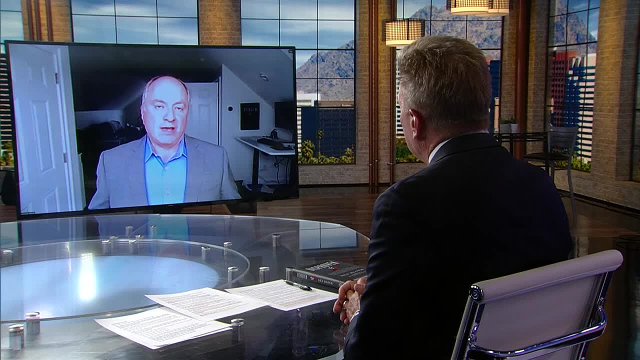 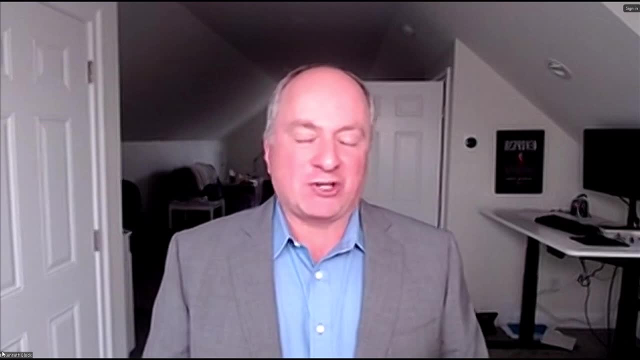 It, it has to meet the road and you need experts like me If you're going to go to court. you can't go to court with somebody who's delivering you a custom ordered set of results, because the other side's experts are gonna blow you up. 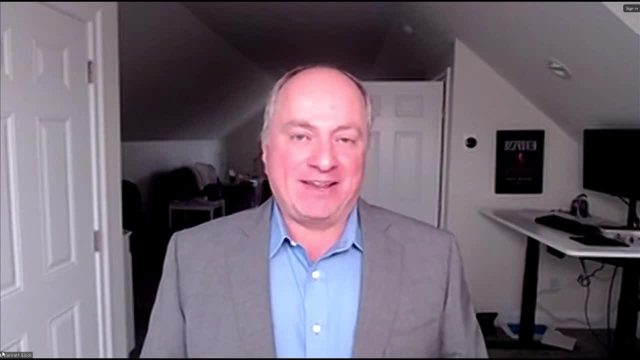 and it's going to go badly. You have to find it, It has to be done carefully, It has to be real And if all those things are there, you have an ability to make a strong case. I can't tell you: you're going to win. because you still have to show harm, as we discussed earlier, and I don't see how you can do that. But to bring a credible case, it's possible to credibly identify enough voter fraud to impact the to be bigger than the margin of victory. It's possible. It hasn't happened, but it's possible. But it's not possible the way most of the voter fraud narratives are being pushed out there and the very shaky evidence on which every single one of them rely. It isn't the sexiest topic. 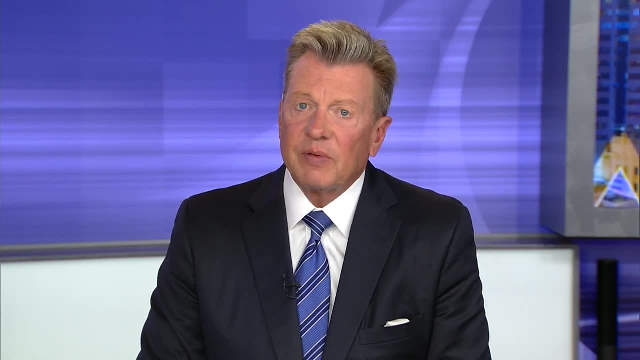 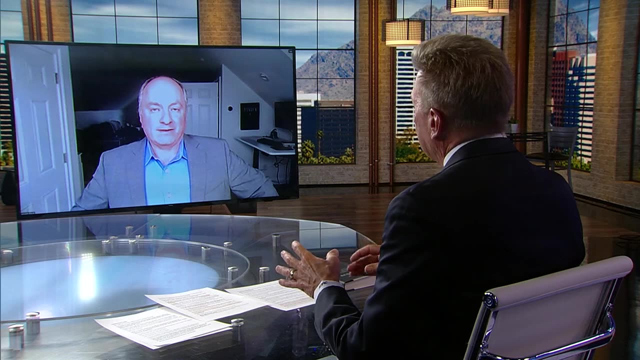 but I have to ask you about it because you talk about it in the book. You take a very dim view of ballot harvesting. Explain what ballot harvesting is and how you think it's anathema to a really clean election. Yeah, Yeah. 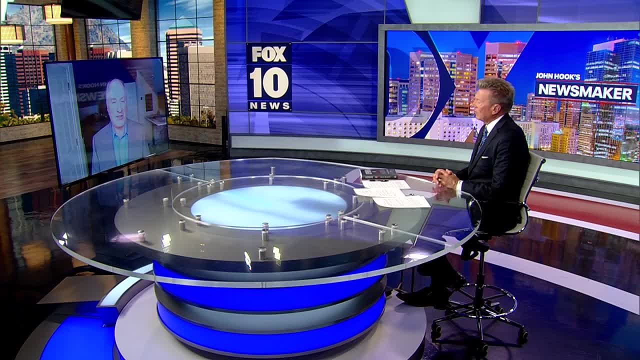 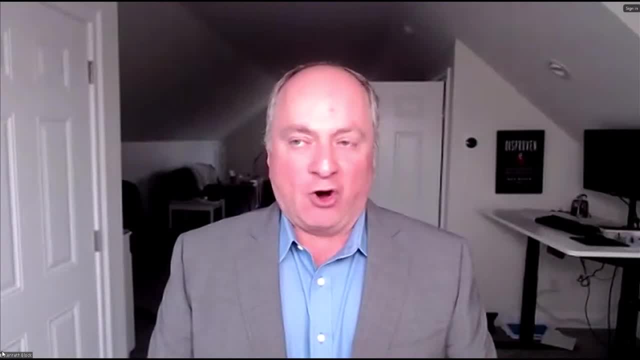 So- and I'm going to come back to my Rhode Island direct experience as a candidate- In Rhode Island, ballot harvesting is legal And the openly discussed truism about Rhode Island politics is: if you're going to win your race, you've got to play the ballot harvesting game. 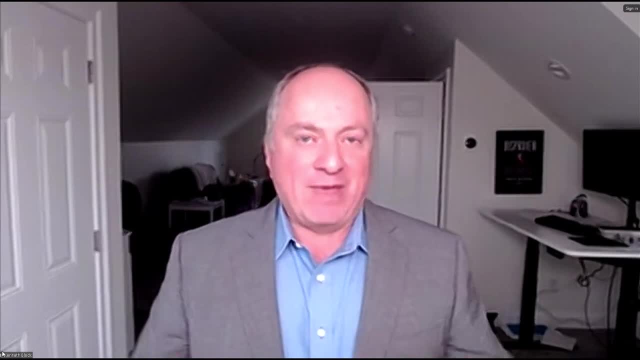 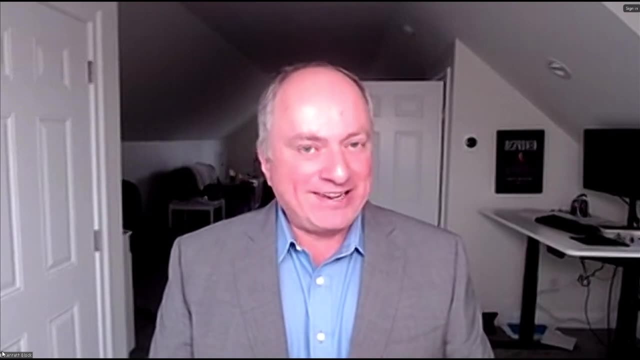 as hard as everybody else. I hired the male ballot king in Rhode Island to do whatever he does for elections- and I'm friends with him now- and I didn't win. But he did his thing and apparently delivered me a couple thousand votes. 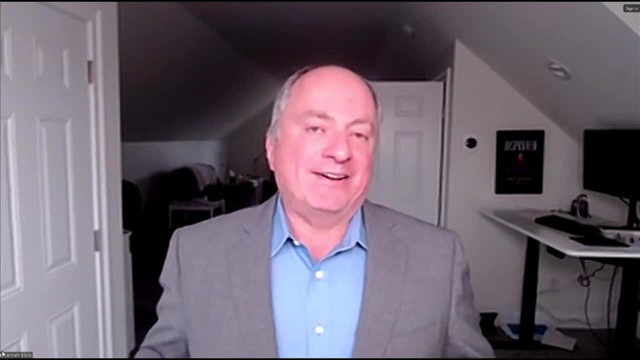 It's not this idea that you have third parties, or sometimes candidates themselves, visiting with voters as they fill out their mail ballots at their kitchen tables, helping them make their selection- There's no rule in many states that prevent that- And then delivering those ballots to election officials. 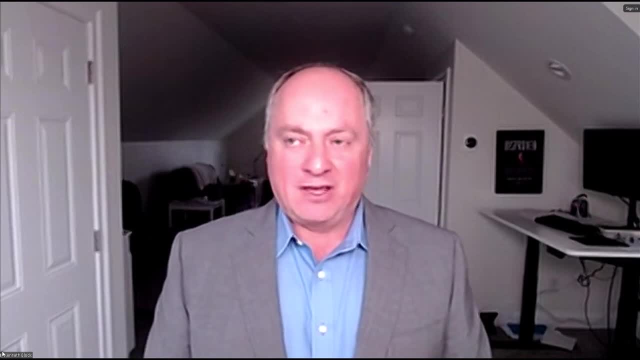 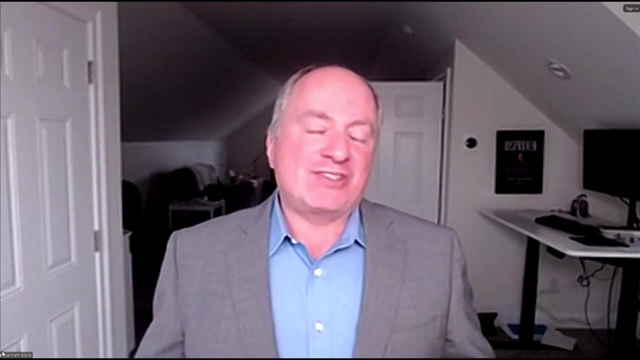 This collection and oversight of the voting thing is terrible. It's a terrible practice. The very thought that our elections could be determined by which side is more effective at collecting ballots is ridiculous. I mean, elections have always been much more about, and this kills me, right. 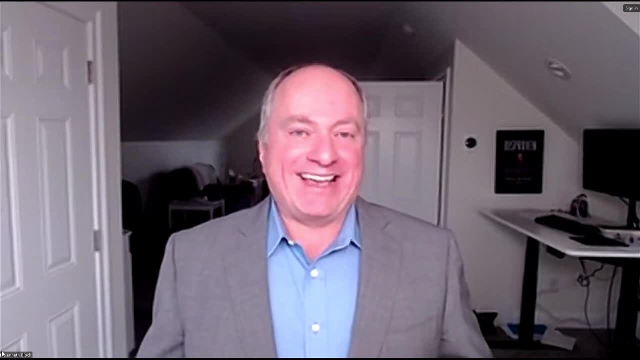 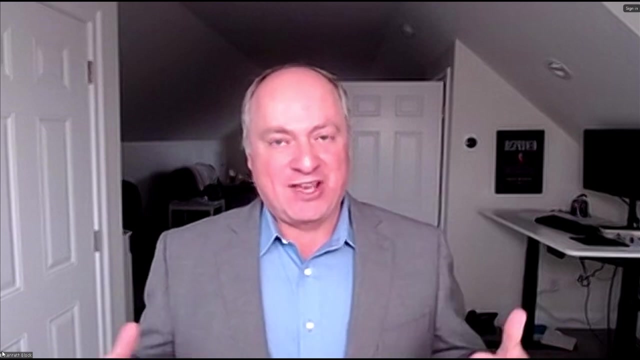 Much more about a beauty contest and about name recognition than about merit and about ideas, And ballot harvesting moves us much further away from the merit of the ballot harvesting. It moves us much more toward merit-based election outcomes and moves us much toward just this collection. 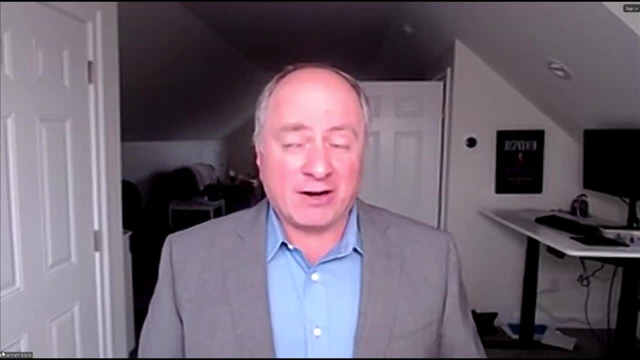 collection, collection, deliver, deliver, deliver. It should be outlawed everywhere. It's a terrible practice and as bad as gerrymandering, And I don't remember where Arizona is with gerrymandering. but if you guys do it, you should stop. 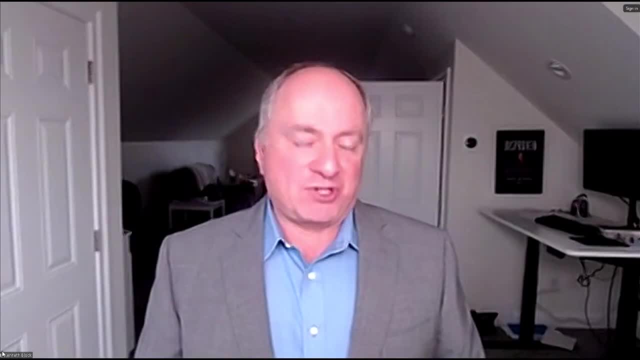 And what I say about most states: gerrymander and Democrats gerrymander just as hard as Republicans in states that Democrats control By and large. And the way I like to describe it is like this: Russia has a democracy. In that democracy, Vladimir Putin runs against. 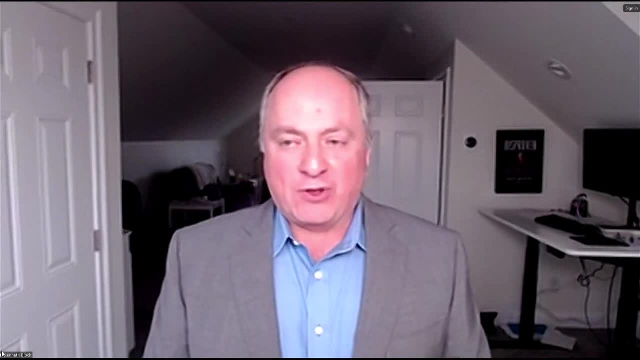 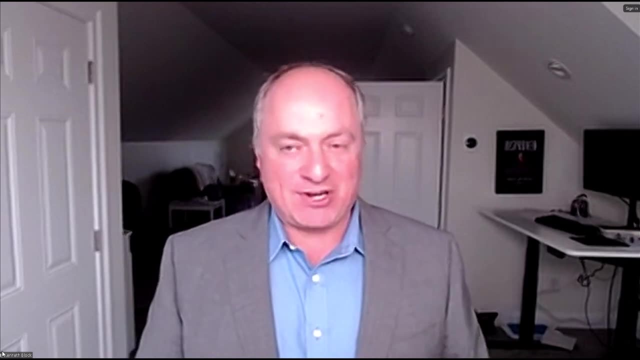 various assorted opponents over the years. For those opponents who get some headwinds behind him, he kills them, And that's how he handles political opposition. And when you have gerrymandering in the mix, what happens is elected partisan officials are drawing election maps. 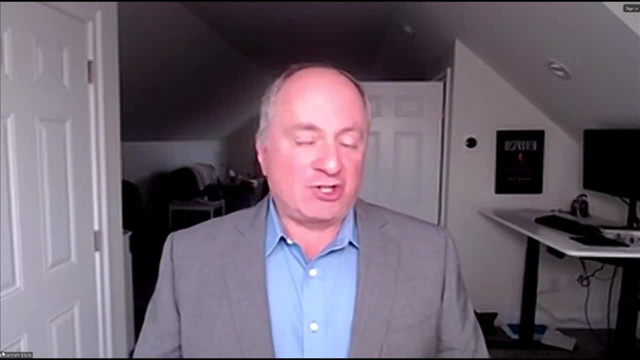 that favor their party. And what they're doing is they're murdering their opposition with maps. And what happens is it unbalances our elections. 80% of congressional seats are no longer competitive. We know with certainty which party is going to win those seats. And when you have non-competitive elections like that, you tend to get candidates who don't have to pay attention to voters, Except the voters at the extremes- And this happens for both Republicans and Democrats- And that's a bad outcome. We need the founders wanted our elected leaders. 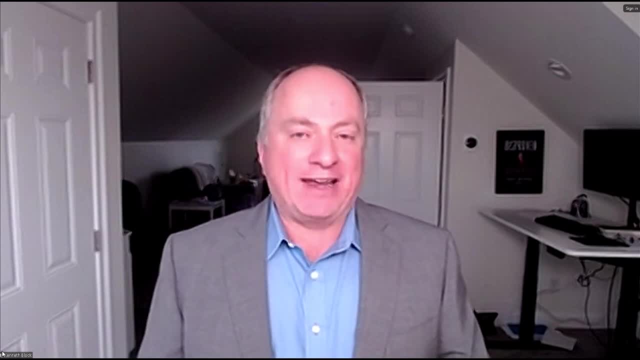 to forge compromises. Everything you look at in terms of how our form of government has been put together was to force and forge consensus and compromise, And we're moved about as far away from consensus and compromise as you can right now, And I think that is a direct result. 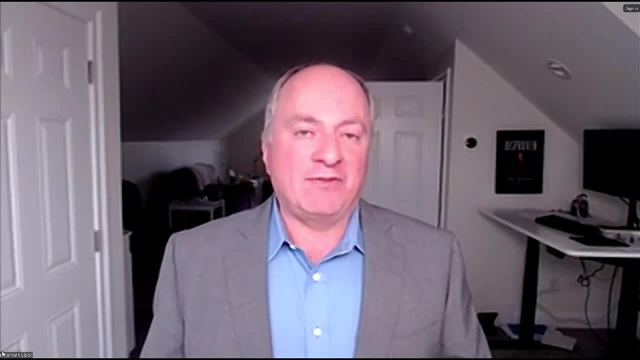 of our, of our un-competitive elections. For anybody who believes that competition is good in the marketplace, that competition helps us with innovation in the markets and that competition helps to keep down prices, how can you look at political competition and say that it's bad? 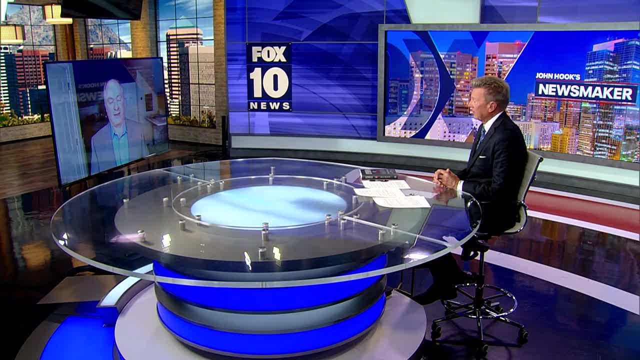 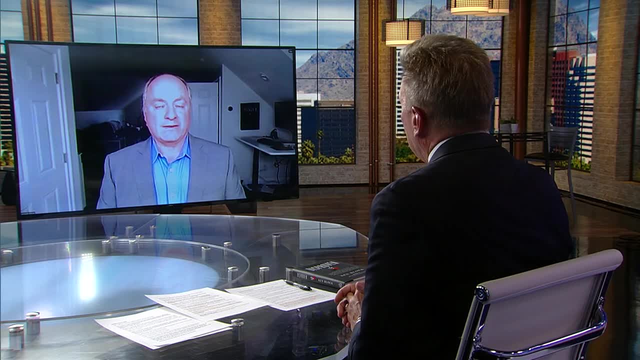 Okay, let me ask you about ranked choice voting. States are trying it, some are doing it. Arizona's tinkering around the edges on this as well- Good or bad idea? Terrible. There are academic studies that show clear as a bell. that voters get confused with the ballot design, And if you fill out the ballot wrong, your vote doesn't even count. The ballot mechanism itself can cause voters to become disenfranchised. It's a terrible idea, not only because of the complexity. 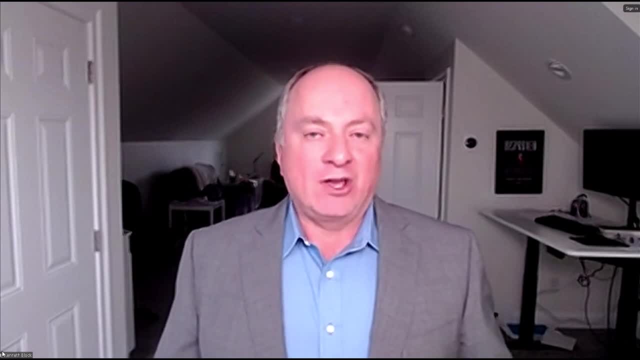 but the purpose of it is to try to deliver a winner who's got 50.1% or better of the vote. who has a mandate? It's a terrible idea, not only because of the complexity, but the purpose of it is to try to deliver a winner who's got 50.1% or better of the vote. who has a mandate? it's a terrible idea, not only because of the complexity, but the purpose of it is to try to deliver a winner who's got 50.1% or better of the vote, who has a mandate If you're winning your election in the third round of counting and ranked choice. 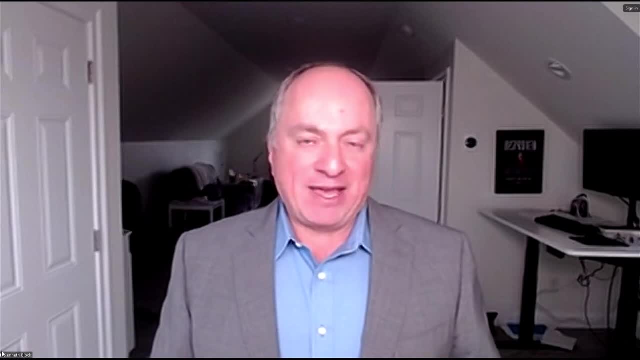 is a terrible compliment on United States. you don't have a mandate. you can't legislate or govern like you do Is a terrible compliment on United States. you can't legislate or govern like you do is a terrible compliment on United States. 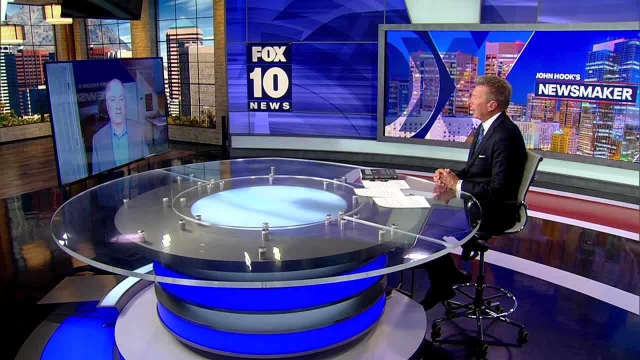 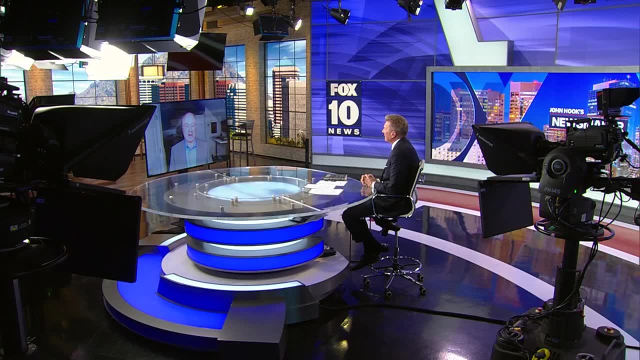 if you win in the third round. Chris Hall gear. Can you give us a quick example of how ranked choice voting works, because I'm getting in my ear that some people may not know what it is. Chris Hall gear, Because I'm getting in my ear that some people may not know what it is. 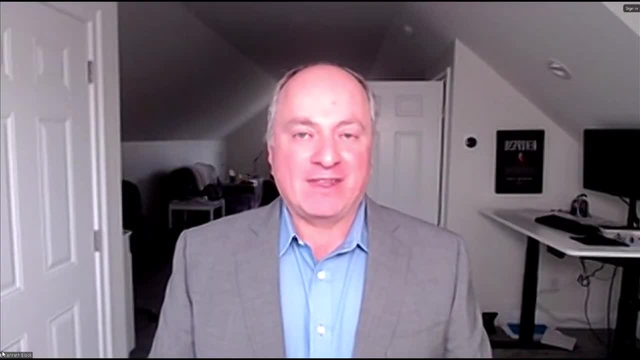 Chris Hall gear. So in a race where there's, say, four candidates, the voter is presented a ballot choice where they can pick their first choice candidate and their second choice, and their third choice and their fourth choice if they want to. And what happens is, when you count the ballots, if no candidate has 50 percent of the vote, you take the candidate with the least votes, remove those votes, look at those ballots and see what the second choice was and add those second choice votes to the candidates. count again, rinse repeat, rinse repeat. 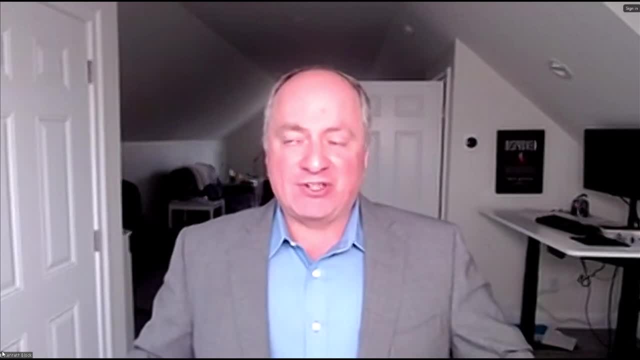 It's actually pretty complicated And I don't see that it's ever going to really catch fire. I've talked to some Democrat secretaries of state. You have told me that they just disagree with it altogether. It's not a good idea. 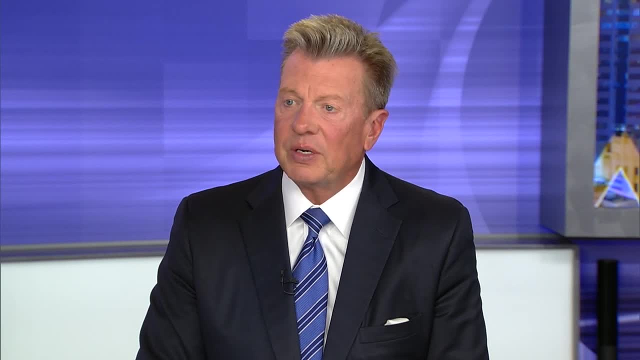 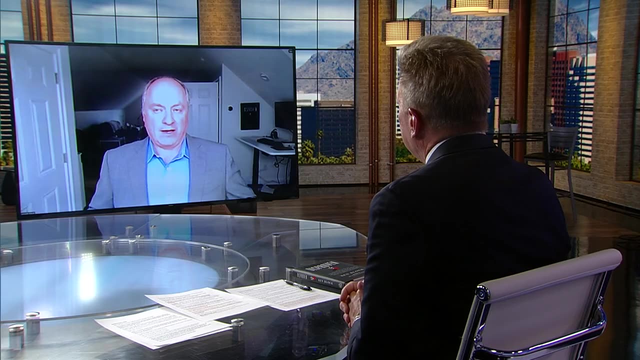 Yeah, I guess it would be a simple explanation. is it's kind of trying to weed out who's the least objectionable of the four you mentioned? That's what you end up with, Possibly. I mean, who knows, Who knows how the counting ends up going. 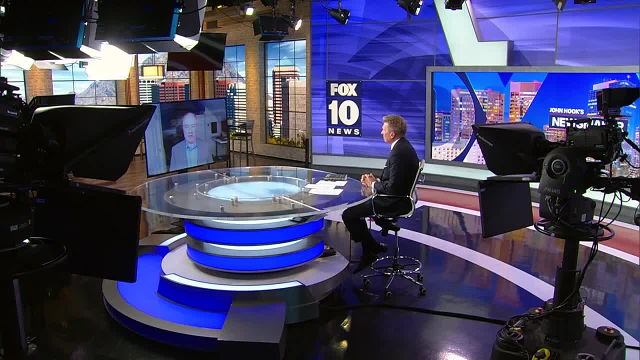 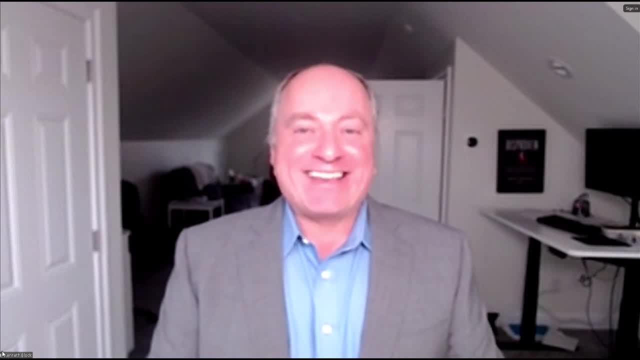 But it's very unlikely, especially with the ideological divide we have right now, that anybody would mark more than one or two choices anyway. Oh, I see, Yes, right, You're not going to see conservatives ranking a liberal number three, for example. 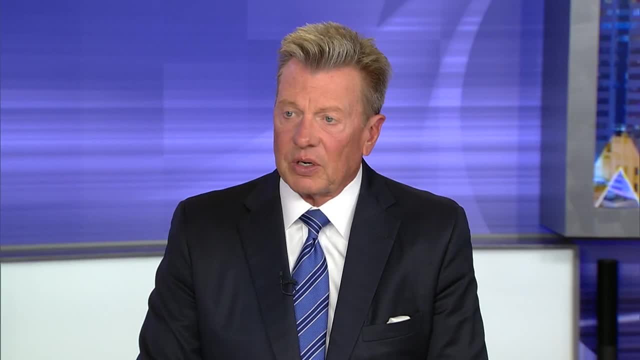 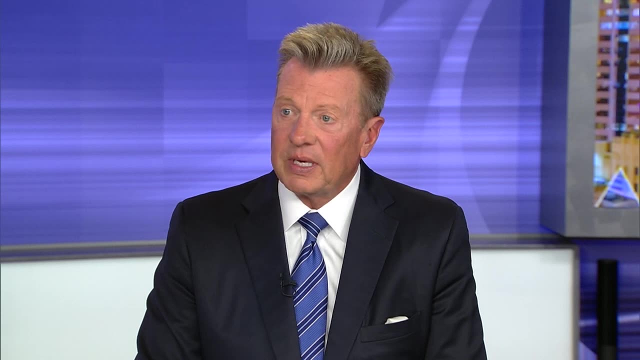 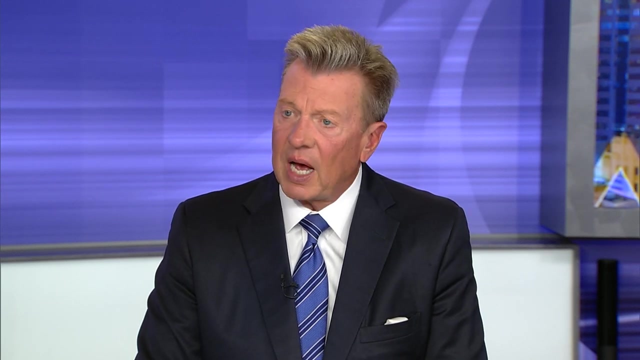 Yeah, Finally, Ken, since you've been diving into this for years, if you were running elections- and it was a national election, seriously not broken up into county by county all over the country, what are the few changes that you think would really make this thing? I don't want to say bulletproof, because nothing is but where everybody could be confident this is a solid election. 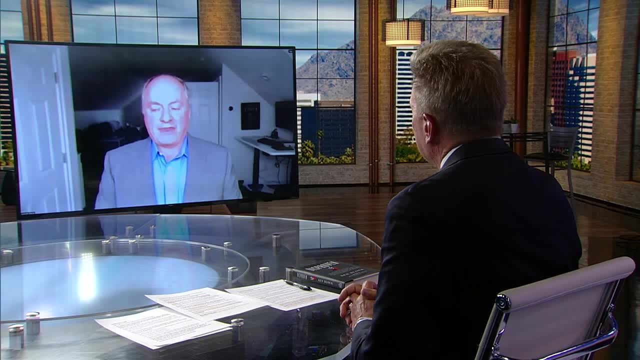 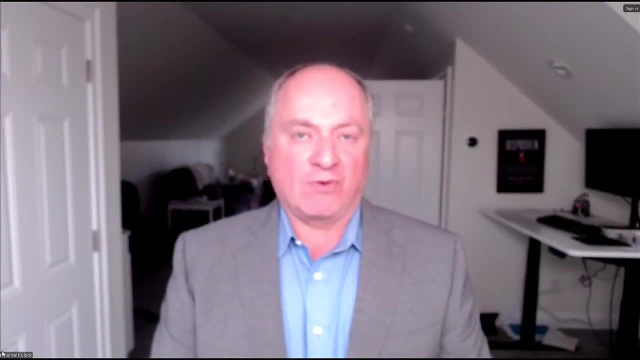 We've got this buttoned up. Yeah, I think the federal voter registry is mandatory In the absence of a single voter registration system. what we need is a computer system that every single state is compelled to participate in, whose purpose is to look for duplicate registered voters, look for deceased voters and remove them from the rolls. 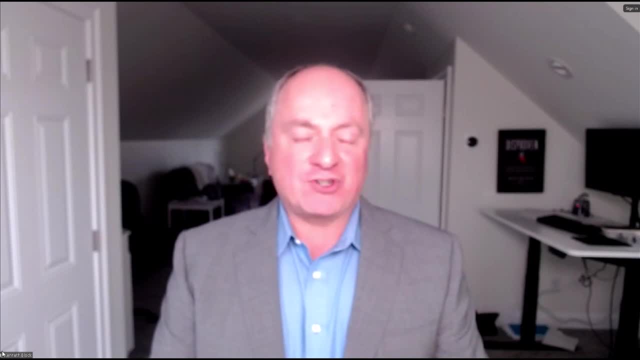 It should be a governmental function. It shouldn't be a non-governmental. It should be a non-profit function, like the Eric Consortium of States, which a lot of states used to take part of- more than 30. Now it's become fairly partisan and just some Democrat states use it now.